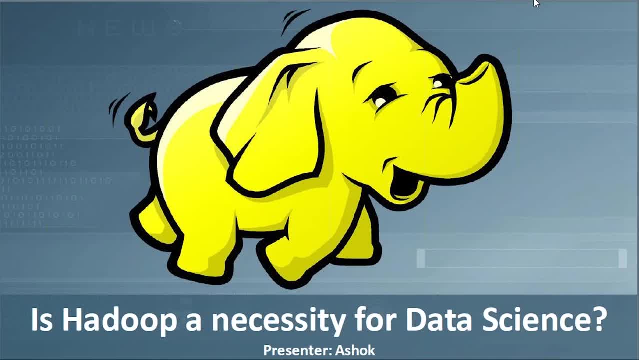 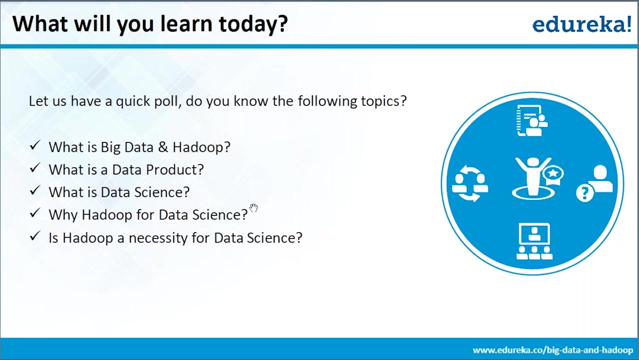 Thanks for coming again. Yeah, So today's topic, as you can see it's quite interesting: Hadoop and necessity for data science, right? So let's get started. So just a minute. So what will you learn today If you look at it? Let's have a quick poll. Do you know the following? Like what is big data, Hadoop? 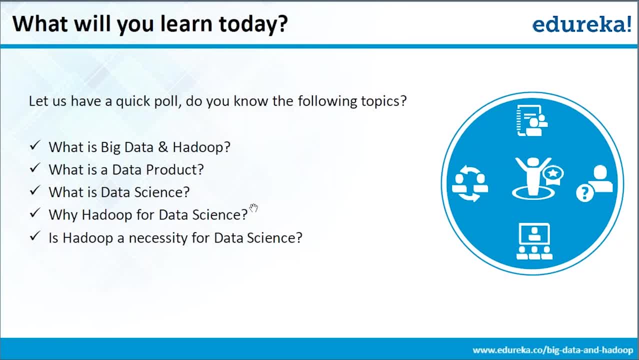 What is a data product? What is data science? Why Hadoop for data science is Hadoop and necessity for data science. So these are all the things we are going to see that in a nutshell today. So I'll try to cover, cover how much ever possible, friends. So I have like 20 odd slides And that also includes a demo towards the end, Right. So Mohit, Okay voice. So friends are you? 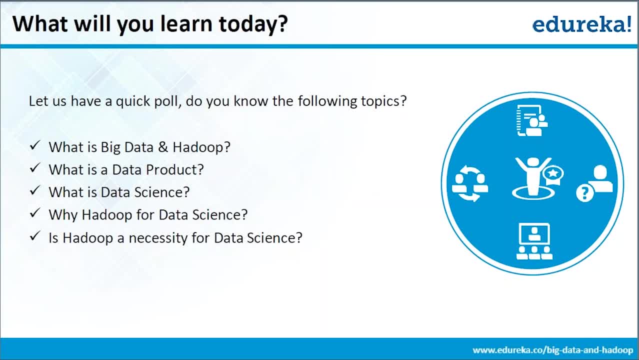 anybody having audio issues. Thanks for the confirmation, friends. Oh yeah, everybody seems to be perfect. Even Mohit also just clarified to me. So he's just doing a check at his side, All right, fine, Not able to hear anything, So I'll coast up, All right, Others can hear me, Right. So, friends, what we will do, you know what we will do- is: 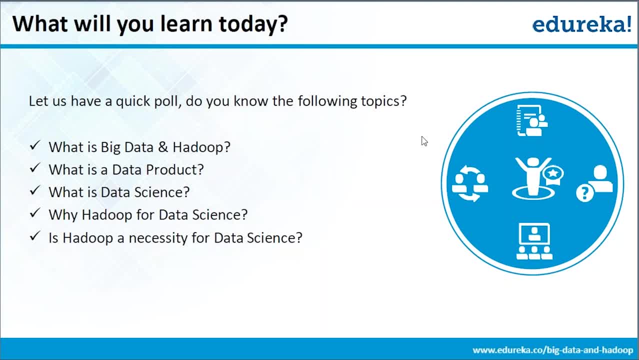 we will the structure of this today's presentation right. The way I want to keep it is: let's go over the deck, because I know everybody's inquisitive and I'm sure everybody has got questions, Correct. So, but just, you know, in the interest of time and you know, and also in the interest of the audience, you know, I don't want to disrupt the flow of the session, Correct, I don't want to disrupt the flow of the session. So what I will do, I will take you through the session. 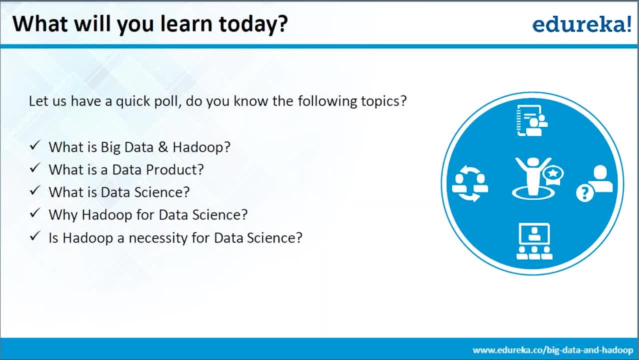 Please allow me to do that, Right, And? and you can always bring up questions. you know when, when we have questions that you know towards the end. So what I will do, you know, before I go to the demo, I'll pause for question Q&A for some time. Then, after the demo, you know we'll have Q&A as well, Correct, And you know I'll try my best to wrap it up in one hour. Correct, That's the agenda. So so what is? 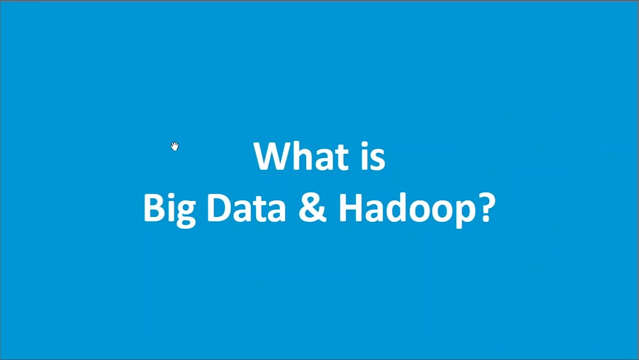 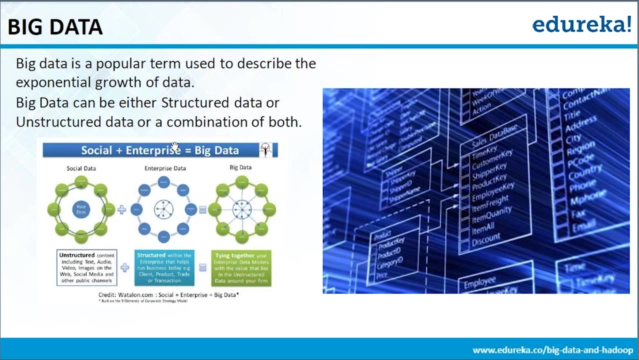 what is big data? and Hadoop Correct. So this is the first thing we are going to see. Big data is a popular term used to describe the exponential growth. of data can be structured or unstructured, or a combination of both. Right? So what we are saying is it: can you know if you look at the today's stats? right, this is a no brainer. You know, the data is coming from various sources today. 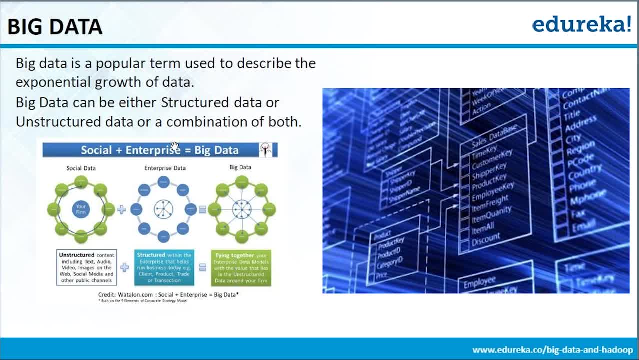 Right, We have varieties of sources, whether it is an application server or you know a web server, or from all these devices like Fitbit and you know any kind of IOT devices or any kind of you know network devices, Correct, And all the social media sites. So everything is you know it, it the data is coming out of that, Correct, And 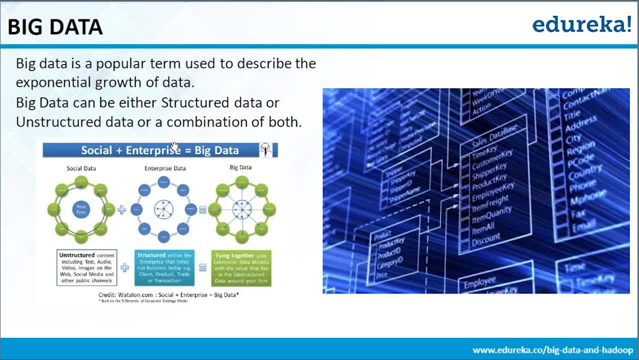 these are the things which we cannot. we can no longer ignore these things, Right, Because in the, in the past, it was just one database and you know very structured way of collecting the data. Now, the data collection, or you know it, starts from the instrumentation all the way up till, you know, visualization. So when, when the data collection happens, Right? So we want the data to to live, to live forever. 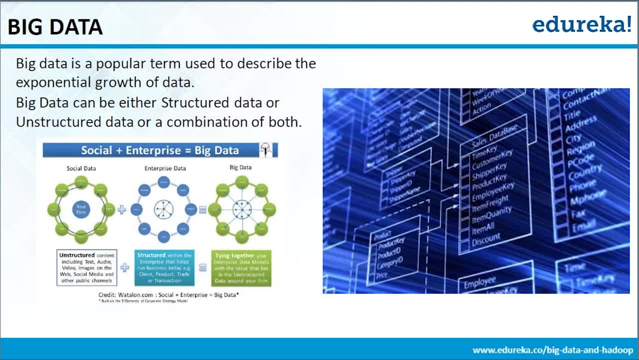 Right, Because we have realized the value of the data, We have realized the potential of the data. We don't want to shell the data or archive the data. Correct, Because we want the data to be available for analytics all the time. Correct, So we have, you know, thought through various architectures that can actually hold the data forever, Right? So if you look at the stats again, it is predominantly 80 to 90 percent of the data in the world today is unstructured. 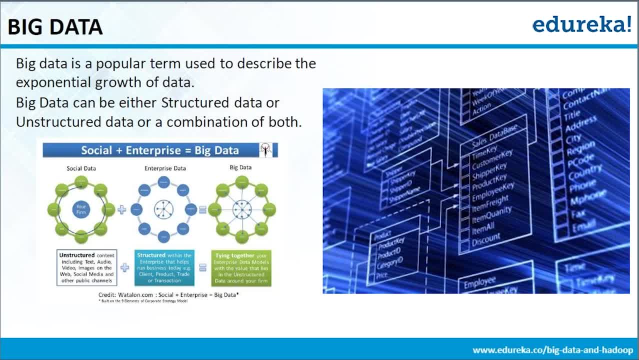 And the data is exponentially growing, as as mentioned in this slide, Right, And if you look at the velocity of the data, which is the growth you know at which the data is growing, Right, The space at which the data is growing, It is phenomenal. It is just a simple example. You know New York Stock Exchange. They are saying they are generating like one terabyte of new trade data every day. Correct, One terabyte of data. 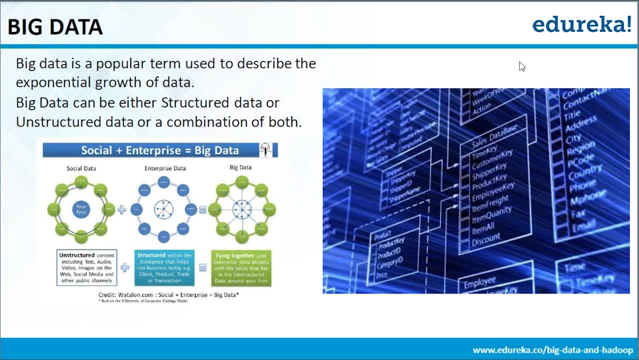 Right, Which is nothing You know. if I tell you a few other things, these things get dwarfed by that, Right? The Hadron Collider, Correct, It's one of the largest particle colliders. They are doing a, you know, big experiment in Switzerland, Right? So those? that collider generates about about a petabyte of data every 3.5 seconds. Correct, Phenomenal amount of data. Phenomenal amount of data. 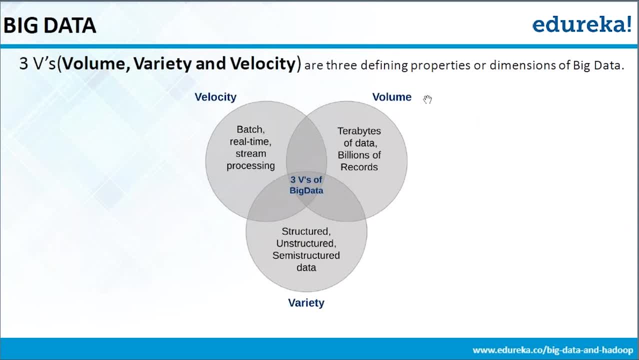 This is a very famous definition. You all would have seen the dimensions of big data represented in three ways: Right. One is the velocity, real time. Right, The rate that the pace at which the data is growing. and volume. It's like in all the social media. If you look at Facebook, if you look at Twitter, you look at Tumblr, Instagram, all these sites are growing like crazy. Right, And you are talking about, you know they are processing millions of queries and you know, and Twitter is like a 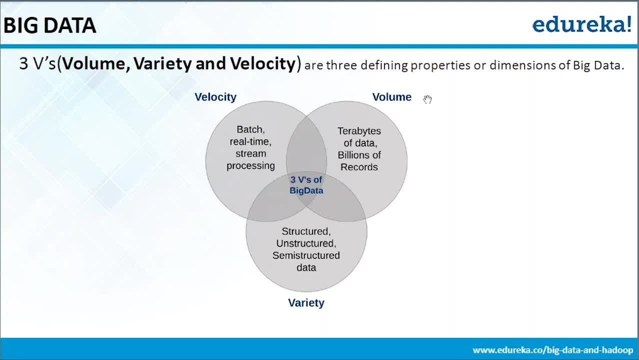 Having 500 million tweets per second- Sorry, per day, Correct, It's 500 million- is staggering, Right? So that's the kind of- and we have about, you know, 500 million CDRs We are processing, called data records, Right? So everything is like the volume is staggering, Correct, The volume is staggering, Okay, All right. So and the variety? we talked about it. Right, We talked about the variety. We said data. 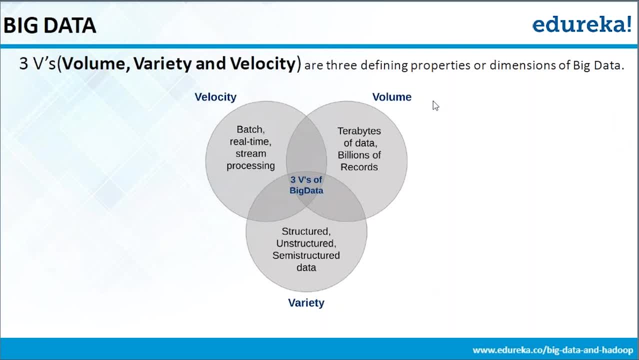 And from what sources. from what sources we are getting, and we are getting structured, unstructured and semi-structured. We have lots and lots of varieties. We are also getting this data Correct. Variety is also playing one of the And one of the fourth dimensions which we haven't mentioned here, which is there in your IBM is just which is your. Can you all guess it, friends? What is the fourth dimension in the four V's? 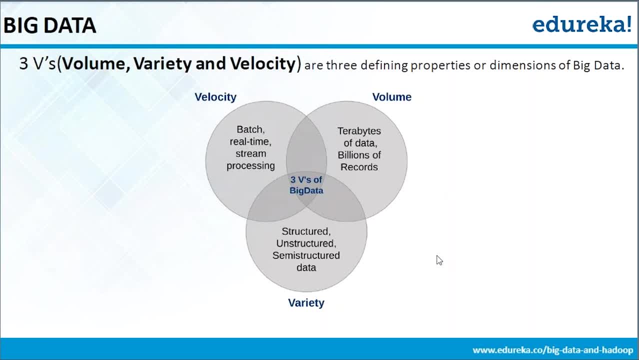 Veracity. Okay, Can someone tell me what is veracity? What is veracity, friends? It's a very interesting one. Truthfulness, Fantastic Truthfulness, Right, Fact based information. Can you give me an example? It's a lovely thing, I mean. what I feel, personally feel, is no. it has to be accorded the same amount of respect. What we are called, what we give for velocity, volume or 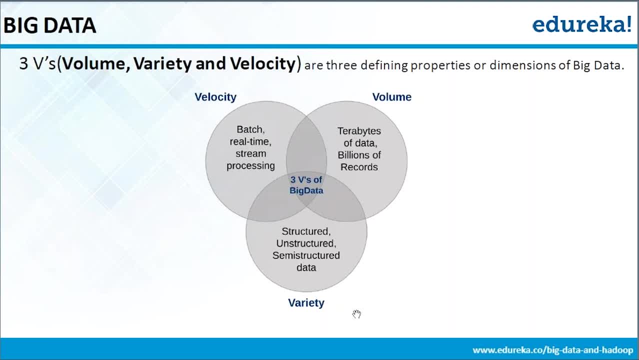 Variety Right Because truthfulness, if some field got missed in the database, it should still process the data. Is that what it is, Abhishek? Truthfulness or the you know, the validity of the data itself. Right Validation, Correct Right, The validity of the data, or if there is any certain uncertainty in the data, Can you give some kind of? Can you give me an example which happened quite recently, Quite recently? Can you give me that example? 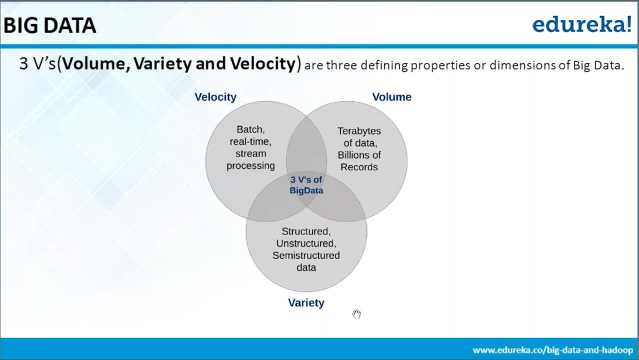 That happened in the automobile Mobile industry. I just give you all the clue. in the world, Volkswagen, Fantastic, Yeah, I think you're all. emission scandal, Right, Correct? Fantastic friends. Volkswagen emission scandal. So they just fudged a small device, Right? This fudged a small device so that it will. you know whatever the emission of nitric oxide? it goes undetected in the emission test. You know whatever that is done in the research labs there, Right? So they just fudged that. 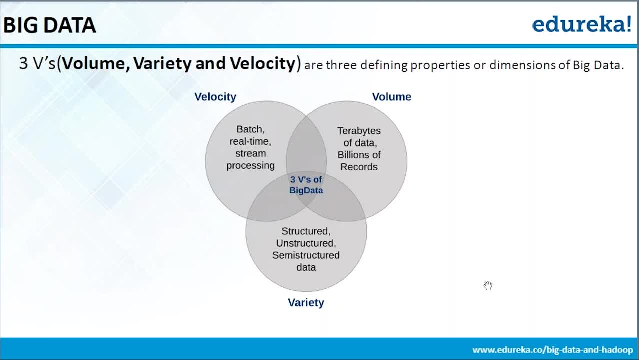 Like a Student Technology Theory Competition or some anything like that. actually, one of the interesting things in this too is, you know, first of all, this person will be honestly flashed, even if given some kind of Due Mass Effective- puisqu- the کہ friends- when another random data source or something happened. and then people are, although it came up with a kinda beter color choice, and you know, keep him up with these flying colors. and the same guys, you know they tested BMW upside down. you know they found Wo to be extremely successful and 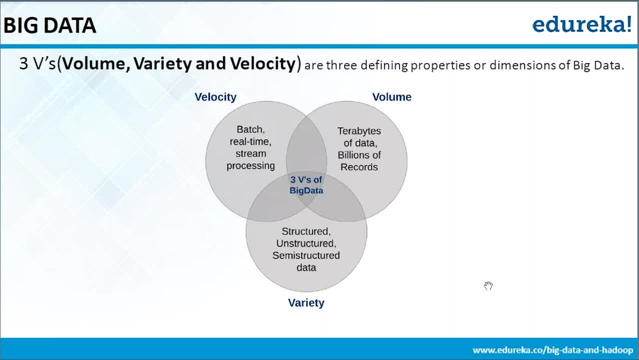 and they also certified Volkswagen, especially the Passat model, and see what has happened. right, it is the case of veracity. right, the truthfulness, the if there is any ambiguous data coming in, right, the whole thing. friends, what I'm saying is, if the data is uncertain, if the data is ambiguous, 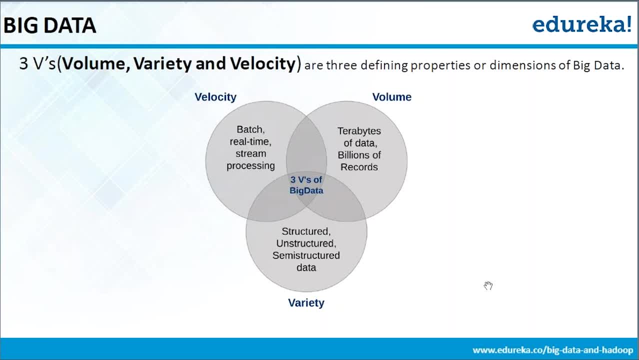 whatever coming out of the data, it may still make sense to you because- and you may be- you may make you know, you may derive some insights and based on the insights, you will come up with a product decision, or you may come up with a major business decision itself. so that may prove to be completely. 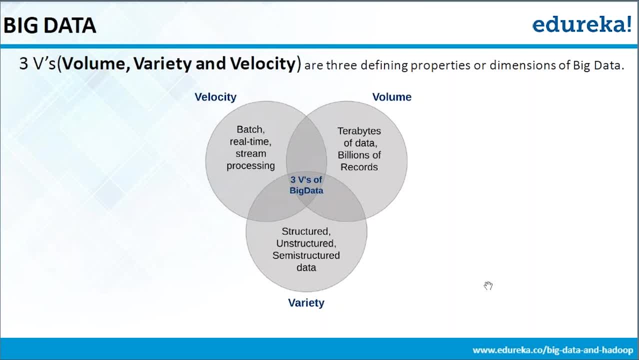 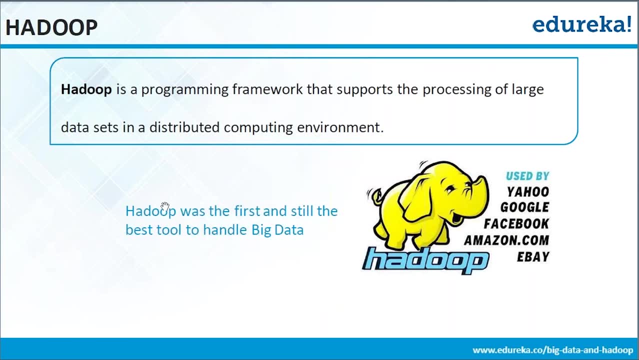 wrong if the data itself has got some issues right. so that's the classic case, thanks, thanks for explaining, friends. I think you're all right up there in understanding this veracity part. yeah, so Hadoop is a programming framework that supports the processing of large data sets in a distributed computing environment. first and still the best tool to handle big data. 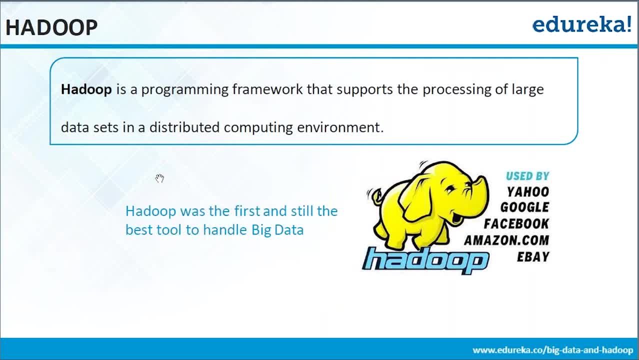 I think there are lots and lots of tools today, right today, people are talking about spark, people are talking about storm, people are talking about sparks, sparks, streaming, people are talking about flink. I think you'll have lots and lots of derivatives and you lots and lots of flavors. 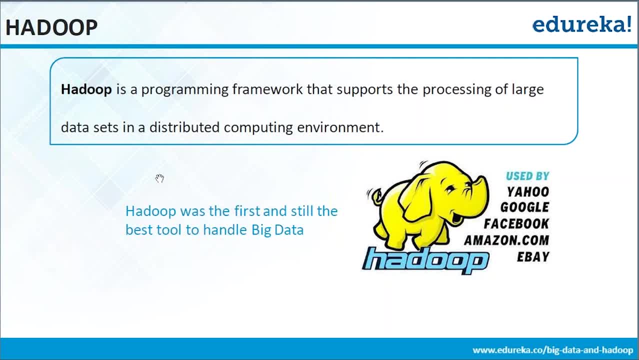 coming out and out of Apache, Hadoop still continues to be one of the most powerful ones, and a Hadoop's. you know the investment is close. you know it will get closer to $2 billion by 2020, and it's growing at a staggering rate. 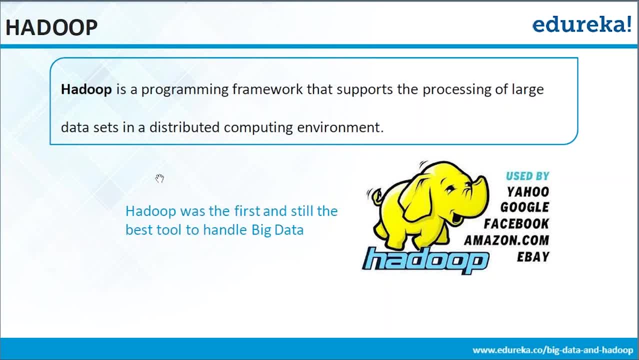 of 58% year over year. right, So there's no way Hadoop is going down. you know There are a lot of misconceptions. People say that you know Spark is going to overtake. It's not like that, because Spark is in-memory computing. 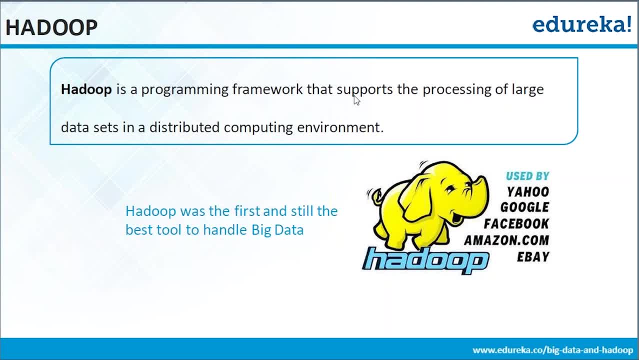 and you know Hadoop is for a different purpose, correct? So I mean Hadoop can handle elephants. That's one of the reasons why they put the elephant here, right, so it can just take any amount of data, right? 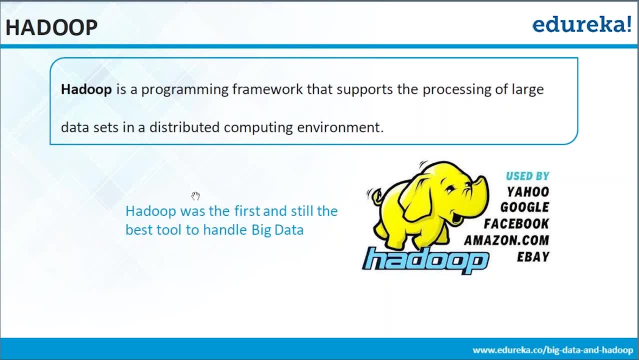 And what is the difference, friends, between Hadoop and your traditional RDBMS? can someone tell me Quickly any fundamental NoSQL database? okay, all right, can handle unstructured data? fantastic, Yeah, that's the kind of difference I want, friends. 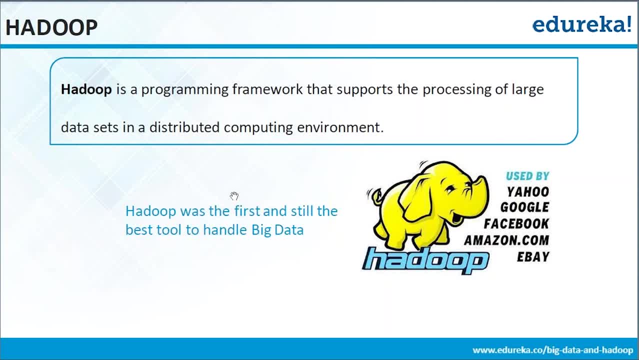 the framework, Yes, and distributed file system: excellent, correct. Unstructured data. distributed file system: okay, That is OLTP. this is OLAP, correct? Find schema on read. schema on write. I think a lot of I think you guys are rocking here, correct? 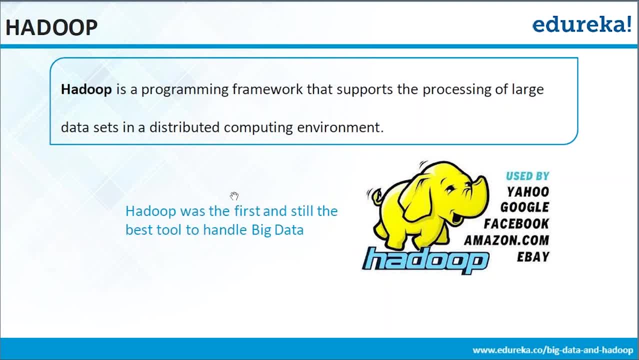 Works in different code, moves to the data. Brilliant Anshul. yeah, Lots and lots of great points are coming in. I mean, what I other thing I wanted to talk about was the architecture piece, right with Hadoop. 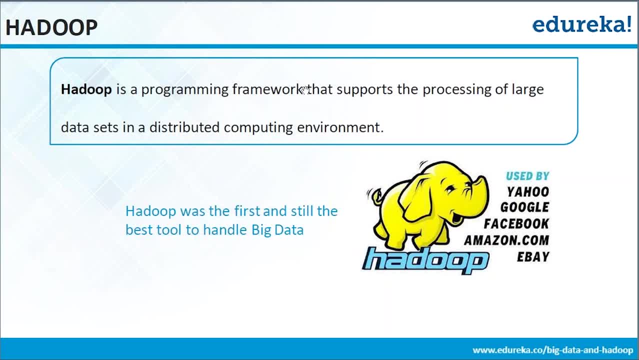 I think you guys are gonna like it. right. It is more a scale-out architecture, not a scale-in architecture, a scale-up architecture. right, It is scale-out, scale-out architecture. meaning if we need to go right- I mean if I am expanding- 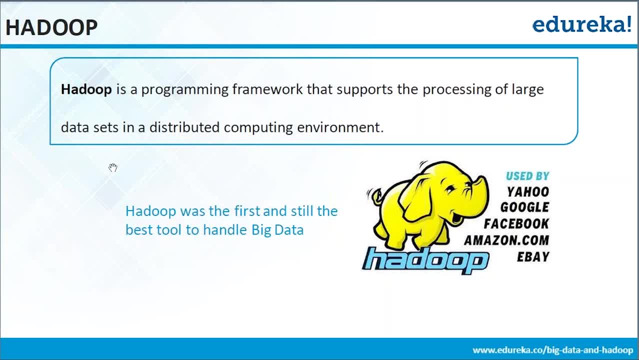 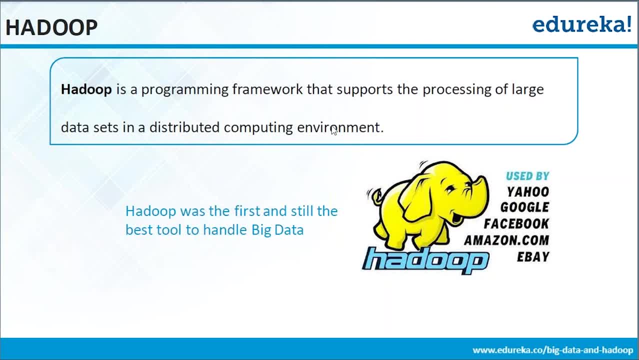 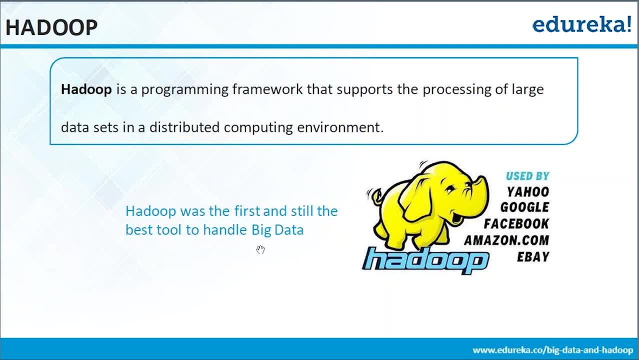 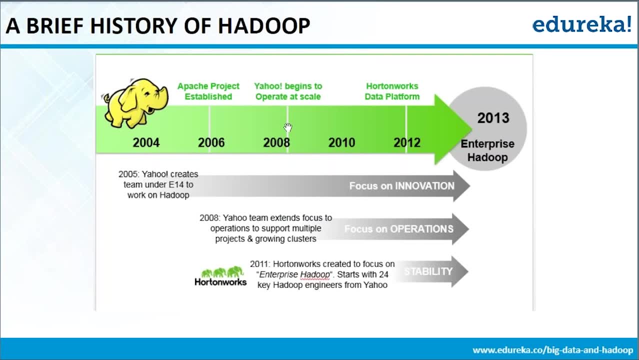 That's one of the significant differences, correct? Hadoop was the first, still the best, okay, sure? Brief history of Hadoop 2004.. Yahoo creates 2005 under E14 to work on Hadoop. Apache project established. Yahoo begins to operate. 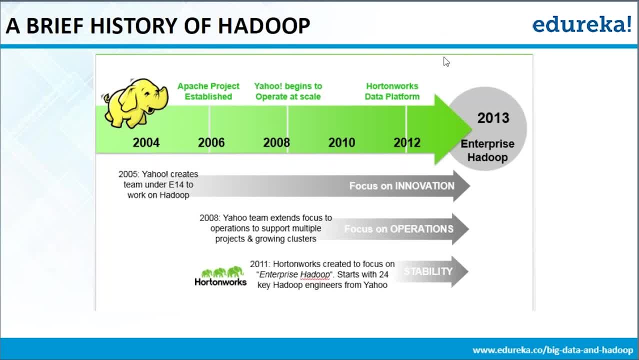 at scale. Hortonworks data platform. Okay, focus on innovation. Actually, when Yahoo, when Yahoo started it- and you know later it was- it became a full-fledged, you know, Apache. it was became a full-fledged Apache platform. 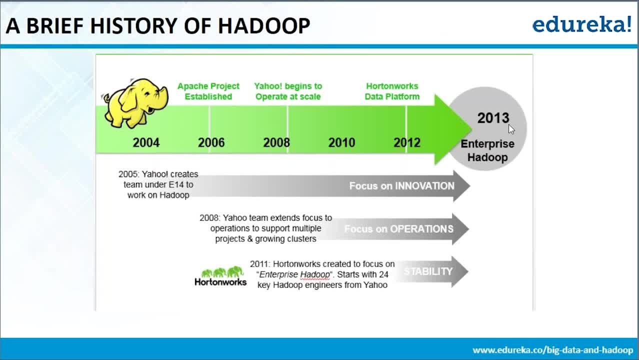 It was incubated and, you know, became a formal launch, correct? And I think, as we speak, I think we are running 2.72,. I think we are running 2.72, if I'm right, because every day you know. 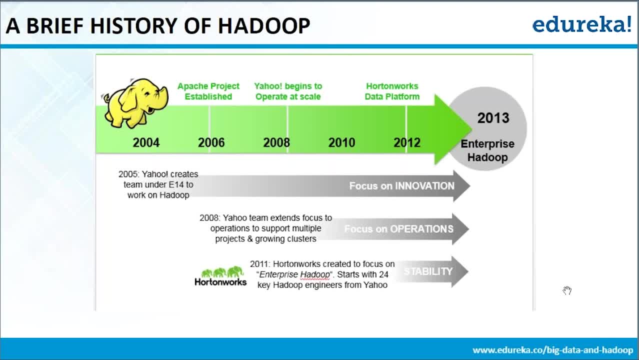 things are evolving right. Things are moving pretty fast, So it's. it used to be 2.72, then I saw 2.72, one of those formal releases. I don't know what it is today, but it should be around that 2.6 plus right. 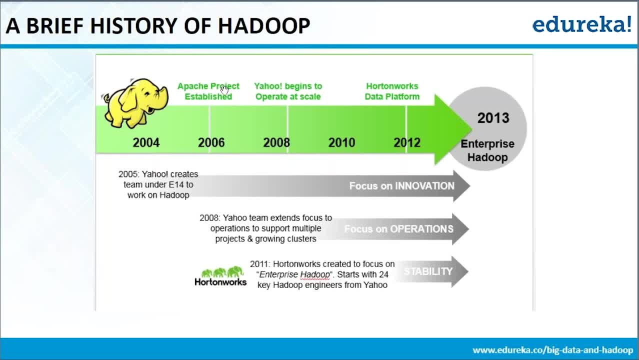 2.6, 2.7 types correct. So it provides. you know Hadoop provides a lot of fantastic features. you know it provides economy on scale and it provides liability through fault tolerance and it provides flexibility. 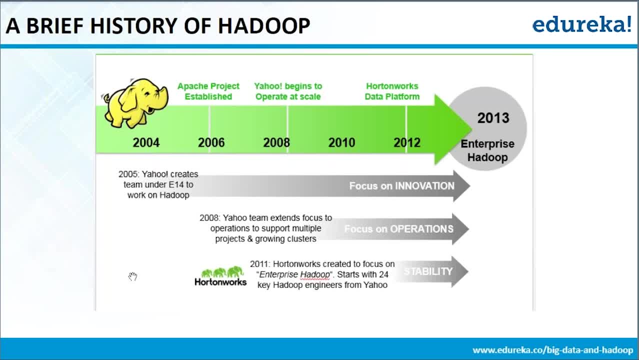 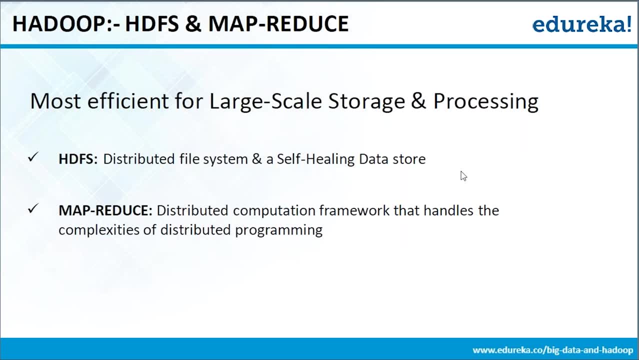 and these are some of the standard features of Hadoop: correct. Most efficient for large-scale storage and processing. Correct Distributed file system and self-healing data store. Correct And MapReduce distributed computation framework that handles the complexities of distributed programming. 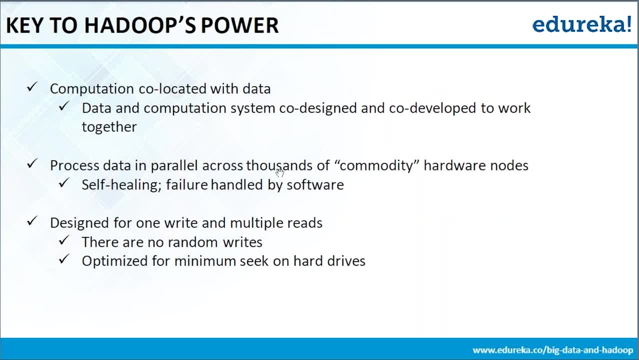 Correct. So we have this computation co-located with data. so that makes it special, as many of you pointed out, Data and computation system co-designed and co-developed to work together. you all would have seen the name node and the resource manager. you know, name node is the master daemon for storage and resource manager is 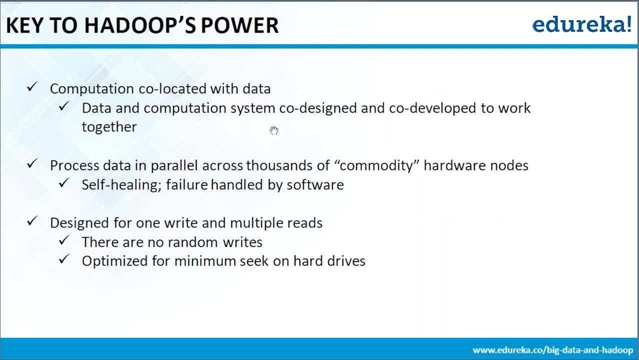 the same thing for processing. they actually sit in the same server in the distributor cluster, correct, and similarly on a slave nodes and all that you have, you know. similarly, you have data node and you know node manager is for the processing slave daemons. right, they do that. 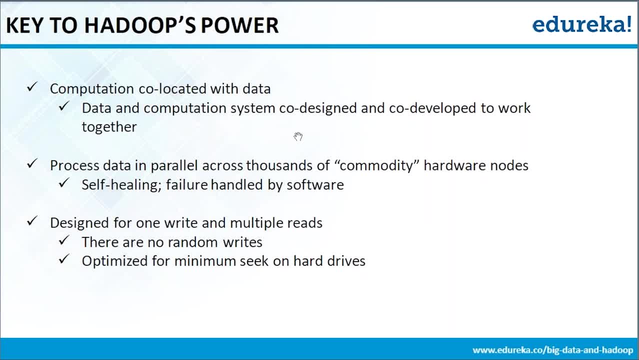 So it is one of the frameworks. you know where they have conquered this. you know where. in a traditional system, what we do? we move the data to where the program is running. that actually cripples the network bandwidth and it can crash the system as well. that's why we were doing the 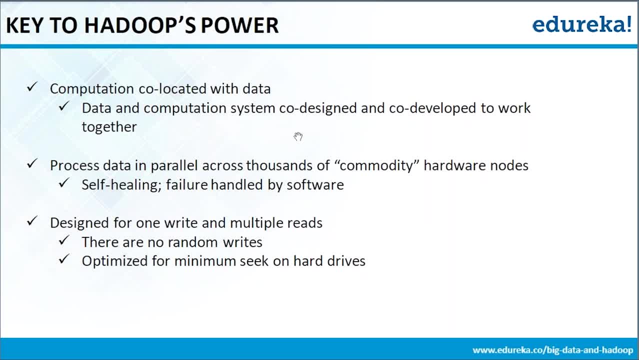 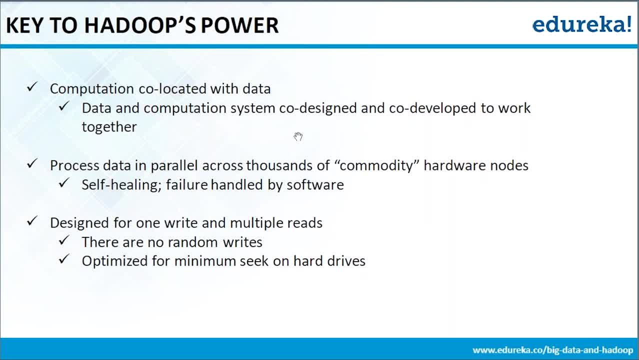 a proper architecture in place to handle a high volume data, correct. so now, with the advent of Hadoop coming in, now we know how we can do this. so because the data and computation have become together right. so the compute layer, the date, the, the, the program itself, is taken to the place where 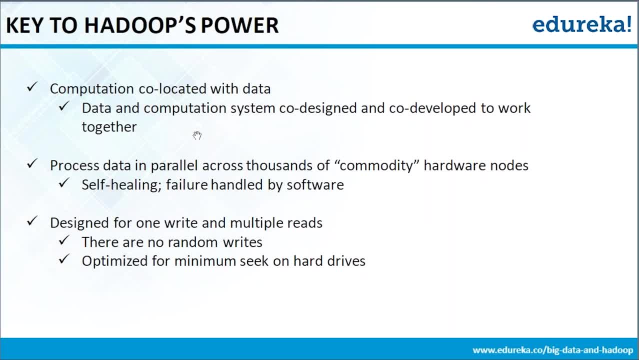 the data is located. so this feature is called data locality. right, it's a very, one of the most significant standout feature in Hadoop. data locality really, you know, makes it very powerful. right, the data is never moved. the program is moved right, process data in parallel. the other thing is the data is stored as blocks, right, as chunks, in various 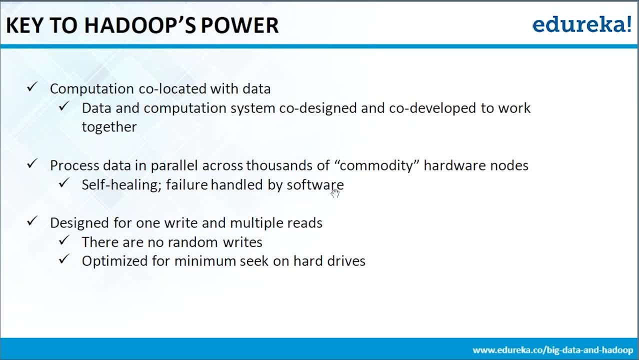 commodity servers that may. that also makes it very special in Hadoop, right, so we are able to do things in parallel. commodity hardware nodes, self-healing failure handled by software itself- correct, then designed for one write and multiple writes reads- correct. there are no random writes. optimized for minimum seek on hard drives- correct, and Hadoop provides high throughput. 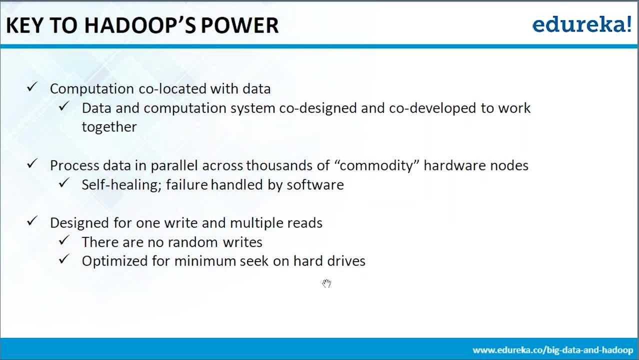 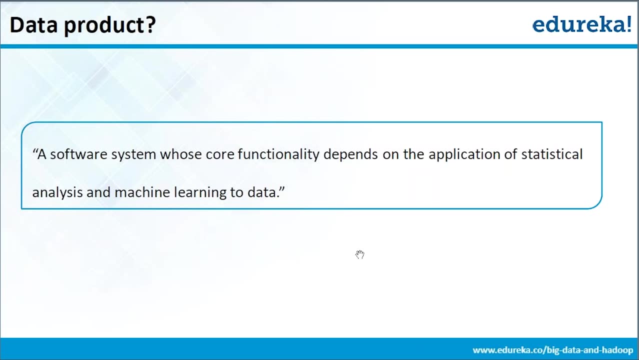 and high latency as well, because you know, I think it is. I think some of you pointed out that you know, RDBMS is more OLTP, this is more OLAP, it is by design correct, friends. okay, what is a data product? a software system whose core functionality depends on the application of 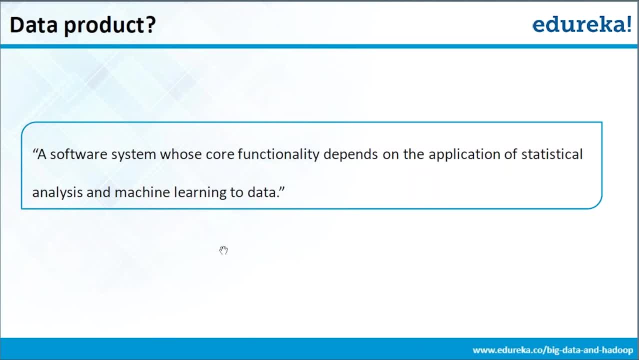 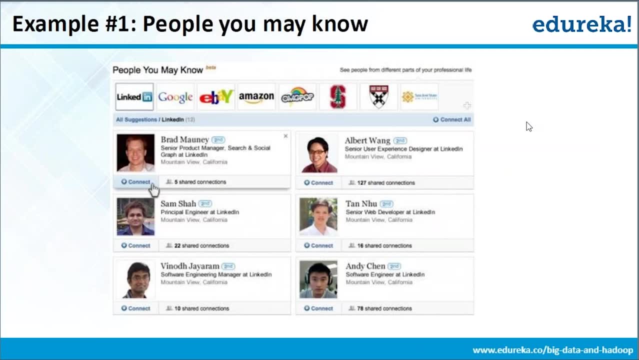 statistical analysis and machine learning to data correct. so, if you look at it, okay, I I want to ask you this: people you may know, where do you see these friends? where do you see this feature? people you may know. okay, bingo, all of you are saying LinkedIn, correct, Facebook. okay, Facebook also. yeah. 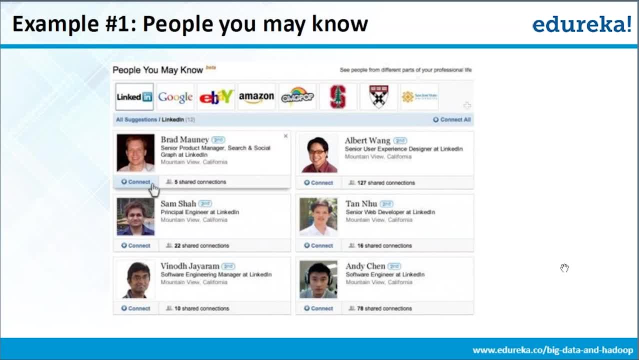 okay, sure, so how do you think they are providing this feature? Facebook, LinkedIn, okay, how do you think they are able to come up? and friends, do you all agree with me, the people you may know? it may not be, so. you know, most of the times at least. 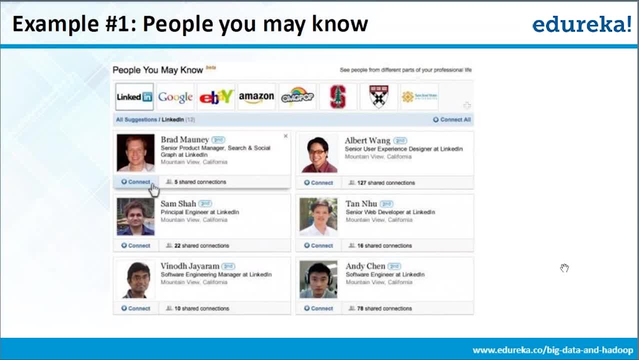 in my case, right, it is 40 to 50 percent of the times. I find that link to be meaningful and I go and connect with the people correct most of the times. so I mean I would say 50 percent of the times correct. so that's, that's fairly a good hit rate, right? how do you think they are doing this? 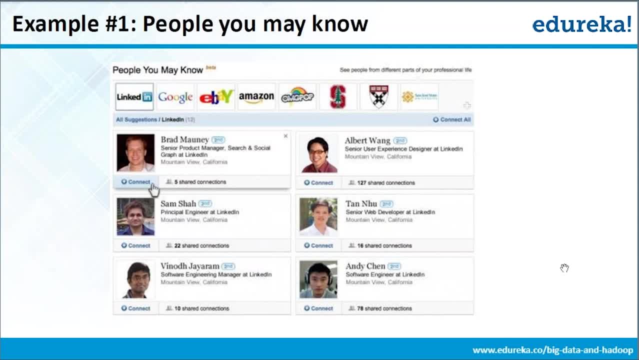 any guesses: machine learning, excellent, correct. machine learning says Bouchon, correct. so they should do some kind of. you know, they are definitely running a machine learning algorithm, for sure, correct. machine learning, correct, and and they are doing it, for I mean, they, they do it, they do. 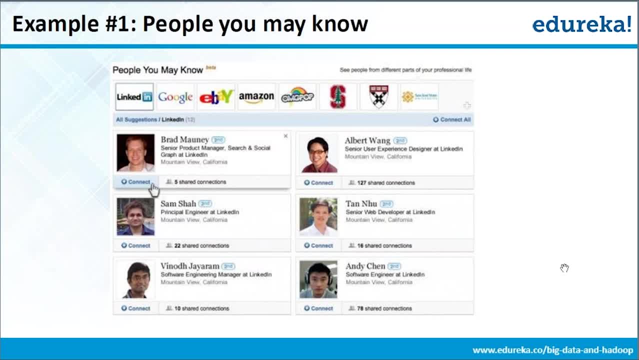 things like you know. for example, you might have heard about a tool called Mahout- right, it's a ecosystem tool of Hadoop, correct, so that one does recommendation engine. right, there are so many recommendation engines and you know they also look at your click stream pattern and click stream. 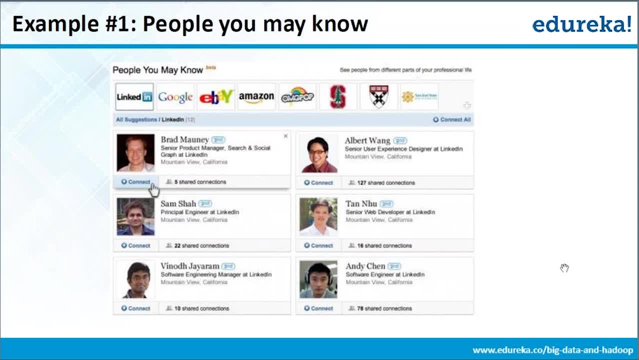 analysis and you know, come up with all these things. definitely, machine learn learning plays a part in this, correct? so they do all these things. come up with recommendation, even Google ads. right, you would have seen Amazon book books. if you are reading this book, it's goes and suggests: okay, go on, okay. people also bought this. 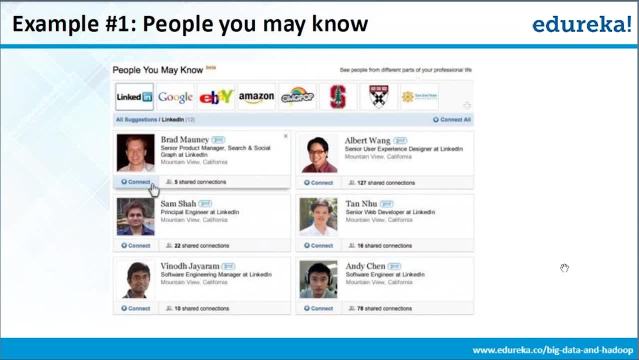 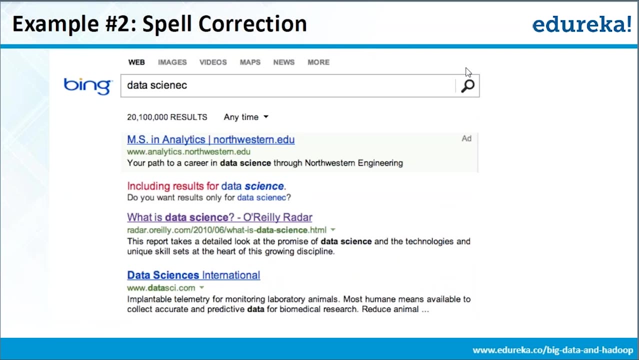 book. it says that right people who bought this, they also bought this book, so that also gives a lot of relevance, sure, so they use that algorithm correct. so look at this. including results for data science. see again. look at this. this also where. how do you think they are suggesting this? 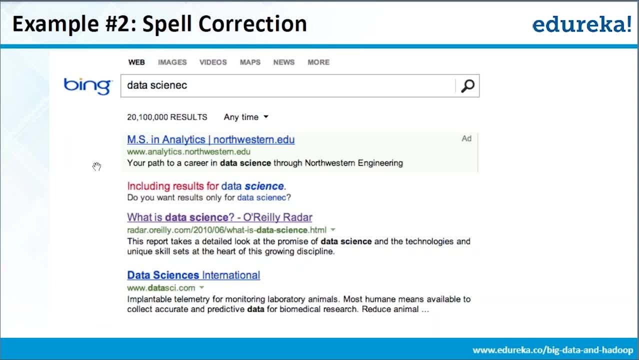 okay, regular expression, Taniru, anybody else? friends, past clicks, keywords, mapping- yeah, there are so many things right, frequent, correct, correct based on popular search criterias, pattern matching, prediction- that's a same machine learning- yeah, machine learning is also there. pattern matching is also there. text mining- fantastic. yeah, they do all these things. if somebody who's doing this right. 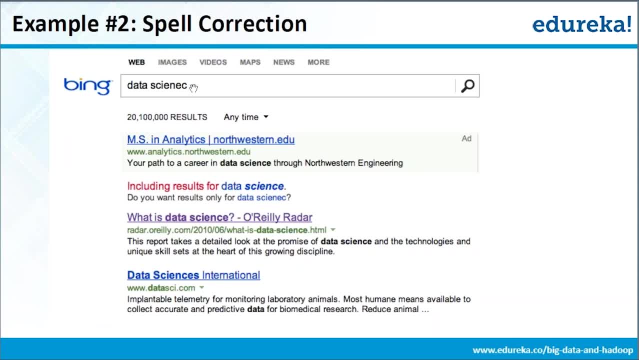 it pretty well knows that. you know you're probably it's just a typo here and it already doesn't auto suggest correct with pattern matching, with data mining. fantastic, Samira, right. so when they do this, right, they also list down the data science things below. they don't waste time by giving 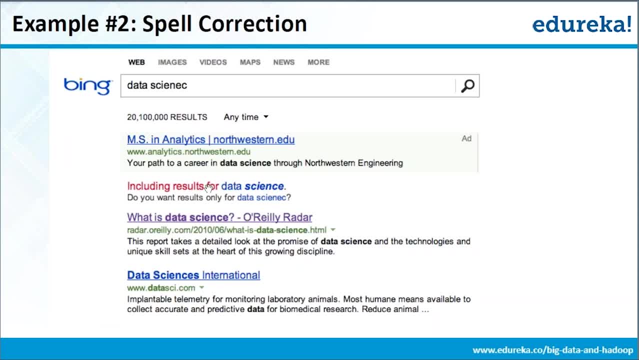 you a? did you mean data science? yes, but they already say this is what we are trying to do, but do you want results one day for this? they are still asking this. so they are. they are already gone ahead with this, right. so it's all you know. very intelligent way of doing things through machine learning. 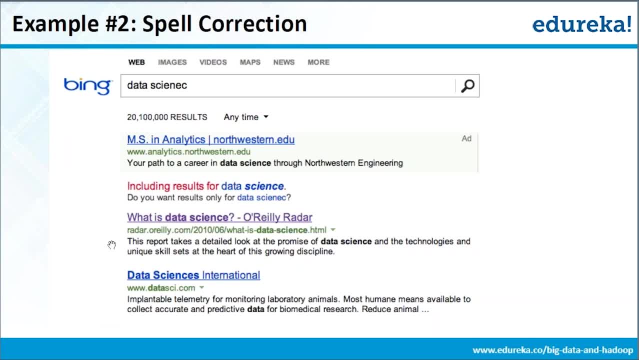 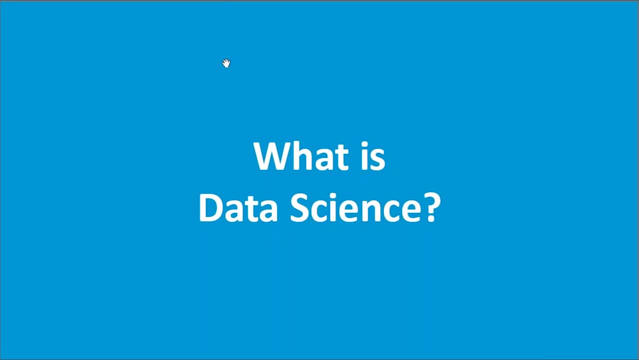 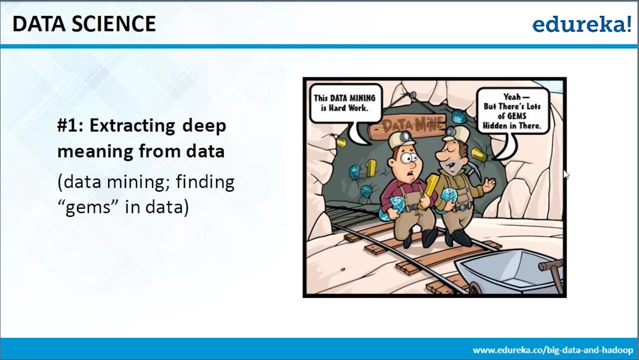 you know, as you all rightly saying, data mining, extensive data mining here, right. so what is data science? so we are embarking on what is data science? extracting deep meaning from the data, finding gems in the data. so data mining is hard work. yes, there's a lot of gems hidden in there. look at that. 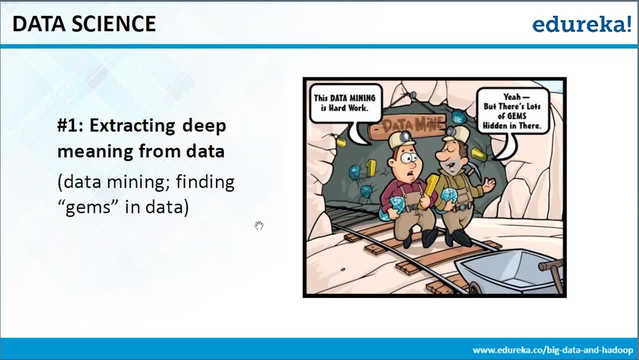 so, friends, just to give you a small heads-up, in good old days, in the beginning of nineteen century, or even little more, little more on to 19th century, right, or 20th century, correct? so we were. all people are running after gold, right? there was a heavy gold rush everywhere, right especially. 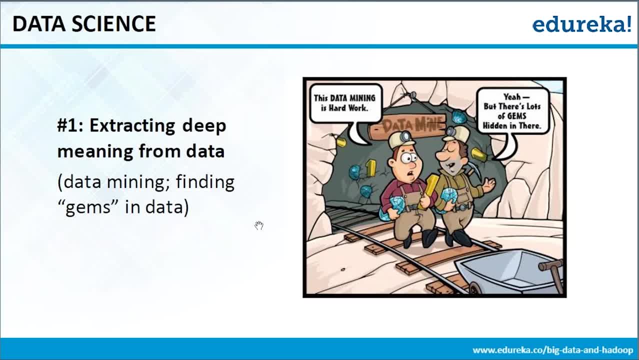 people in the US mass exodus to California. I think that's how people say: you know, you know people even found California right. so there's a lot of science and a lot of history to that. I'm not getting in there. my point is that was the gold people you. 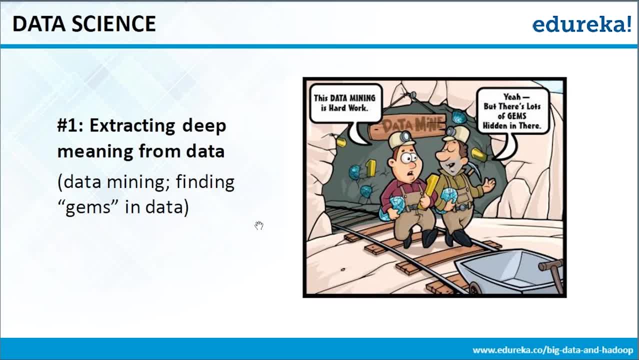 know there's a big gold rush moment. then 60s, 70s, 1960s, 70s and all that you know, middle, most of the Middle East, prospered because you know they call it black gold right, petroleum and all that today data is the latest gold right. so, without mincing any facts, I'm telling you if, if a smart 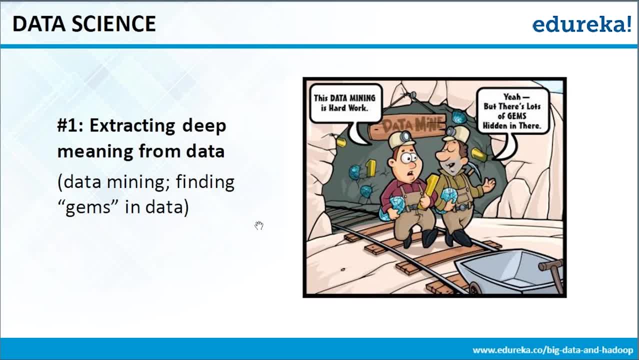 analyst. if that person knows how to mine the data right, how to mine the data and extract the insights or the gems, that person can go a long distance right. so that's precisely the nature of the job for data scientists, right given the data. otherwise you know the data will exist, right it. 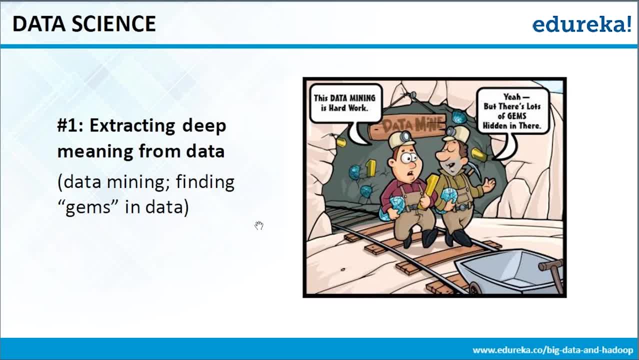 become like a dumb data. correct. if you can really unearth a lot of insights from the data, then it goes very long way, correct? you can do wonders with that. look at some of the common data science task: clustering data and collecting data from all around things like it is the most welcomed щоб. helps you a lot if there is also. I was having a huge number of groups of people in my town that work in looking for some like respect. help them came back within less than six minutes of מאbetween negative existing in the last intense cons-hack network of a mix and make sure that you. 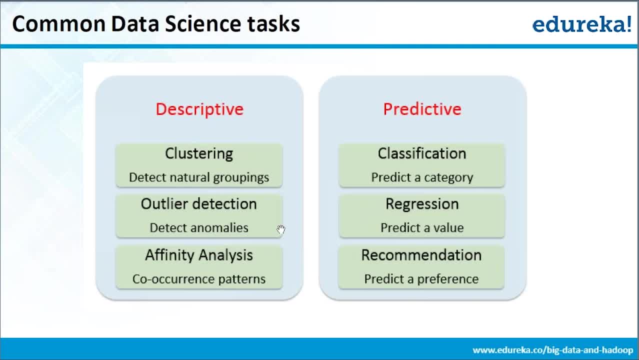 Detect natural grouping. So just to give a small example of that, you know clustering is also, you know all about. you know you look at some patterns correct. You look at some patterns and group them correct. That is your clustering. 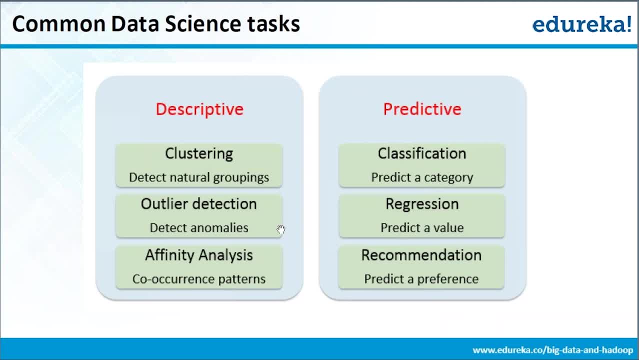 Outlay and detection. So again, you know you look for some anomalies or some bad data, right, Something which is outrageous. So even a data scientist may check with the business analyst, even in this case, because the outlay and detection is more like. 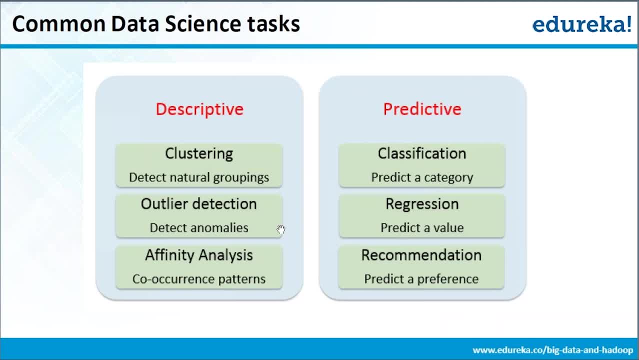 you know, just to give you a small example, friends, you are doing, you know, like a mean and median of somebody's salary, correct, Of salary for a particular city. Then suddenly the one of the salary goes like a million right. 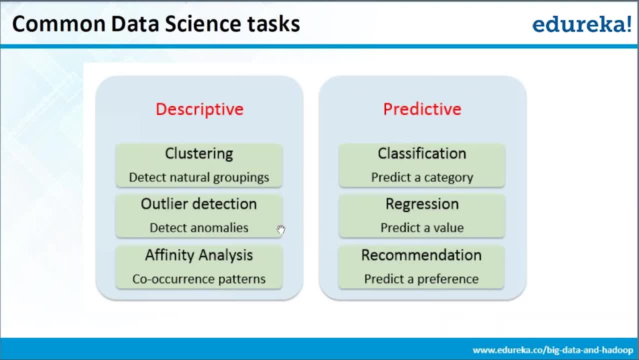 That person may be acting. you know you may be a rock star there. You know you cannot. you cannot exactly classify that as an outlier, because you know you need to first. you need to detect the anomaly and still check and take a meaningful decision. 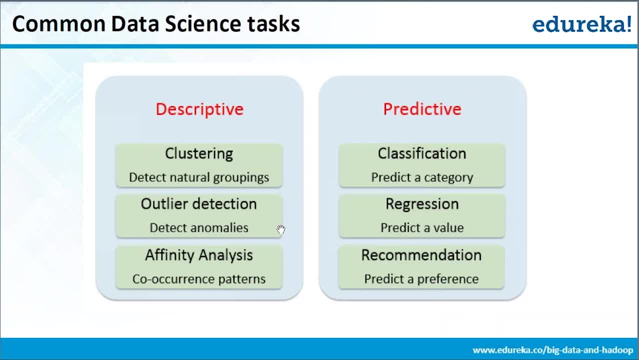 Again, affinity analysis: Look for a co-occurrence of patterns. Classification: okay, This is like predicting a category right, Doing a regression correct. You can do a linear regression. You can do a logistic regression. There are multiple ways to regress and find out. 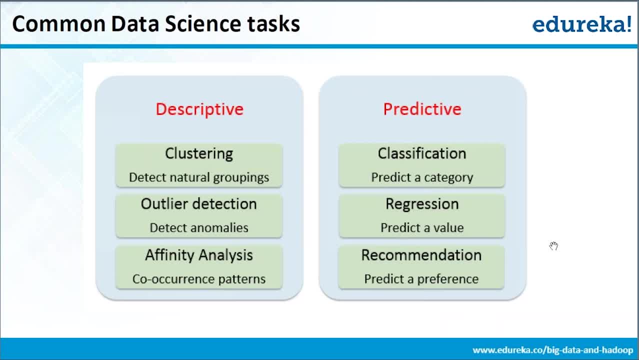 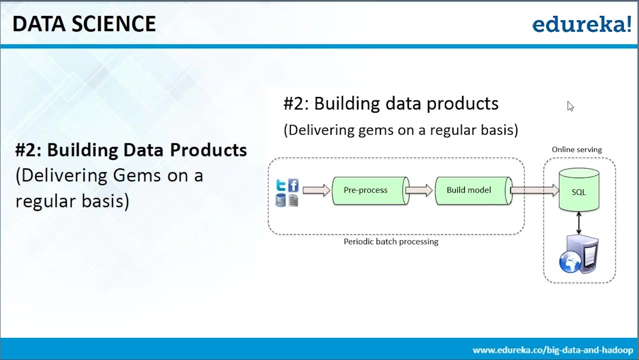 and come up with predictions. right, You can do a linear regression and recommendation, predict a preference, what we saw just now. So these are all the descriptive ones, These are all the predictive ones, correct? So building data products, delivering gems on a regular basics basis, 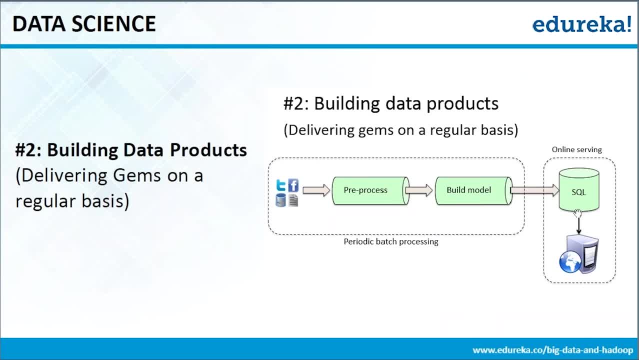 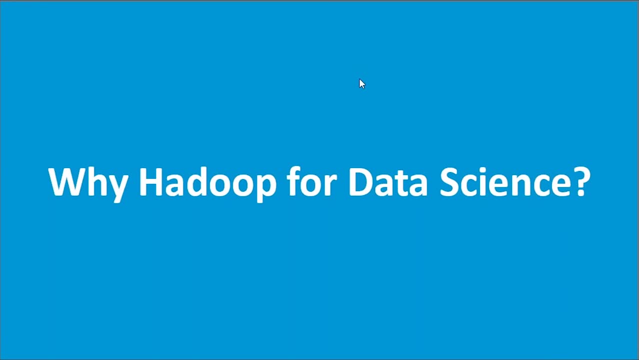 Sorry about that. Pre-process build model and periodic batch processing and throw it onto the SQL So you can. I mean, this is just a model, So you can use anything here, correct, Okay? Why Hadoop Again? why Hadoop for data science? 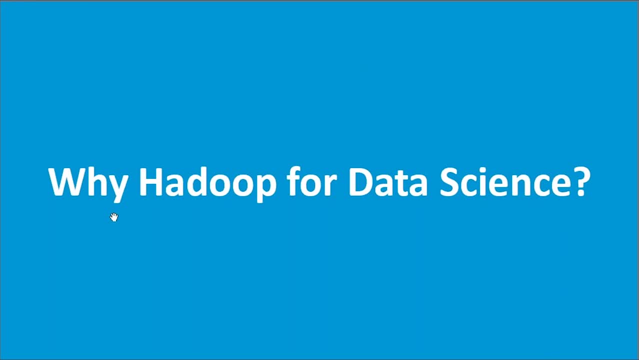 What do you think, friends? You have seen what is Hadoop correct. You have seen what is Hadoop And we got a dipstick view on what is data science. Why do you think Hadoop? where do you think Hadoop will serve the purpose? 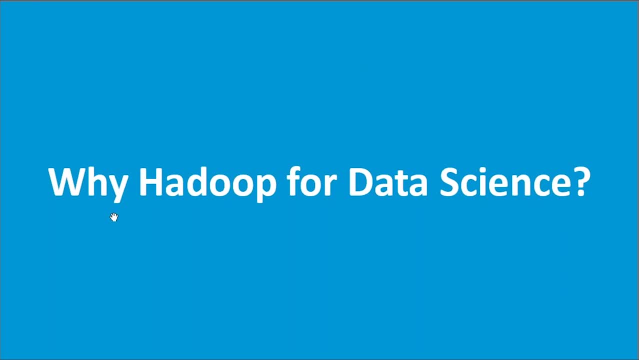 Before I go deeper, I just want to put this question to all of you: Provides economy on scale, Helps the data scientists. Best way to handle high volume data, any kind of data, efficiently, right? So size of the matter, size of the data is really doesn't matter. 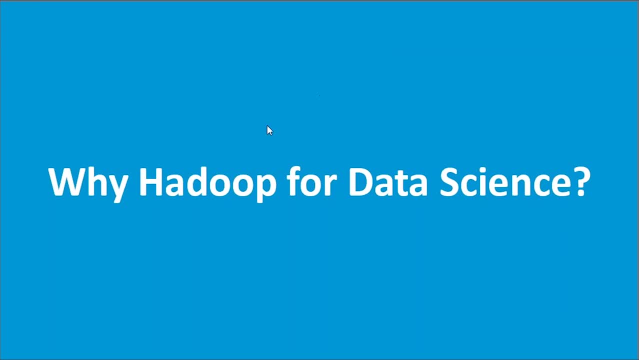 So long as we can handle it, Big data in a systematic way. Okay, So a lot of people are giving Hadoop can work on humongous data in quick time, Quick time. So one thing is, friends, as I told you, 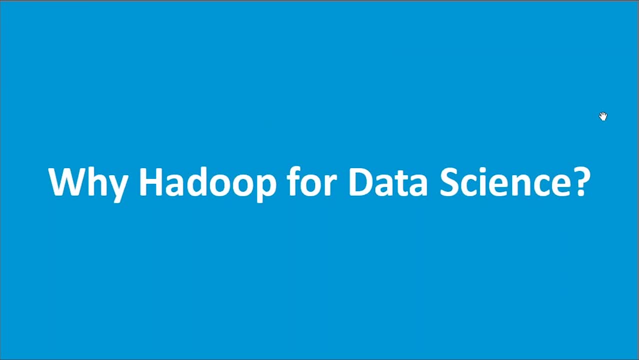 Hadoop provides high latency. So what I mean is you know you cannot hunt down a particular record and all that. It processes things in blocks, blocks of data, correct Blocks of data, high volume of data in a very effective and efficient way. 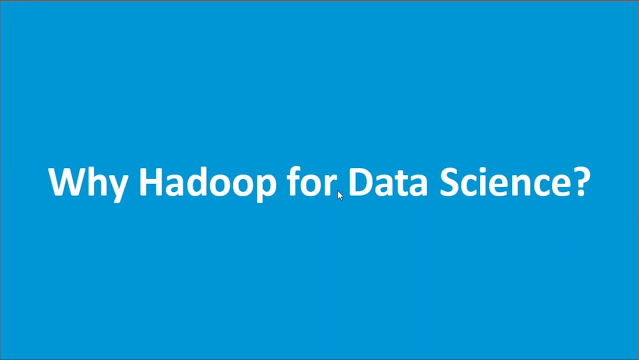 So if, if, if. I want to read something in RDBMS. right, If you walk across a bank and tell them, okay, here is my bank pass book And this is my name, They will be able to pull your record. 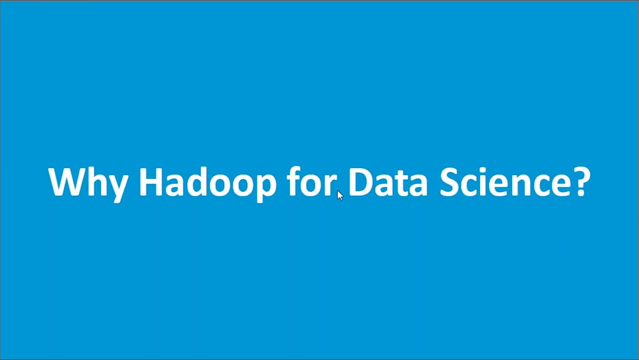 Maybe in a couple of seconds. That is not possible in Hadoop, But if you tell the Hadoop, okay, read five terabytes of file, it can still do that in a few minutes, which RDBMS can probably never do that. 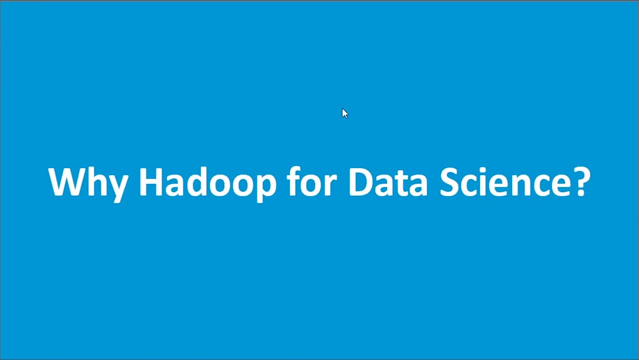 correct. It may probably take ages and fail and all that stuff, because because of scale up architecture, right Here it is scale out Sure. So Hadoop is very powerful And since we are dealing with large volume of data, right. 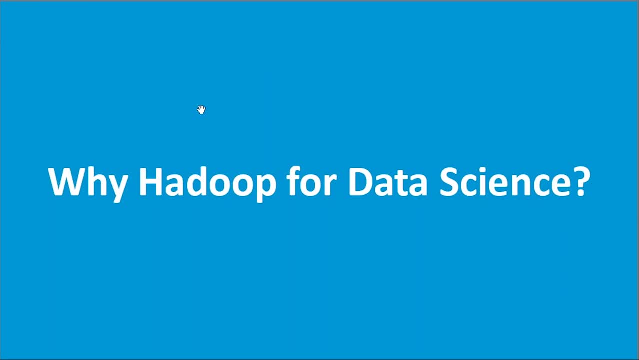 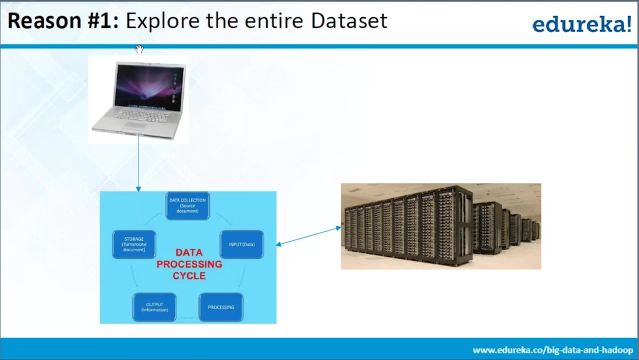 So that is becoming one of the popular choices for even data scientists to work on. right Data scientists, data analysts- you can have any of these combinations to work on. Hadoop. Explore the entire data set, if you look at it. So this is my racks and all that data processing cycle. 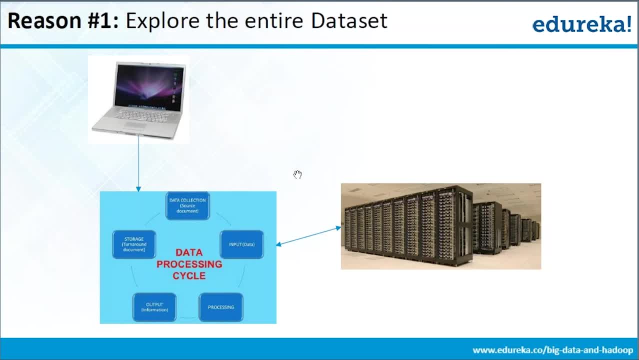 storage, data collection Is Hadoop more scalable. Arun is asking: Absolutely scalable. correct, Absolutely scalable. So I can have, I can go on adding clusters- I mean commodity servers to make cluster, or I can even have more racks. 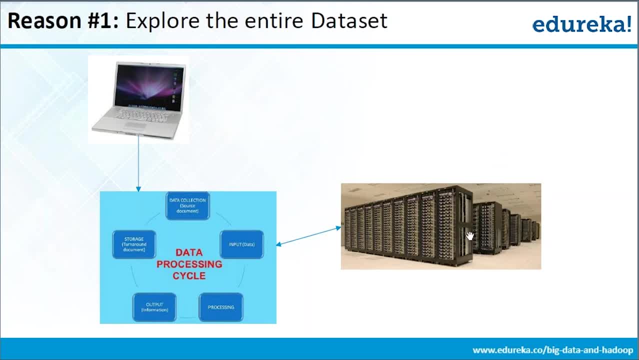 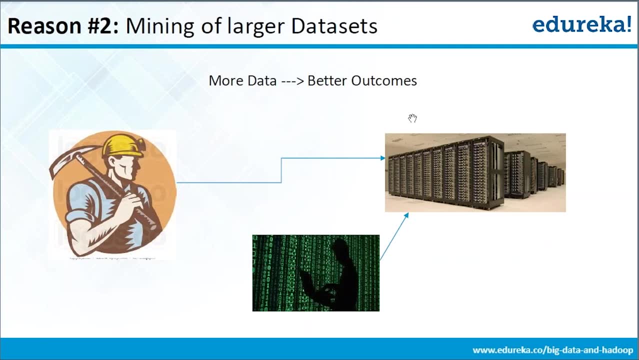 more space, more servers. I can keep adding the servers, Exactly Correct. So explore the entire data set. It's possible Mining of larger data sets, better outcomes. So the more and more data you have, right, Better and better. 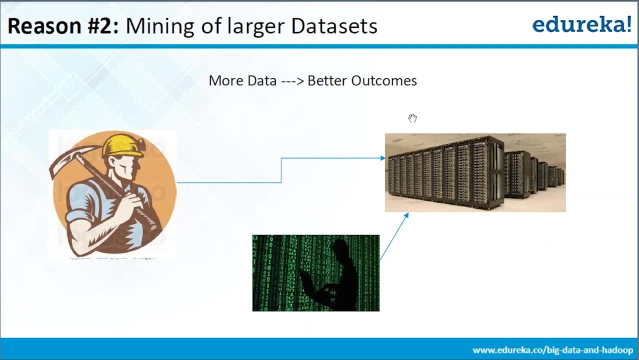 The outcome becomes correct, friends. So it is like even even you know it is for a data scientist. Even if you are training a model, for example, a particular algorithm, people always say: we train the model, then the comp and the. 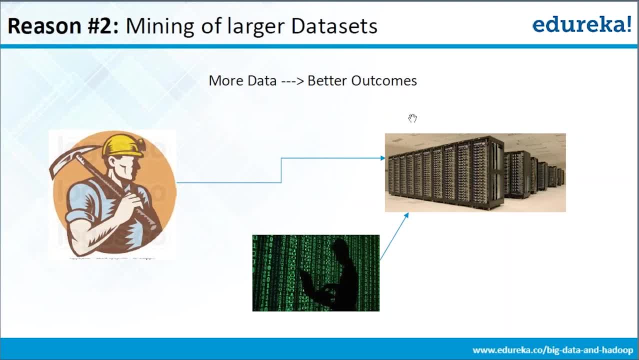 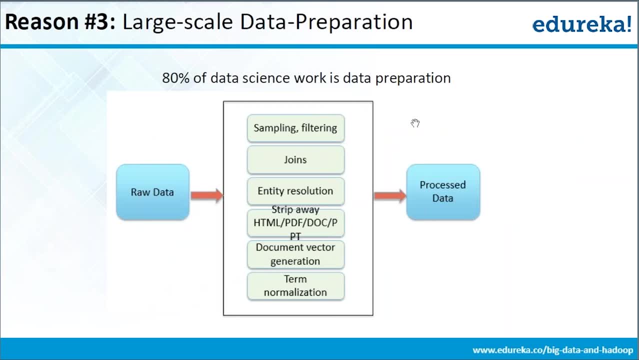 you know, the algorithm becomes more stronger, correct? So they always say that the more and more data, it always yields a better outcome. 80% of the data data science work. you will be astonished. So this is the. this is the truth. 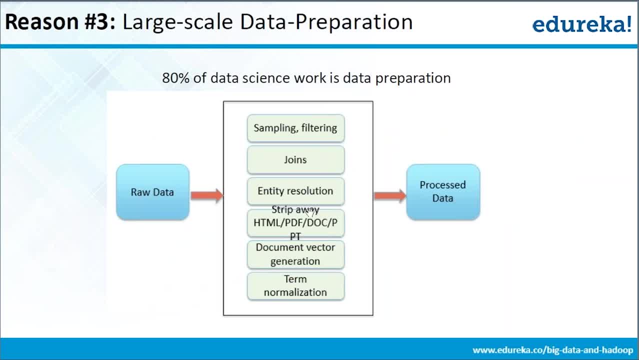 Actually raw data sampling, filtering, joints, entity resolution, strip away all these things, document vector generation, term normalization, right. 80% of the work is actually involving the cleaning up the data, correct Data preparation. They say they do a lot of transformation. 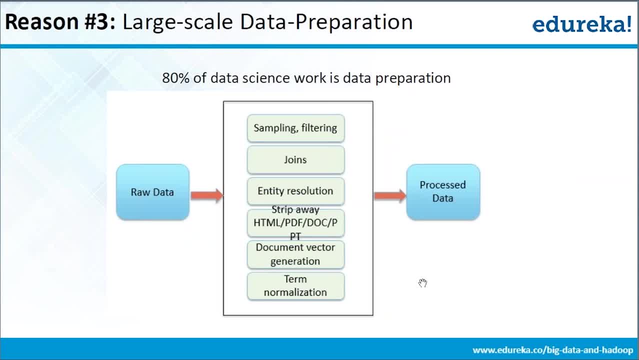 You know, when they say cleaning up, right They, they set the data because it may come in different formats. It may have some web bots laying there, So they need to make the data, They need to give meaning to the data before the data gets analyzed. 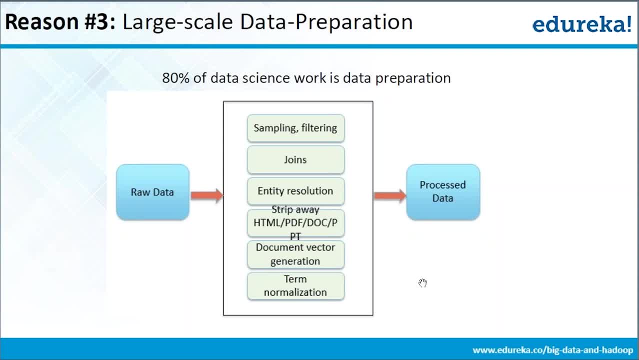 Correct, So the data has to be in shape. Generally, most of the times, the data will never be in shape, Correct, So they need to make the data, make it available and and, and you know, make it consistent so that it becomes good for analysis. 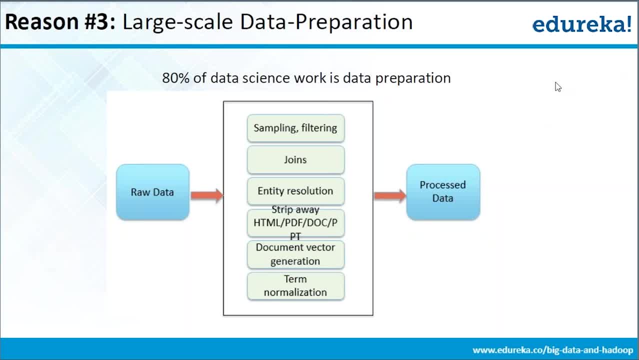 Correct. What are the? okay? just one question, friends, Before I go further. there is a question here: What are the other frameworks, like Hadoop, for data science? I think, Ravindran, there are a lot of you know. 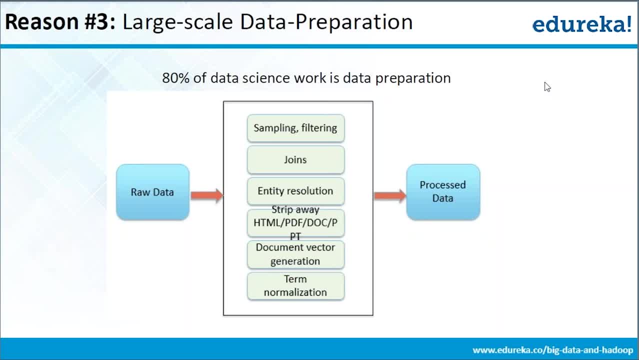 Hadoop is taken in conjunction with data science because of its ability to handle large data, Ability to handle large volume of data, Ability to handle high throughput, Correct- All these are plus factors, So people also do. if you're only looking at some regression and all that. 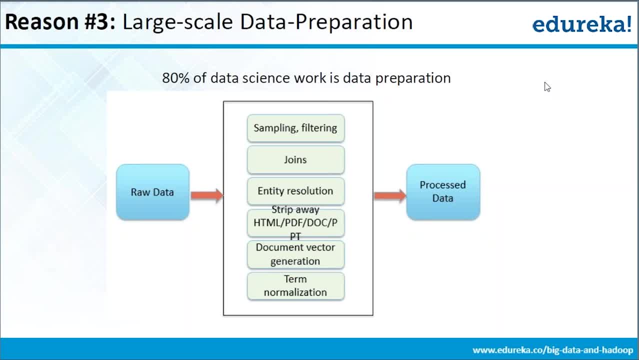 I think, yeah, you can look at, you know R, you can look at SAS, you can look at, you know some of these tools as well, which provides you a statistical insight onto your from the data science perspective. 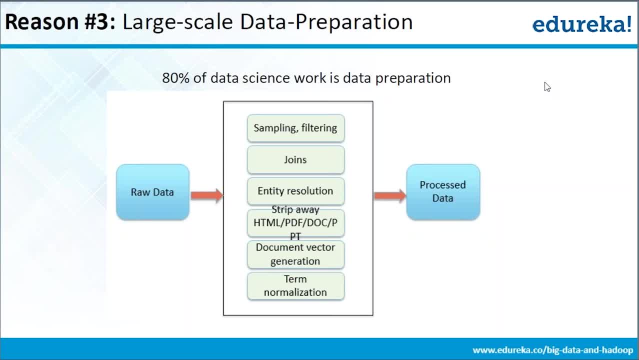 Correct. So that is one way, but you can always use it in conjunction with Hadoop. That's what we are trying to say here. Correct, Okay. RDBMS uses schema on write, whereas change is expensive, High barrier for data driven innovation. 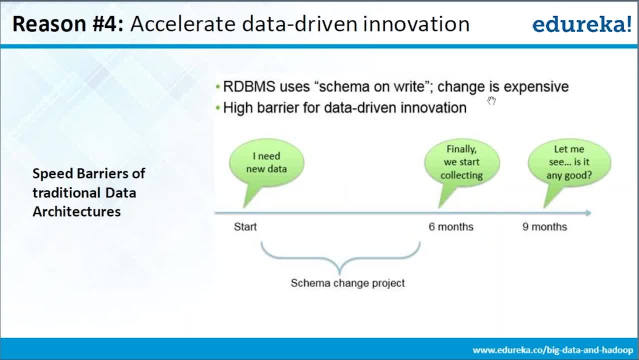 Sure Speed. barriers of traditional data architecture. I need new data. Finally, we start collecting. Let's see. is it any good Correct? So RDBMS has lots and lots of you know schema on write Meaning without doing anything. 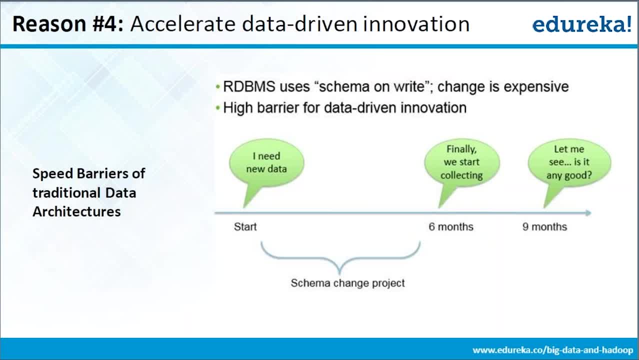 right Without doing anything right Without doing anything. RDBMS has lots and lots of you know, schema on write Meaning without doing anything right, Without doing anything right, Without doing anything in the sense, without even inserting the data. 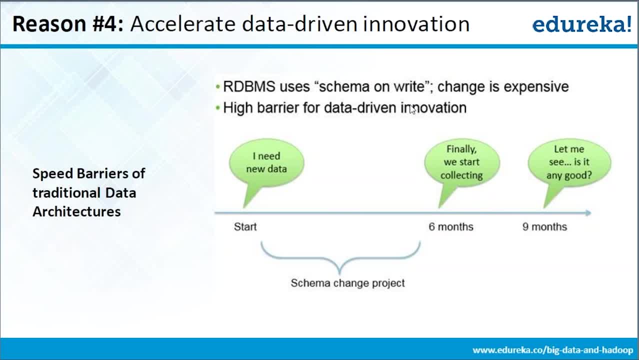 before you insert the data, right, You need the schema in place So that any change, right, You need to go, go to the, you know DDL, you know, make all those changes. It is quite expensive And 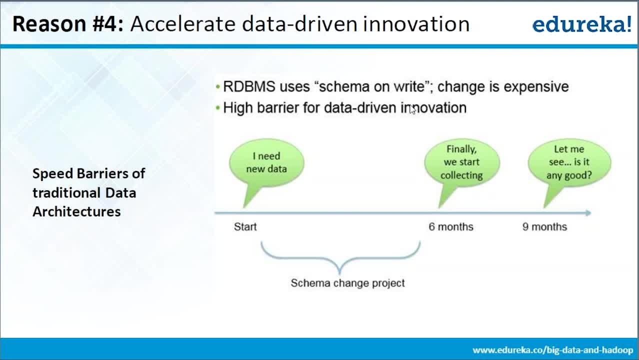 you know, that's not the way we work today, right? Because the data will come in a very sparse format. The data will be completely unstructured. So those kinds of things- RDBMS, BMS- are already falling flat here. 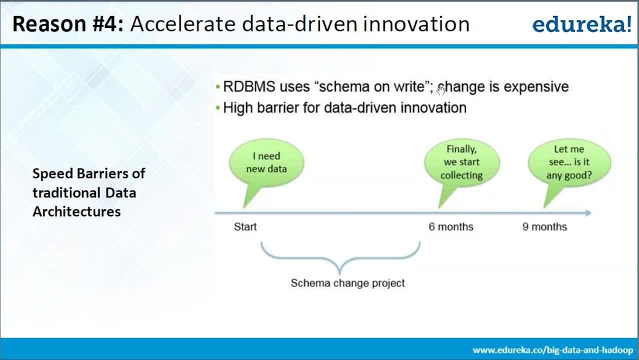 Right, So so it is really required for you, for you to have an accelerated data driven innovation When the data is predominantly unstructured. you need more flexibility here And you need, you know, Hadoop, especially. it supports schema on read. 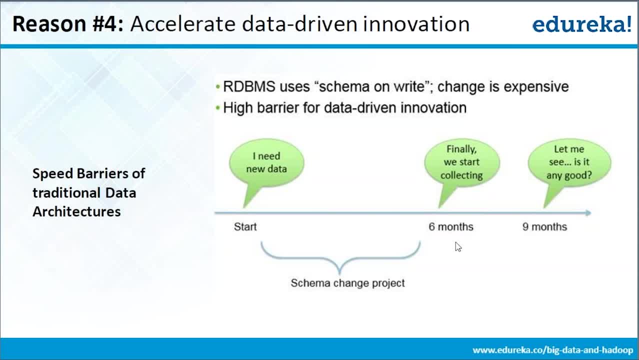 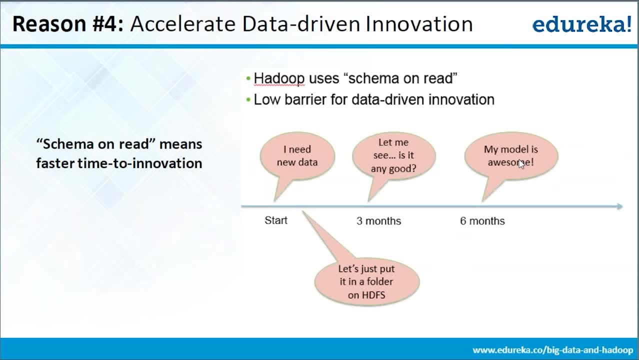 versus schema on write. Correct Things can happen pretty fast and very volatile. Schema on read means faster time to innovation. I need new data. Is it any good Low barrier, Correct Data driven? So that's precisely what we want. 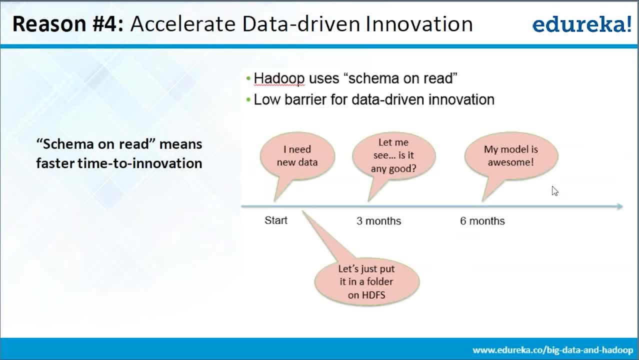 right If it is a high barrier, meaning there's any changes. if I want to do it with the data, you know you need to go, go and make this changes to the schema, everything right. That's going to tie it down or discourage anybody who wants to pursue. 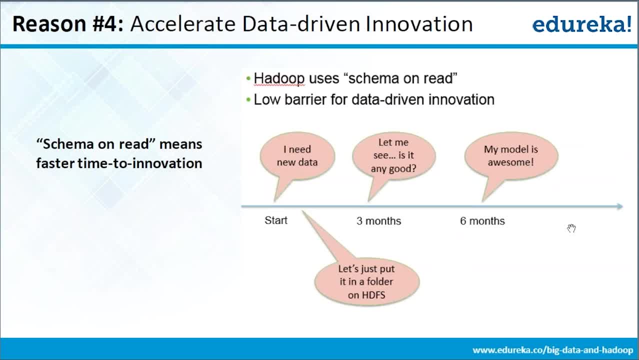 or who wants to innovate in the data front, Correct. So this one is. it's a radical thought. It completely makes it very, very easy for anyone to move forward, Correct. So so, so, so, so so. 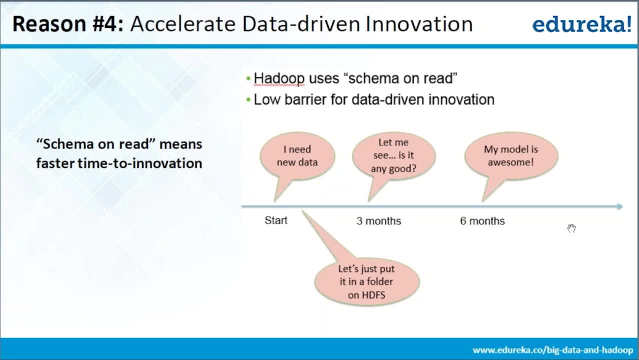 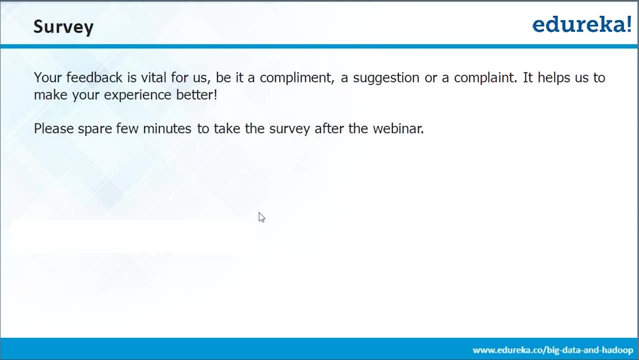 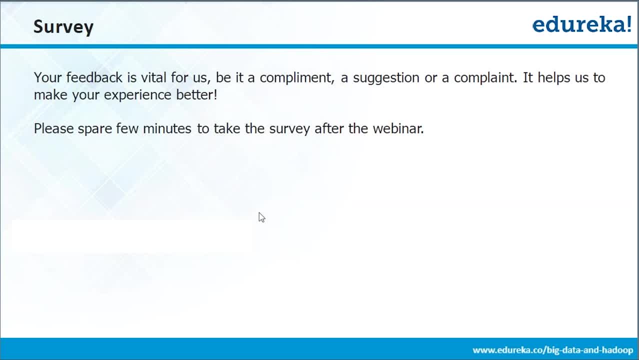 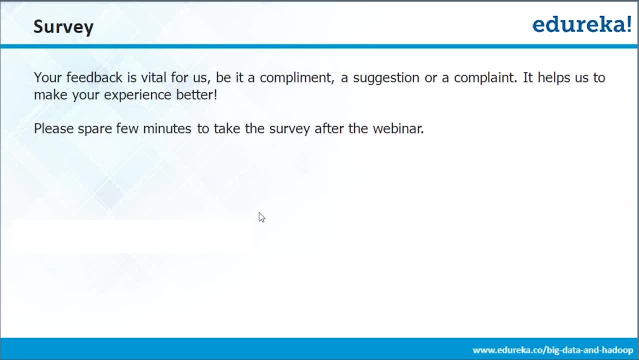 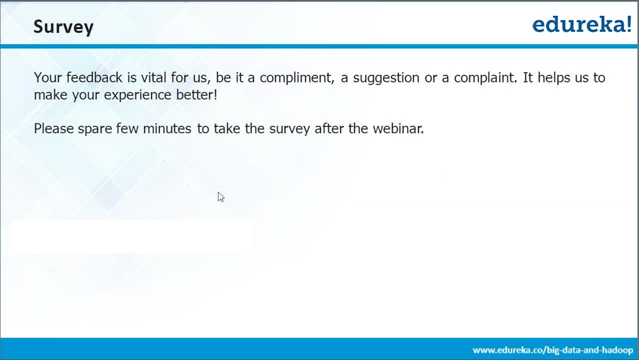 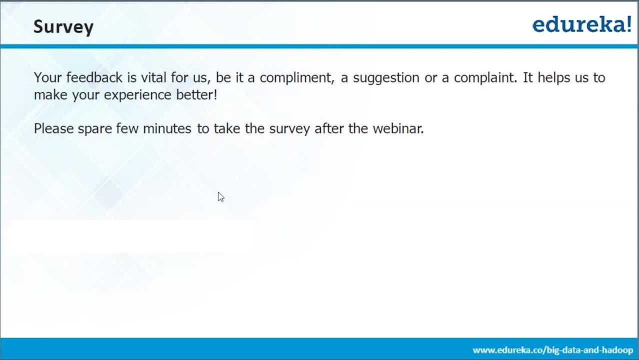 between these two things, correct? Sure, okay, So I just want to understand the set of Hadoop environments- very costly or moderate. Mohit is asking: It's actually friends. can I just do the demonstration and come to these questions, correct? 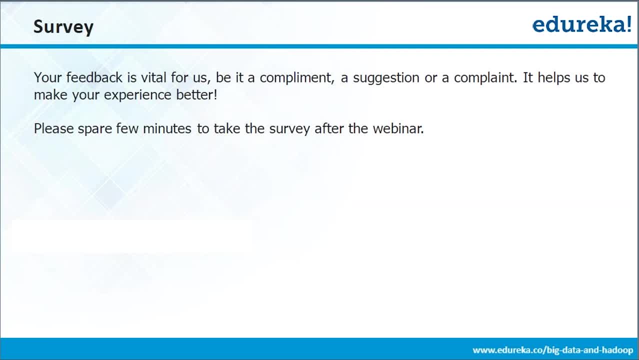 So I will probably finish that because we are not done there. We can, yeah, required. the setup is not very expensive, Mohit. If you have the expertise, I think it's not so expensive because it's open source. Hadoop is open source, end of the day. 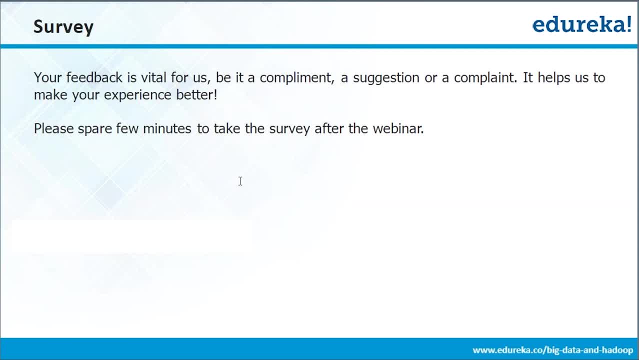 We can use MapReduce. only Soumin is asking. It's not true, Soumin? There are things like Spark- is there? there is things like Storm- is there? right, There are so many processing frameworks that are available today, correct? 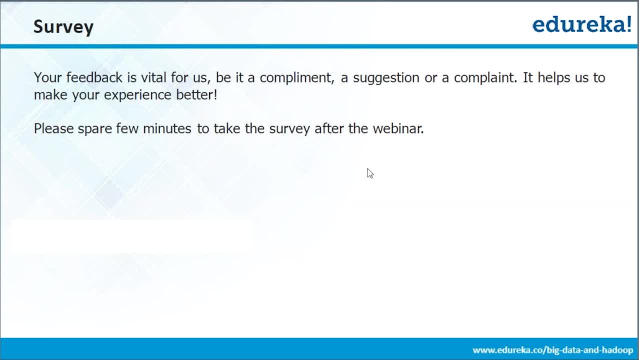 Okay, So of course, towards the end, friends, I'm going to do a. you know, please complete the survey once you're done, right, Once I'm done, I would request your feedback. You know that's going to be very important for us. 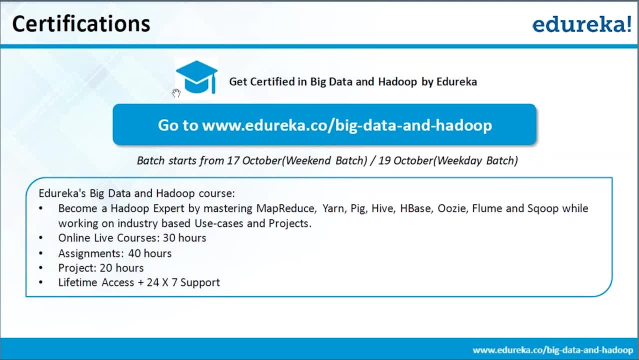 So let us certifications. I think I don't know what they have to say here. Okay, there is a big data certification. Okay, you can always aim for this. BAT starts from 17th October. you know, you can give it a shot, sure? 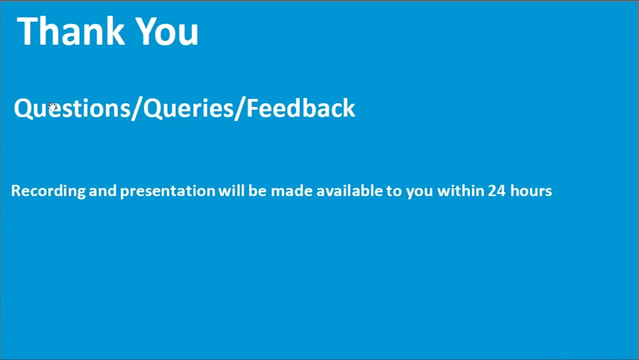 So that is something. starting here, Reading and presentation. okay, So these are some of the features of Hadoop. I mean Edureka. so I just want to highlight this. Then I want to move on to the. this is it. 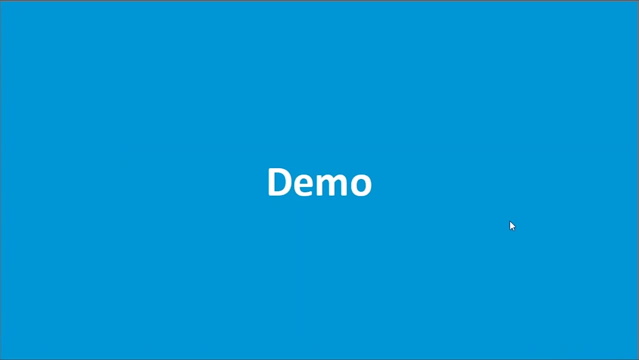 Just a second. thank you, Friends. one second. So that is a demo. So can I finish this and go to those slides? I think I missed the demo part, So I'll quickly show you. you know any analyst right data scientist. 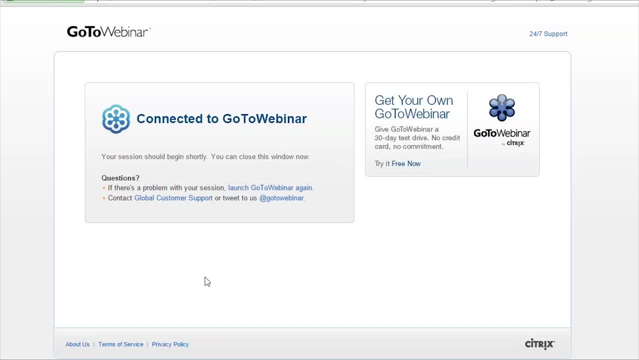 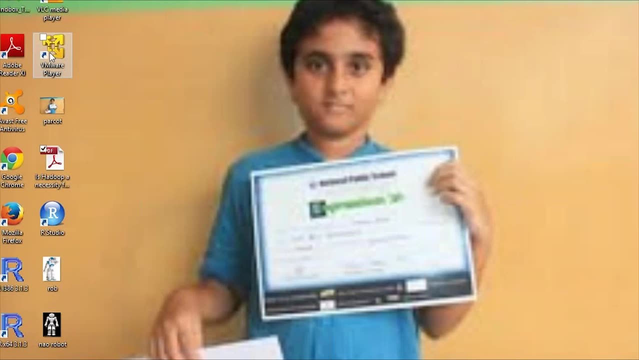 any data scientist, right? They also. they are quite familiar with all these things, right? they are also technically equipped- Most of the data scientists are. they are. they have a good background in mathematics or statistics, correct? And they also have a good analytical attitude. 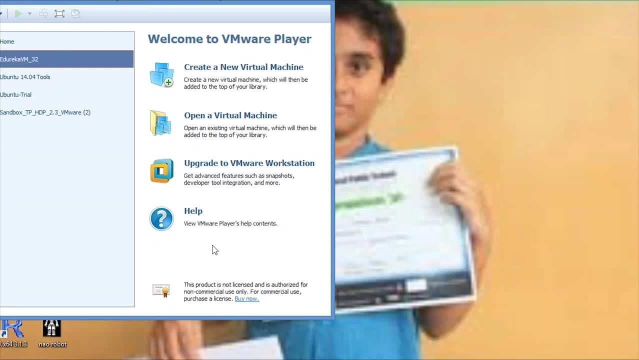 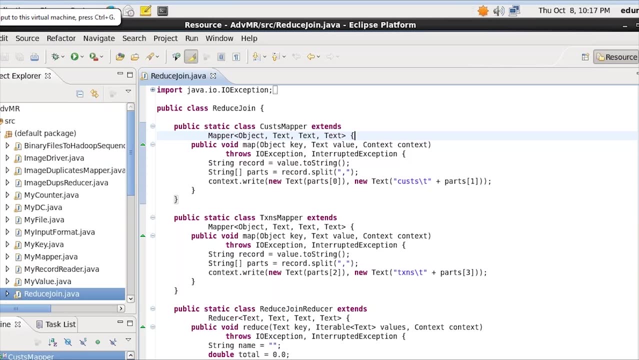 So I'll just show you a very quick, you know, a specific example: small program, how we, you know, I just want to do a quick analysis, fine. so, friends, I am just doing a quick, you know, I'll show you this demo. okay, I have a. 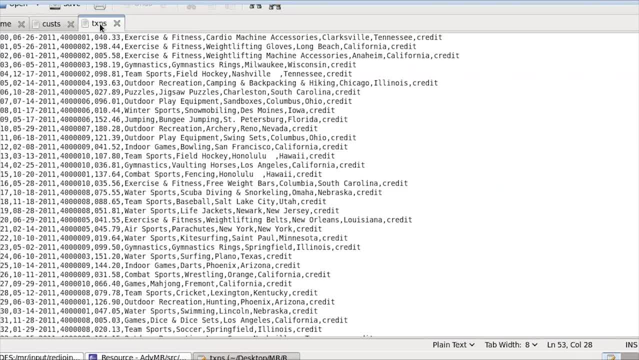 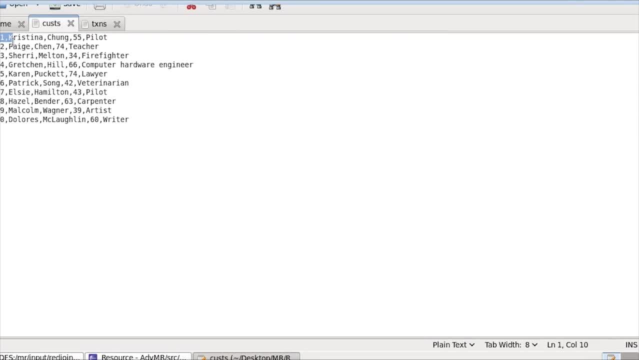 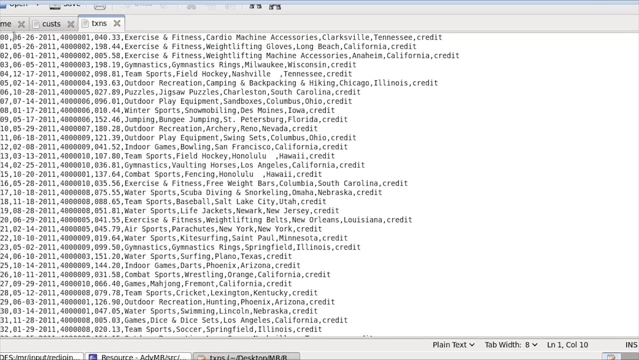 couple of data sets. okay, I have a couple of data set. one is the customer. fine, you find all the sorry customer records are here. this is a customer code: first name- I'm sorry. last name, age, profession correct, sure, and you also have. you also have transactions for that customer. correct the transaction ID and you have. 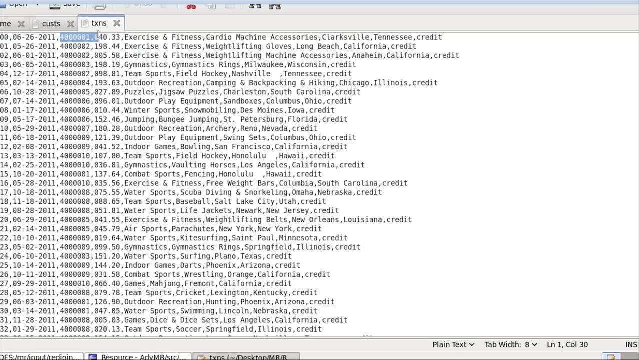 a date, transaction date, customer code, the sale value right here is my category and if I have a customer ID in my phone, I do have a transaction ID in my phone. here is the product and i have the city state payment mode. are you all clear with the data set? 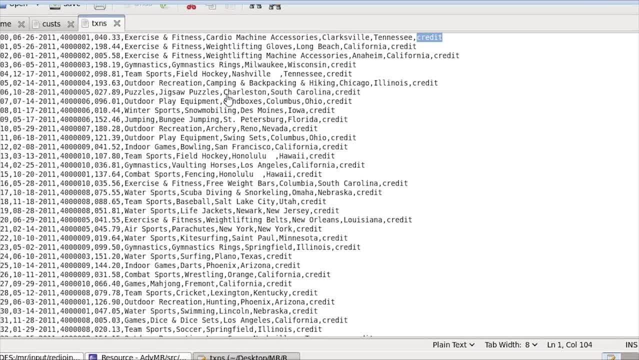 friends, i haven't told you what is the problem i need to do, but are you clear with the data set what i'm trying to say? you have a customer file and you have a transaction appropriate transactions file. is that clear so far? awesome, okay, very, very simple. i you know what i want to. 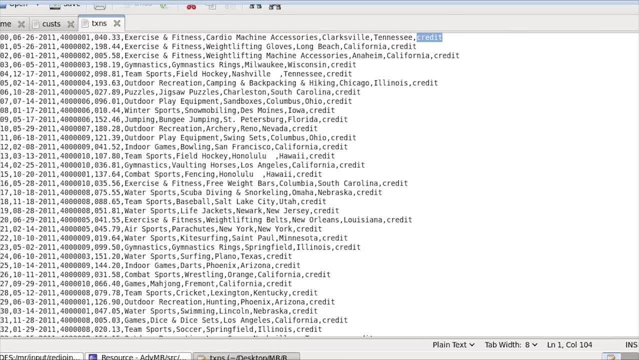 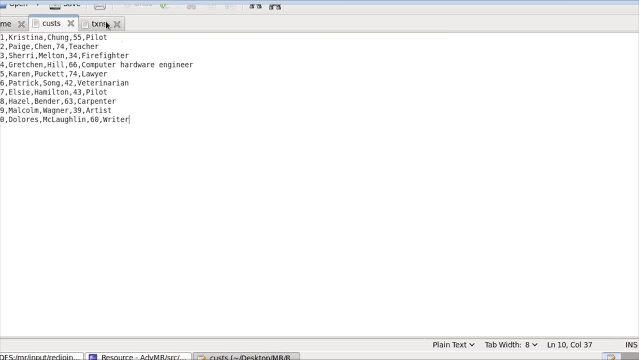 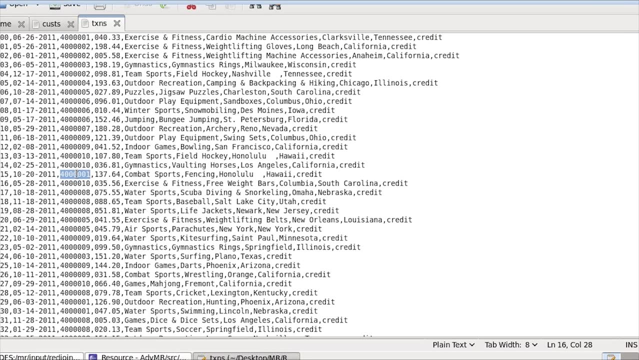 do the problem statement is all about for each customer. i have about 10 customers right here: one, two, three, four, five, six, seven, eight, nine, ten. i have 10 customers for each customer. i have multiple transactions right: four, zero, zero. one is one of the customers and you know, yes, that person. 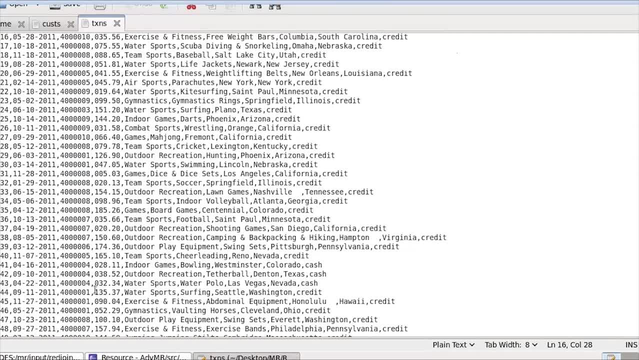 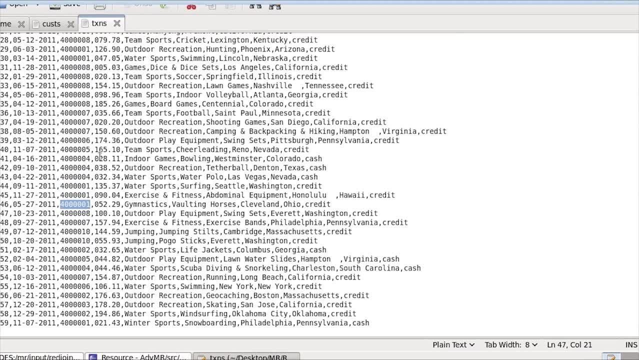 has christina, right. christina has bunch of transactions here here. here, six, seven transactions are there, right. so for each customer, similarly, i have multiple transactions. now all i want to do is to print for each customer. i want to print the name and i want to print the number of transactions and i 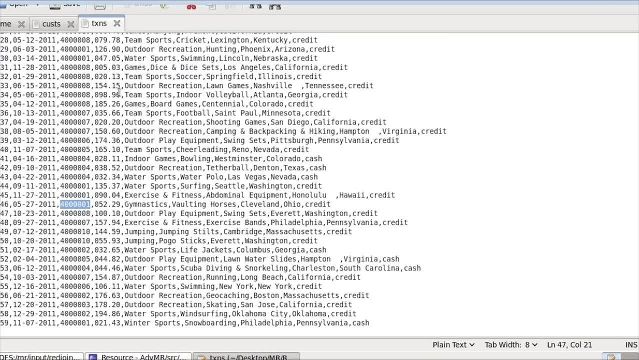 want to print the total number of transactions, uh, total sale value. right, i need to have a sum of all the uh transaction amount, correct for the number of transactions. is that clear? so how would you do if i give you, if i just give you, these two tables in sql? 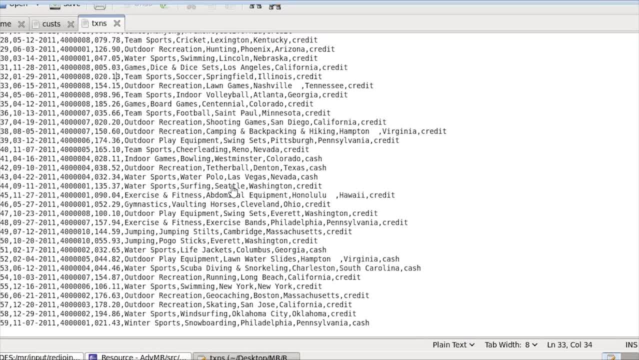 what's your thought process, friends? how will what will be your approach here? write to join- fantastic. so what will be your joining attribute here? join and group, exactly joining all the customer, correct? so how many lines would you do it, friends? how many lines will be your sql code? two to three lines, okay, sure, okay, it's not. 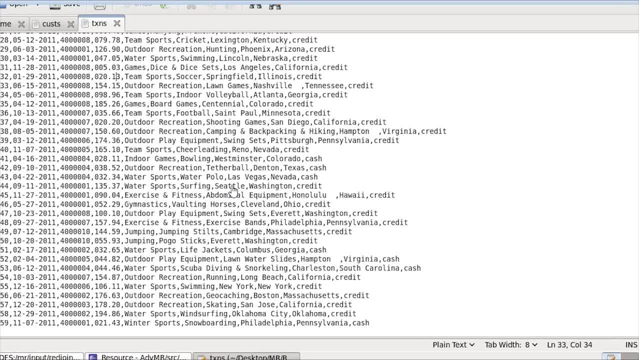 I'm going to show you the program in Java: Four lines, okay, whatever, right? So it is going to be a little more. you know it's Java MapReduce, right? It is if you're going to use joins and other things, right? 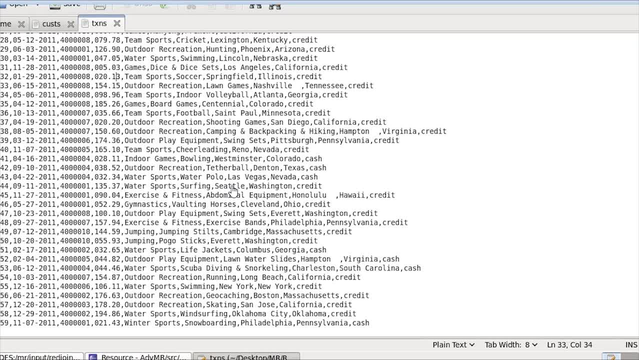 My natural choice would be to use pig or hive. right, They are pretty fast and you know they are. you know, hive pig is a declarative language and it's really quick that way, right? So I'm going to show you a traditional MapReduce. 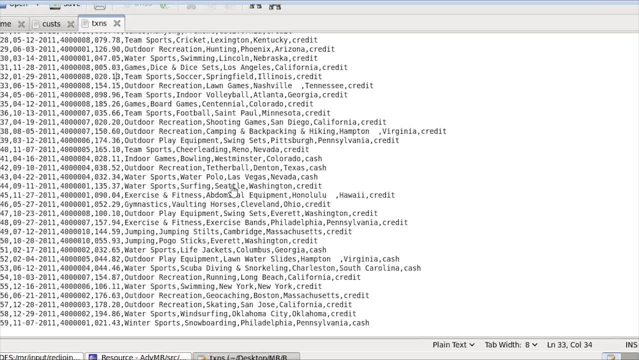 So, as a data scientist, right one thing. what I want to tell you is you need to know which tool to use where, because data scientists- they analyze the data, that's true. They also know- they should know- how to optimize an algorithm, and all that. 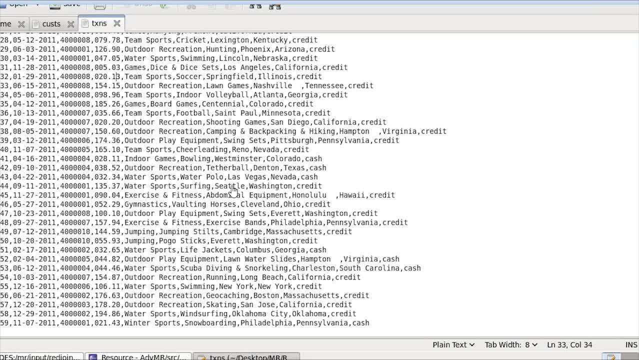 They are very scientific too, right? So I'm going to show you in a very traditional Java program like how we do the joins and other things, right? That's what I want to demonstrate today, correct? So look at this. 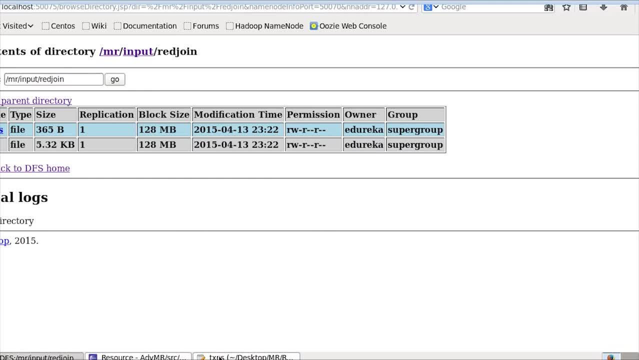 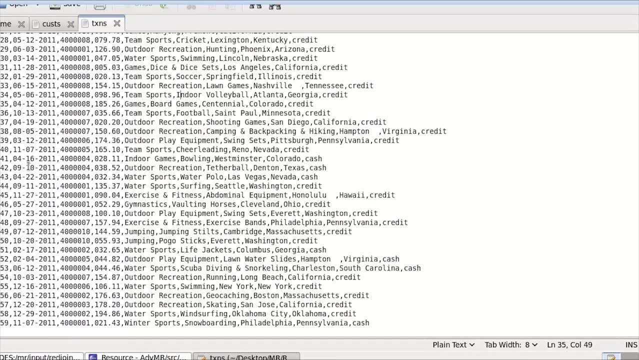 This is my. these are the two files. I've already moved it to HDFS, correct? This is my HDFS. So if you look at this, these are the two files. I've already moved it. fine, So in my Eclipse, correct. 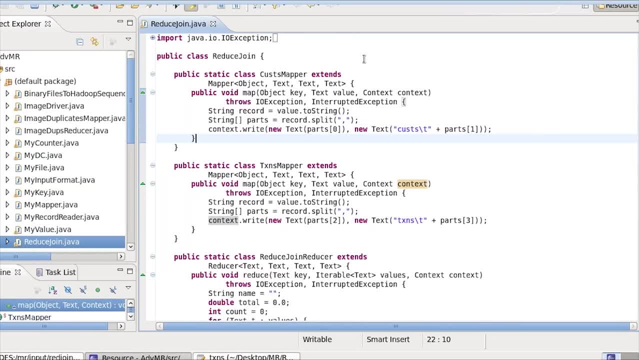 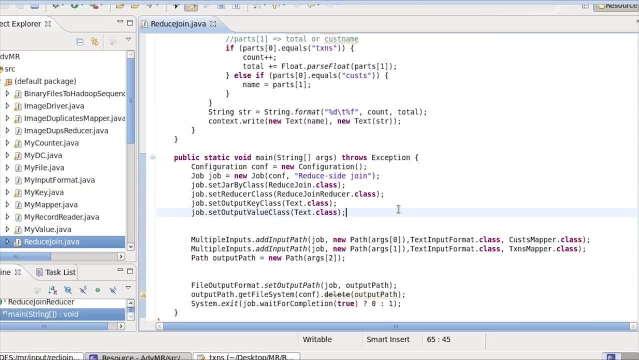 I have something called customer mapper. So I have, like you know, let me go to the driver class, my main class, right. So I'm saying how to move these files to the HDFS. okay, I will do a put command, Abdul. 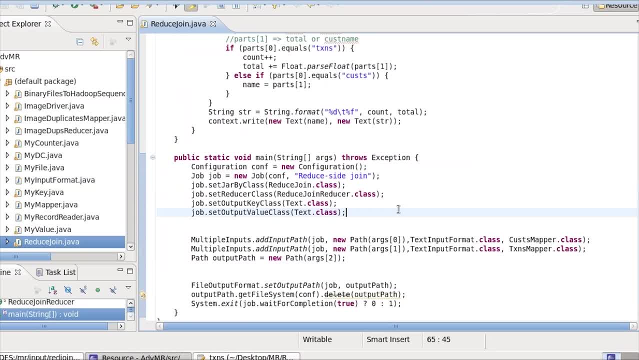 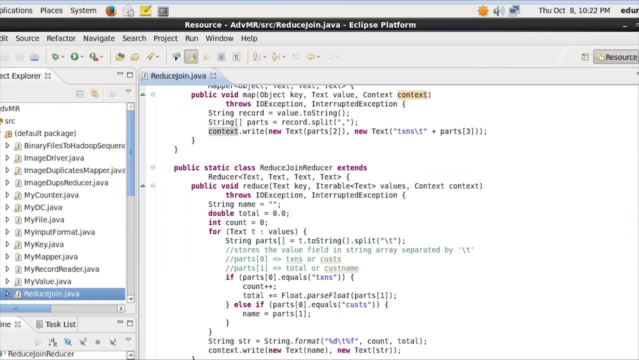 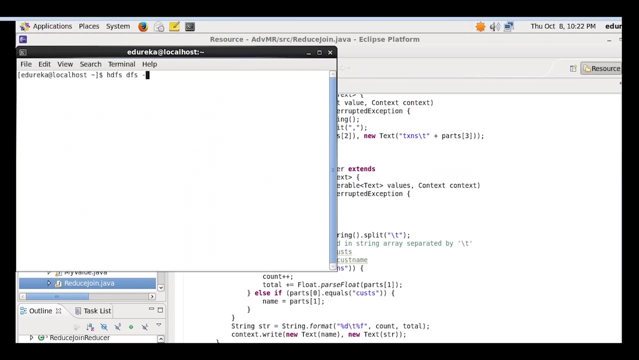 I will just say HDFS, DFS. you know, I'll just say something like this. Let me just type the command for you. It's a pretty easy step. I just say HDFS, DFS, put whatever is the file- X file. 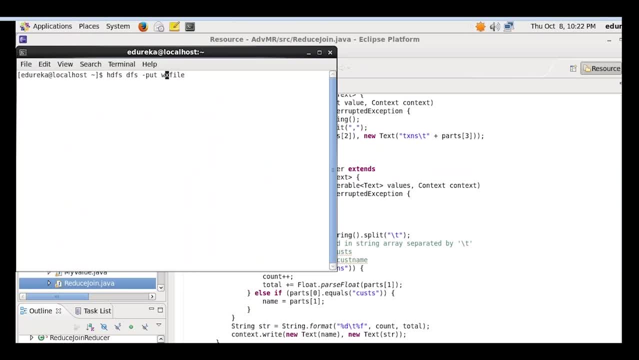 whatever is the file, right. Whatever file, Put that in whichever location you want to put it in HDFS- Correct, HDFS location. Is that clear? How do PFS put: Yeah, that's right, Correct. So this is my syntax. 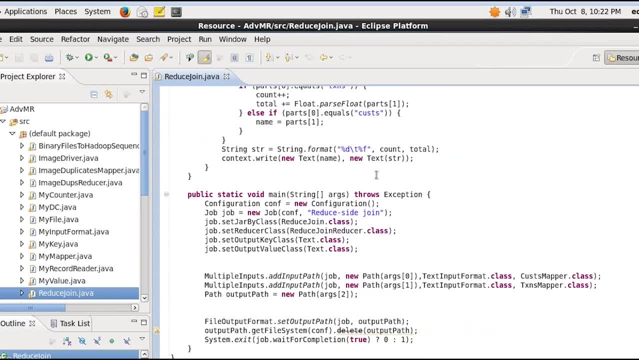 So this is what I've done. I've already put it. So what I'm doing, friends, the mapper right, I want you to understand. It's not so easy to implement in Java, but you know it is quite powerful once it is implemented. 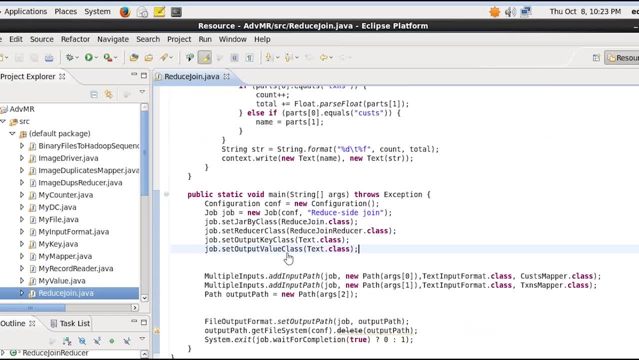 So I am saying, my, I have got, you know, my, I have got two mapper classes running right. My first one is, like you know, I'm giving command line argument when I'm going to execute the jar file here. 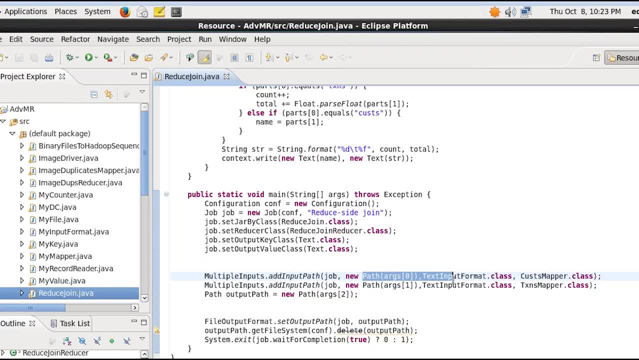 once I build the jar Sure. So my path argument: zero, which is zero base right. So I'm going to give the location of the customer mapper, which is located in this location, right, HDFS. This is where I have. 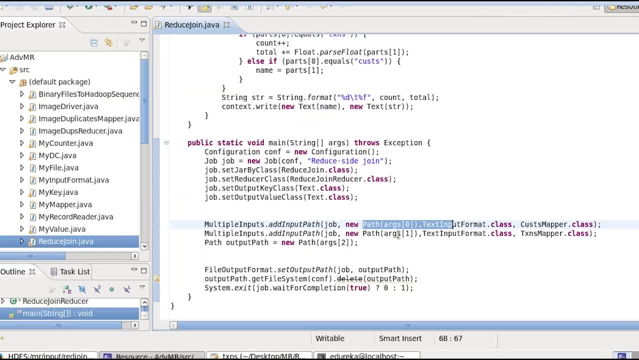 Sure, Correct. This is my, this is my second one, Correct, This is where my transaction mapper is running, Correct. And the third one is the output, what I want to generate for, because that's the problem statement, what I mentioned. 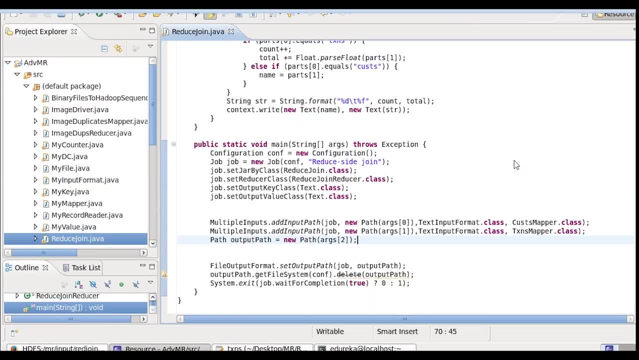 Sure, Okay, now Jagdish is saying he has already done Big Data developer from Hedureka. Sure, Jagdish, See data science. you know you can. You can do all this right. go to: you know machine learning algorithms. that's covered in depth and you will also get to do a lot. 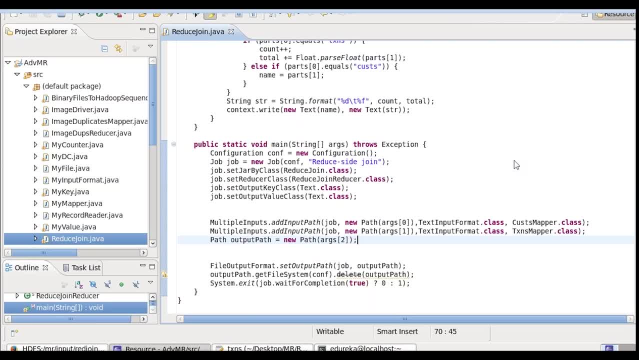 of business analytics correct. you'll also get into the recommendation engines, business analytics. you will do lots and lots of exercises in R and how to connect, how to work on R in conjunction with Hadoop. all those things are coming in there in Jackdish, right, sure, okay. so from my, you know what? 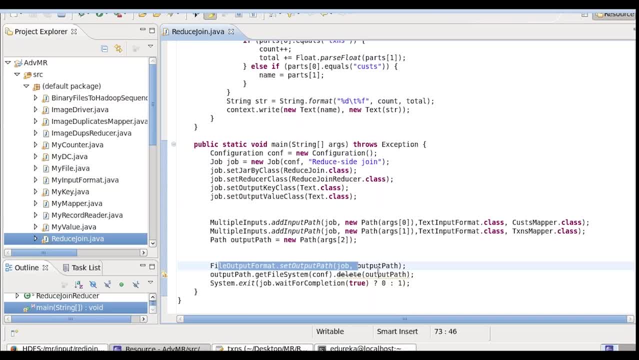 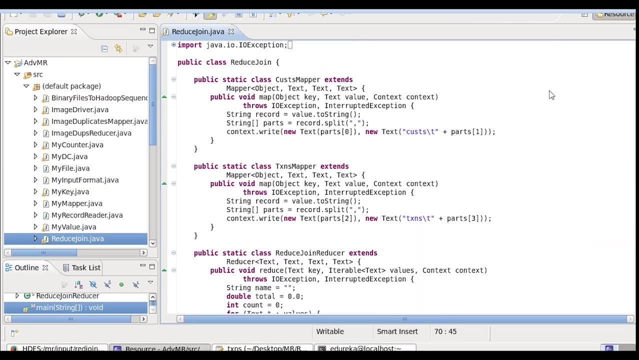 I want to do here is I'm going to do a you know, output path, like: okay, this is, these are all the standard ones, you know. I'm just giving the output path, which is my third parameter, right? so in the first mapper, what I want to do. I want to split this correct. I'm writing, I'm, I'm, I'm reading the. 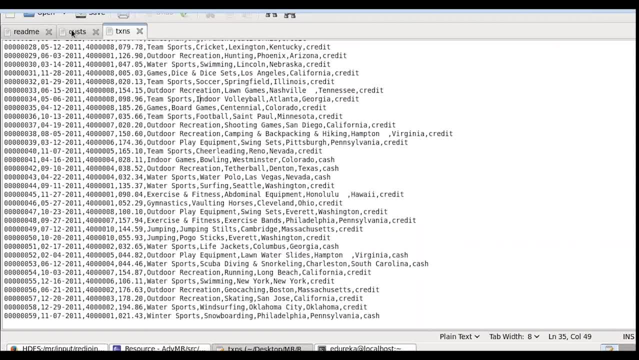 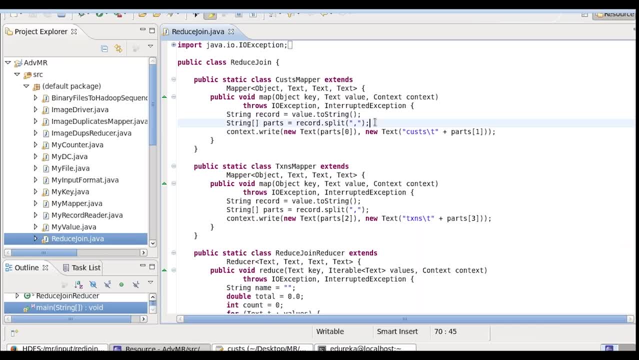 file, which is this file. I'm reading this file, sure, and I want to split that into you. you, based on the comma, right, it's a string array. I'm giving a string array, I'm doing a record dot split based on the comma, because comma is the field separator there. then I'm, I'm writing the. 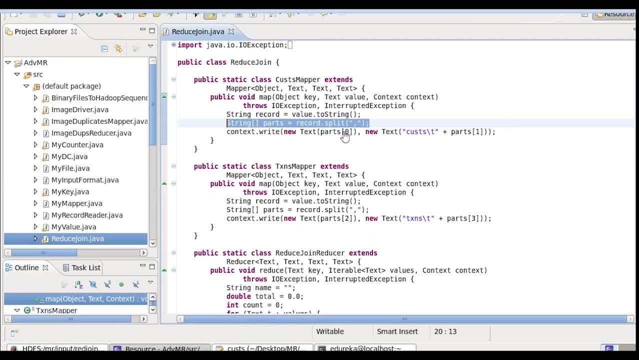 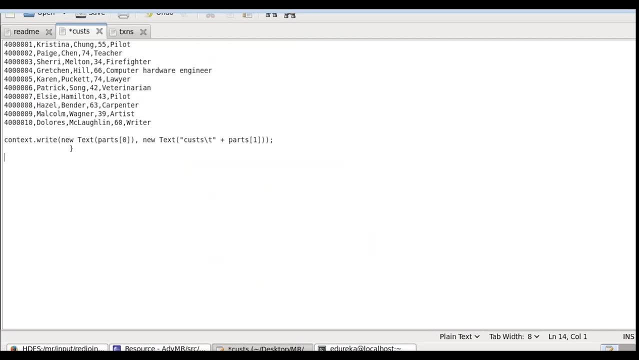 mapper's output as this: one parts of zero. let me just give this, let me just give this, friends, so that you know, it becomes very clear to all of you. this is my mapper's output, right? so what is parts of zero, friends? I'm just curious to know what is parts of zero here? all right, you all got it correct. parts of zero is. 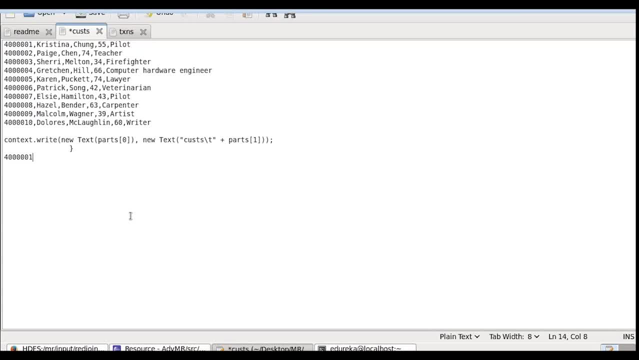 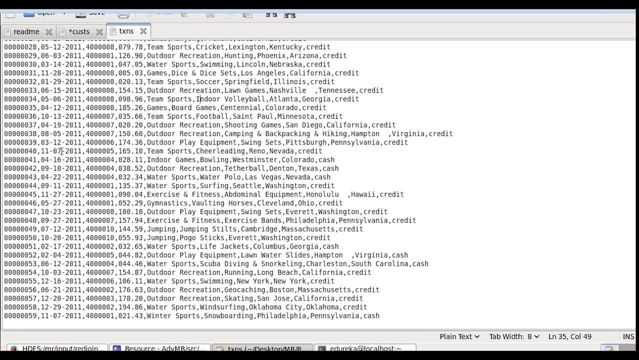 this one, sure, and what I am writing? this is my key, this is my key. this is my key and this is my value. this is my value. what is parts of one here? first name, perfect. first name, right, so it is christina, correct. so this is my cust. this is how it is going to be written. what about the? 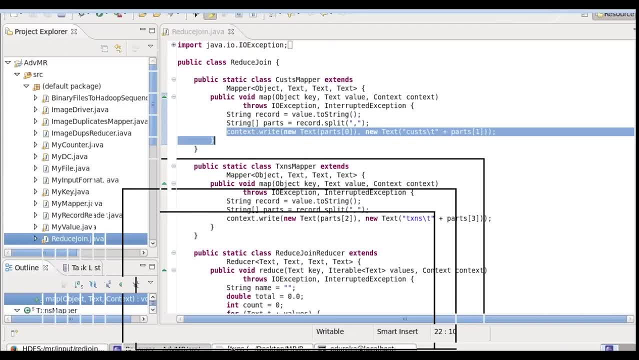 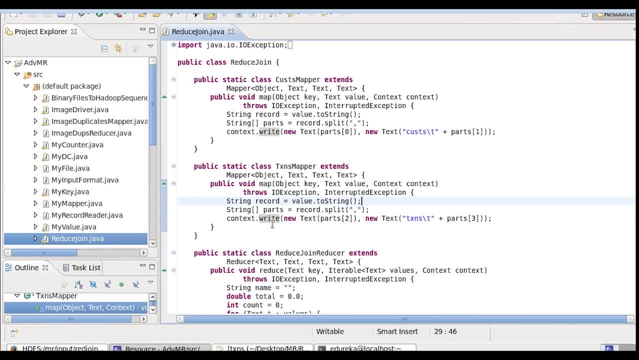 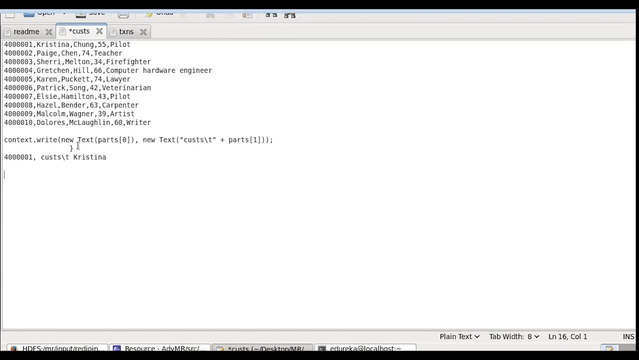 transactions. can you similarly help me here in the transactions mapper? what i want to do? record is equal to value to string. okay, i'm similarly splitting right. so before i write christina, right. friends, one thing i forgot to tell you, i also write. this is how i write right: customer slash. 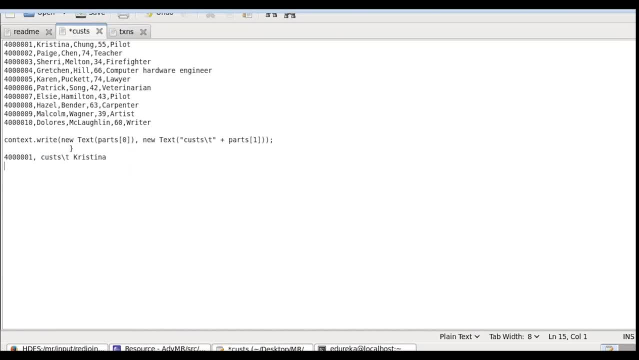 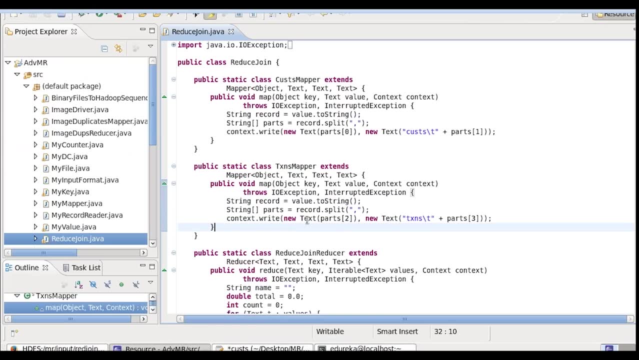 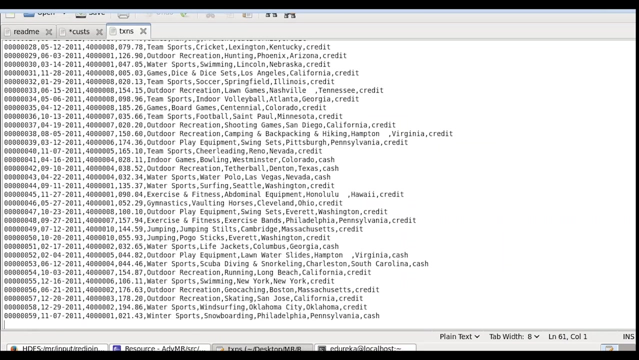 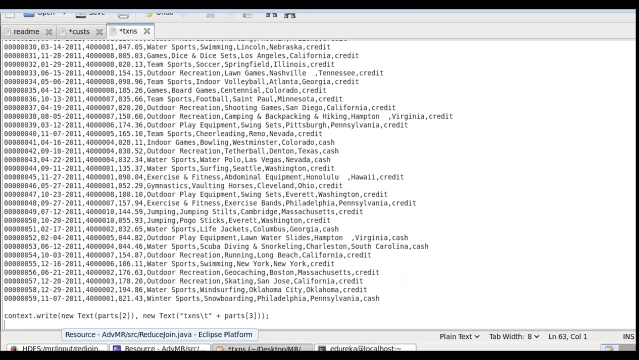 t christina, this is what i do, right, and in this, in this part, right, transactions, what do i do? similarly, i'm saying parts of two. just give me a minute, here you go for the transactions mapper. what i do, uh, this is the one. sure, this is what i write in the transaction mapper. parts of two is what friends here? 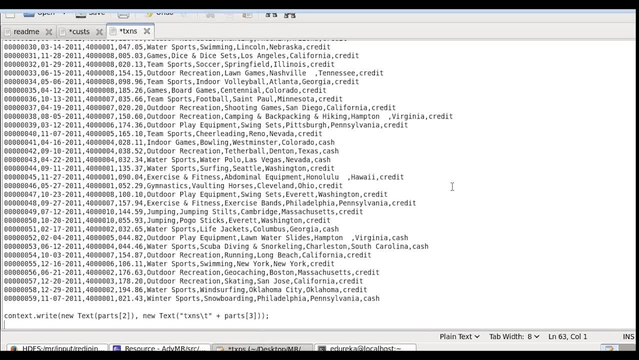 what is parts of two here? customer id, correct customer id. so it is four, zero, zero. whatever is going to come right, okay, okay, what is parts of? so i'm going to write something like this: right, transactions- again, i'm hard coding it here- and parts of three. what is parts of three here? 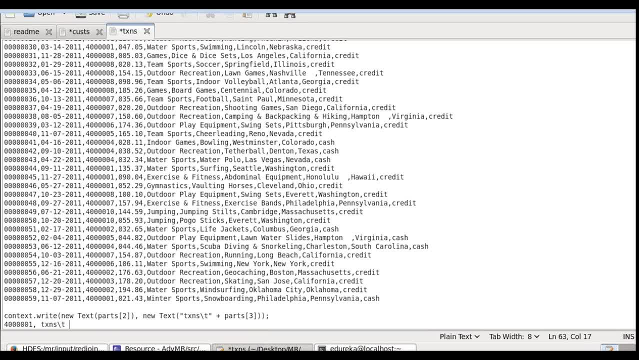 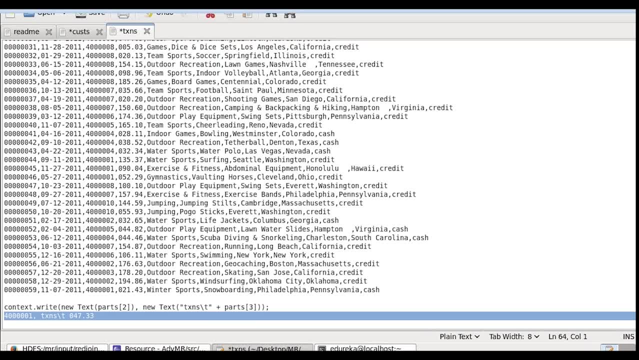 any guesses? the sale value right: 4733, whatever, right. okay, now how many times i should be writing for this? for all the transactions? right, all the transactions. i'm going to be writing this. then what happens? friends, i think you all may have basic idea about map produce. some of you may have correct, some of you have already done so, can you? 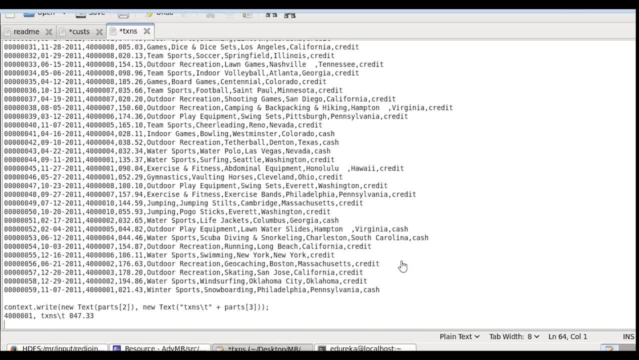 all try to answer. what happens after the mapper's output is generated? what happens, friends? what is the next step in the map? reduce, sort and shuffle. jagdish is you know, since he has attended that? right, excellent, sort and shuffle and sort, okay, sure, so what should happen? excellent, so, let us, let us make this for our interests, right so? 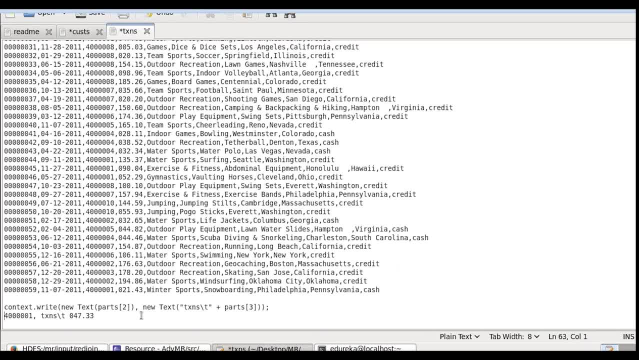 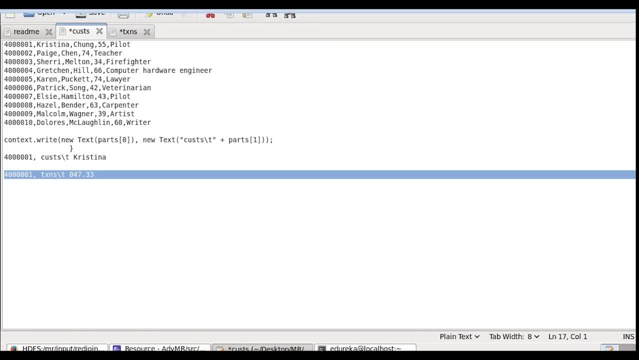 what should happen and then fed to the reducer, correct. so this one- you know what I am saying is it will come here, right. so this one will come multiple times, friends, because you know we have for the same customer. I may have 85. I'm just saying you know how many ever number we have. 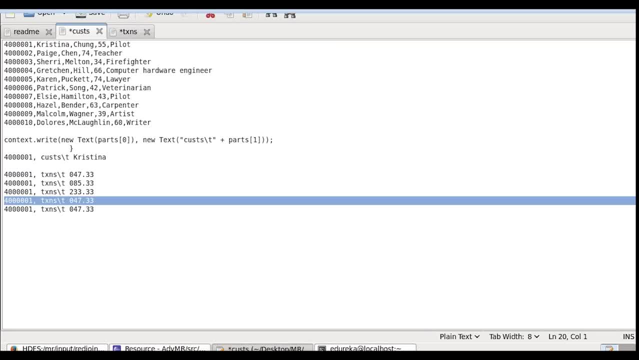 right, just throwing some numbers here. right, so it has three times, let's say fine, three transactions this customer has. so how will be the? how will be the values generated to the reducer as an input after sorting and shuffling? do you all agree with me on this? like it will create a list of values. 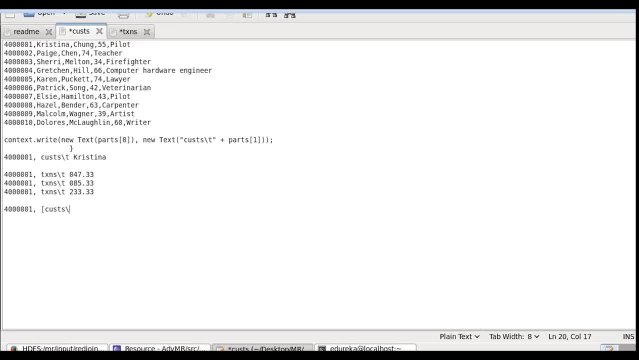 right, it will have something called cust t christina, and let's say I'm sorry. and similarly, transactions t, slash t 47, transactions t 85, and so on, so forth. right, 233, whatever, correct, this is what I will. is that fine, friends? this is what I will have. is that clear? 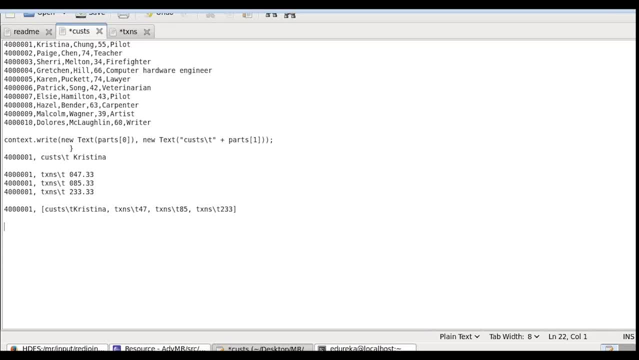 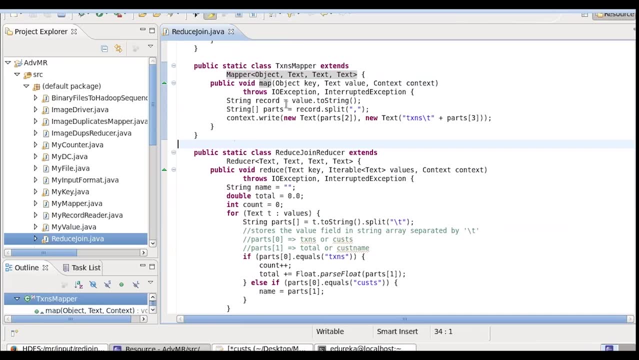 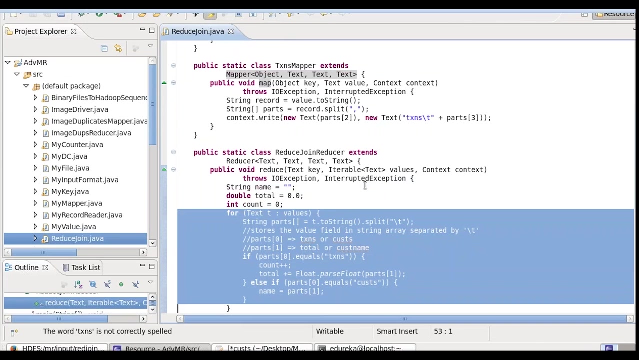 this is what expected to go to the reducer, correct, this is expected to go to the reducer. now I want to tell you, in this simple map reduce program, what I'm trying to do is- this is my logic- to find out the to print these total sale value as well as for every customer right, that's. 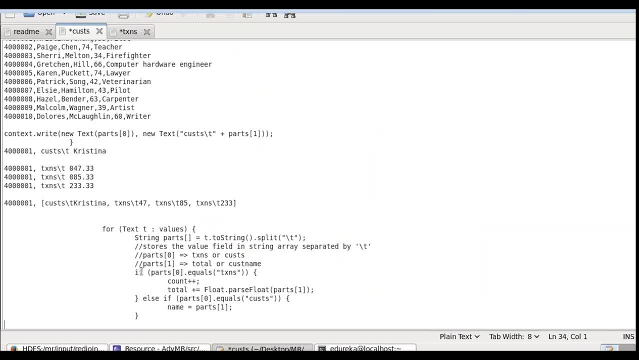 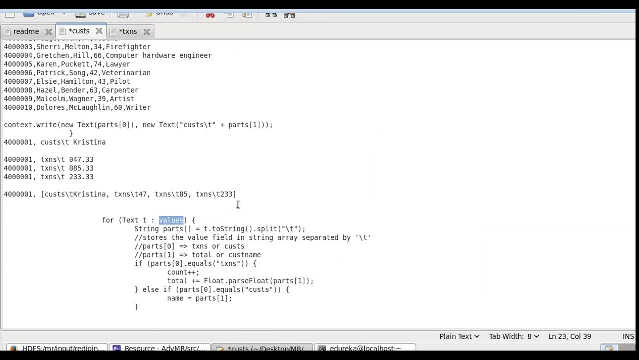 the idea what we are. I mean, that's the business problem we are trying to solve. so I will iterate on the values. so which one, friends, which one I should be iterating on here exactly when I say so? I will iterate on the values. so which one to? 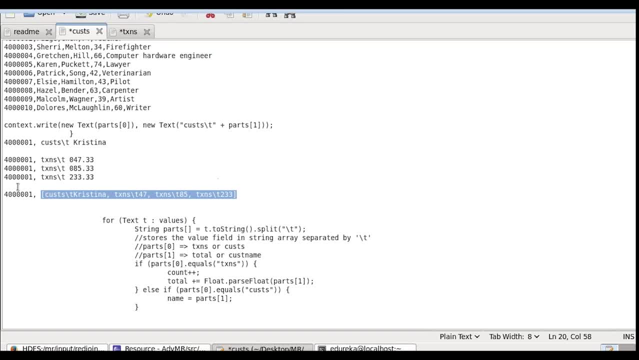 thefor. this is my value, right? this is my list, right. so this is my and not and this is the key after it is shuffled. this is my key and this is my value. this is how it is going to be fed to the reducer, correct? so I'm getting this, so I'm parsing this, so I'm saying, I'm saying: 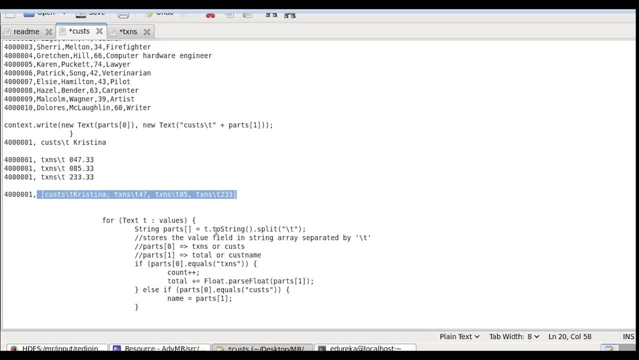 that I am getting this. so this is how I'm getting this. so I'm saying I'm again for each value, because I have hard-coded just to make a split right, because I'm going to split it on T, you know, tab, I could have put a comma also, you know, I'm just choosing to, you know. 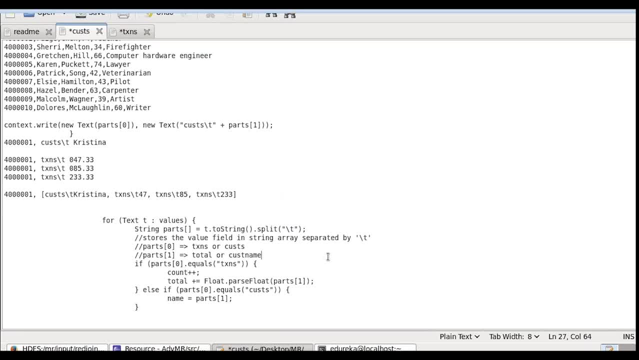 I'm using a delimiter. why I am doing that? because I want to identify or distinguish whether it is from the customer or the transactions. right, if it is a customer, if it is a transaction, I'm simply declaring a variable. you know, right above this. you know, if you see the code, I'm just having a. 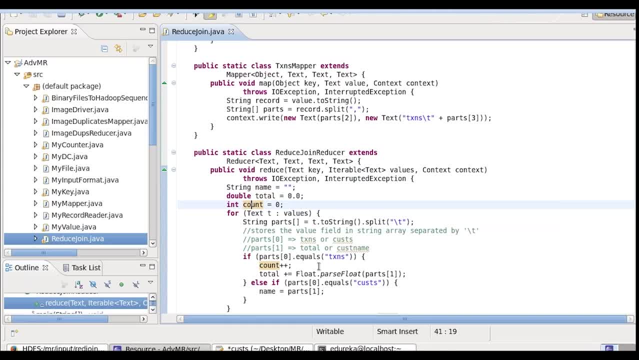 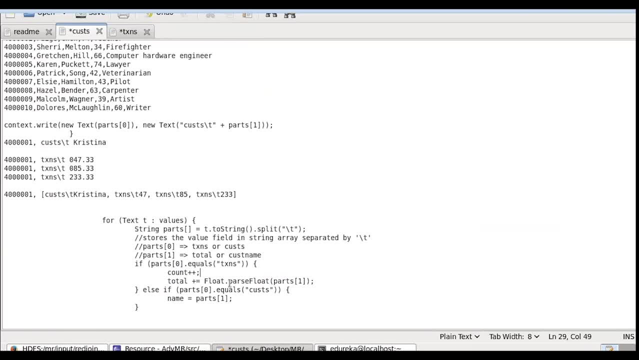 local variable here count right. so I am just incrementing the counter because I need to print the total number of transactions and I'm also totaling the parts of 1, which is my 47, 85 and all these things. can you all hear me, friends? okay, so this is my. 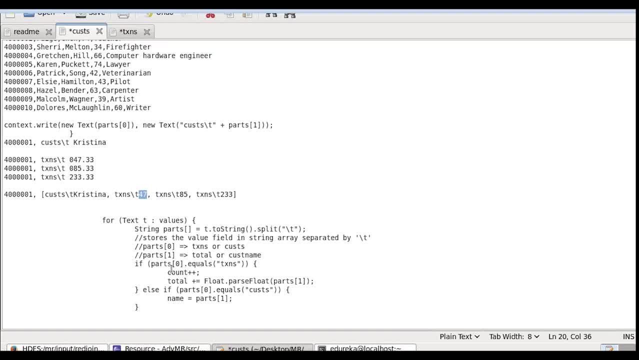 you. this is my, this is how I do the simple calculation here. if it is not equal to transactions, what is the other option, friends? what is the other option I will have? if it is not transactions, what is the other choice? the customer correct, so it has to be, it ought to be customer. if it is customer, the 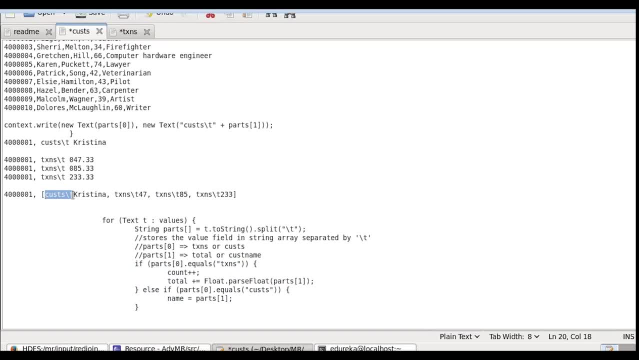 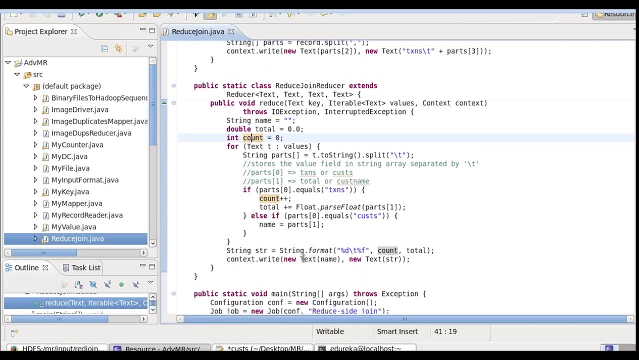 only thing I do is the parts of 1. this is the parts of 0, this is the after slash T, this is the 1, so I am simply assigning the name to my- you know again- a local variable. so what I do, I have to print the name, and so I'm printing the. 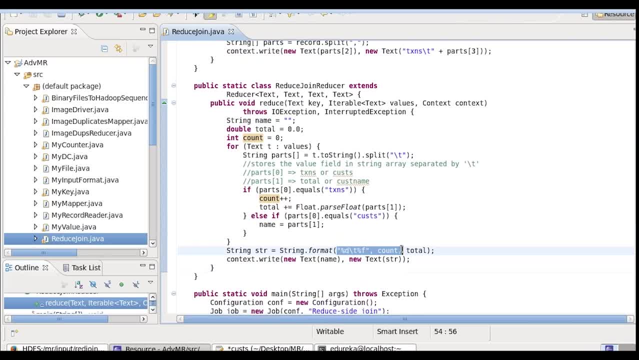 name as the key, the value as the count and the total. sure, are you all clear, friends? so I am meeting the objective of printing for every customer what is the total, you know what is the total number of transactions they are dealing with, and also, along with the total sale value, 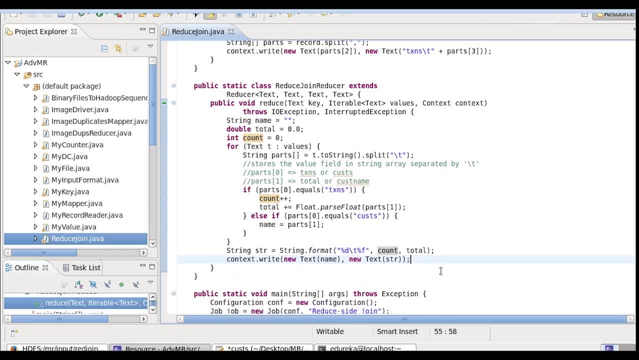 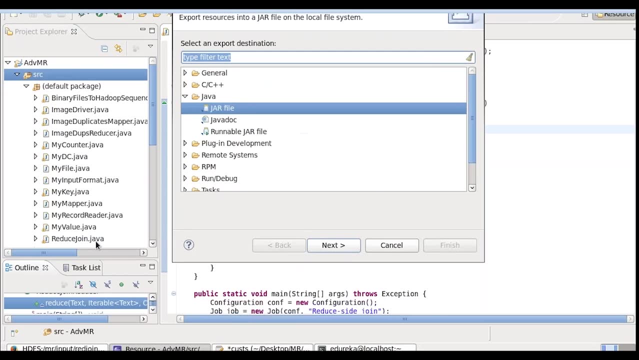 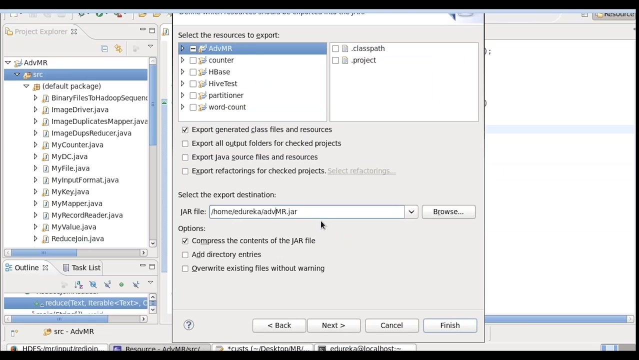 are you all clear, totally clear. okay, so shall we execute this and see just a simple file? right, let's execute this and see this just a second. I'm going to create a jar file, sure, and let me say, advanced ADV jar, sure, sure and sure and sure, and 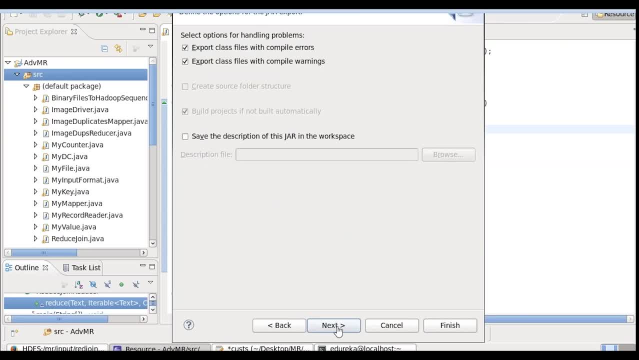 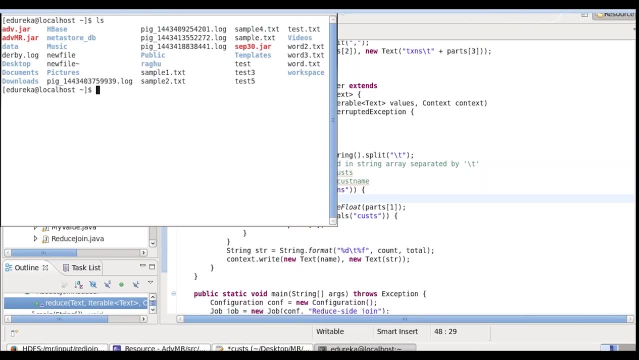 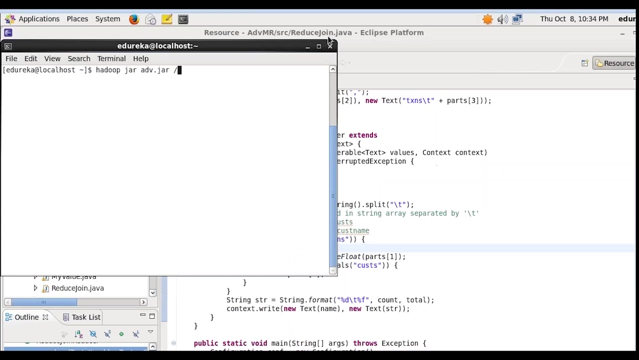 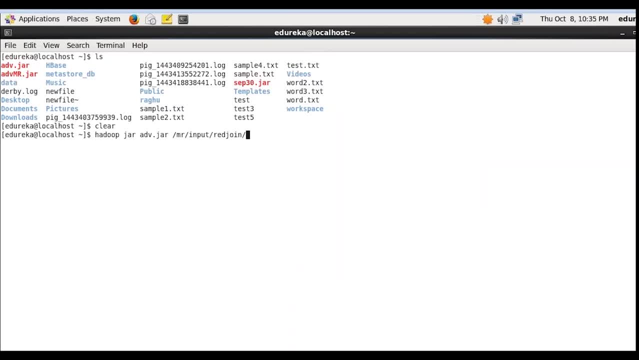 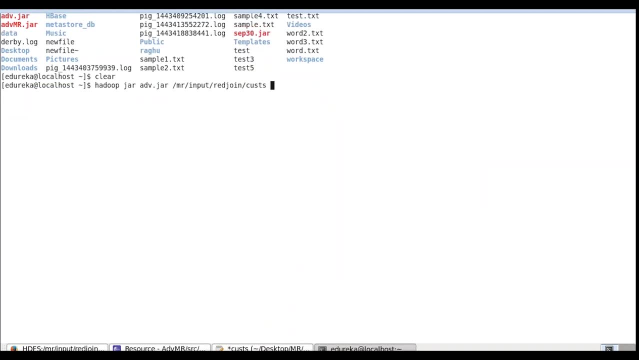 what is my input file inference? let me maximize this input file name. I have it in the HDFS Mar inputond, sure, and Here is my path. that's exactly what I give: Sure Custs, MR output. sorry, MR, Rejoin transactions, MR output. 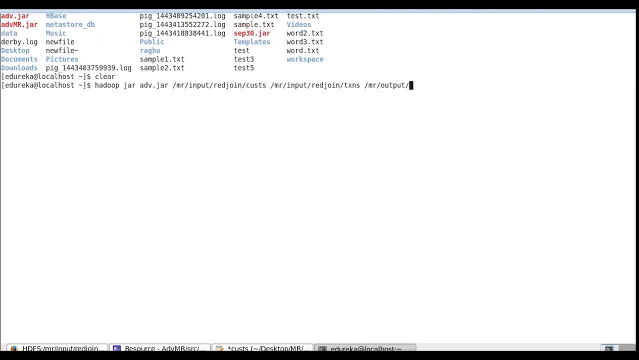 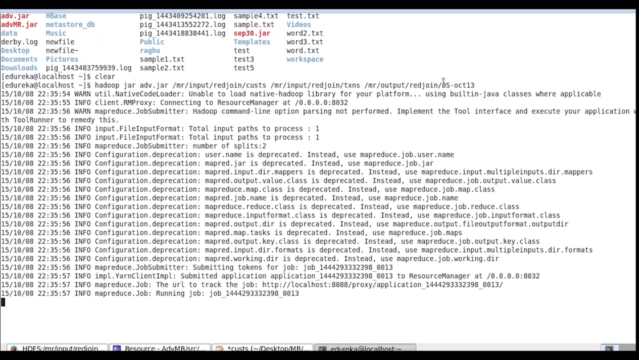 and let's say rejoin, and I say data science, right, Let me say DS, October. I just wanna create a folder, October 13th, Sure, Let's try this. So this is where this is the location in which I want to generate the output. 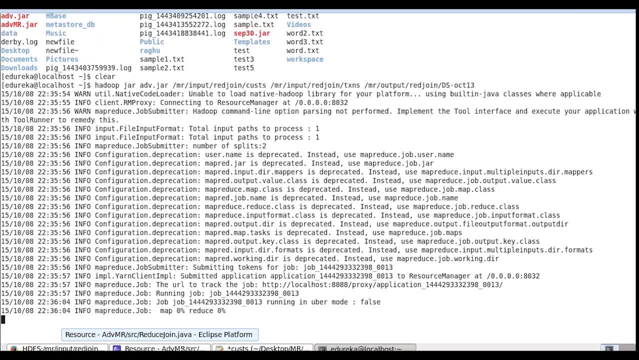 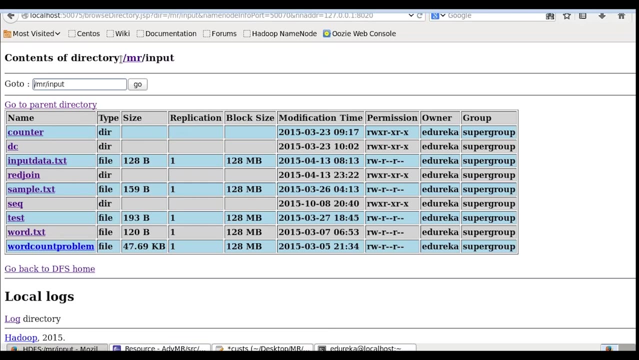 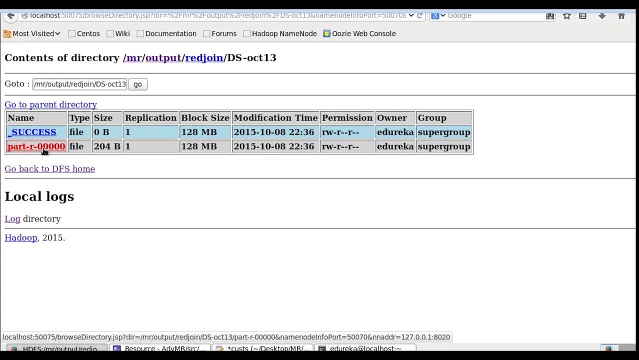 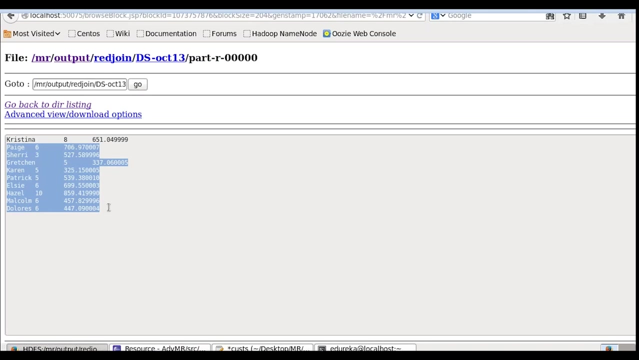 Sure, That's exactly where I'm coming to Done, So I go to the MR MR output. this is where I generated the file. you can see Christina had eight transactions, total sale value Similarly so many other 10 customers. 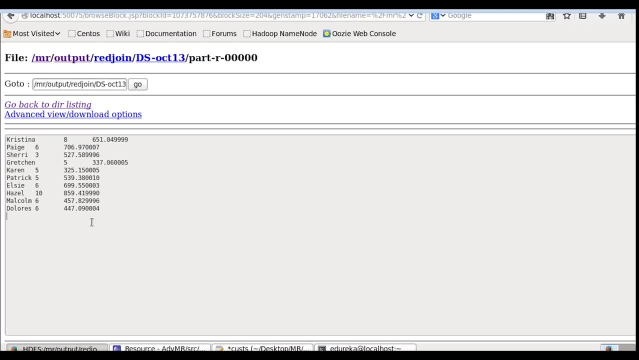 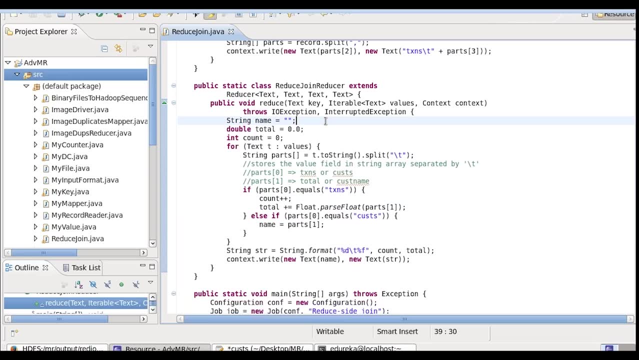 they are all having transactions right. So, okay, the relevance is the data scientist. as I told you, friends, they should know, as a data scientist, they are very scientific, as I told you, they fix the algorithm, they optimize it and all that. they also need to know what kind of solution they have to use in. 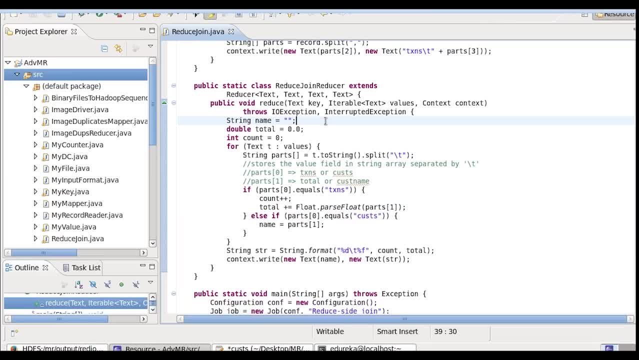 different scenarios, right? so this is a simple one. what I showed you, which is using Hadoop, right, because the, the storage is Hadoop and you know I'm just doing a simple processing in Hadoop. so the data scientist also. they try to use various algorithms, where to use what and all that they need to know, correct. so 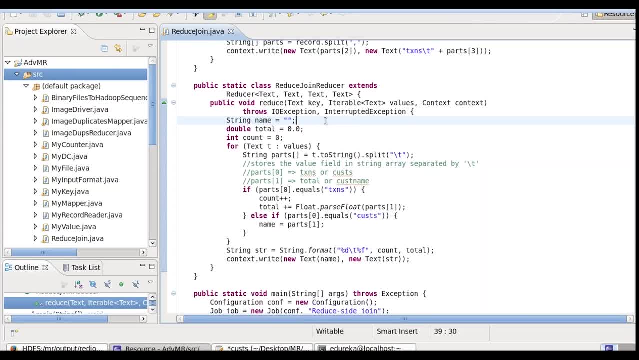 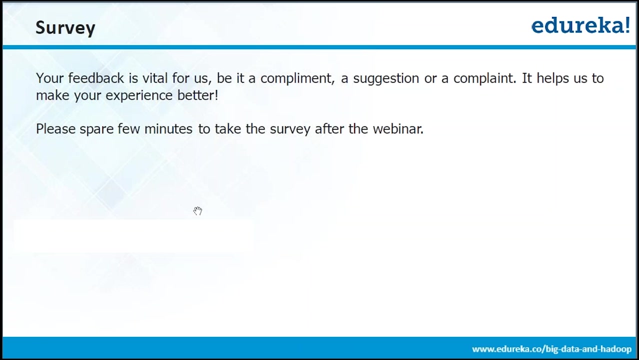 that in order to analyze or or even cleaning up- right they may you speak to do a data transformation, because pig is a effective cleaning up tool. you know it's a transformation tool, the various ways to look at this. so, friends, I'll go back to the deck. I think I kind of you know, just so, as I told you, you know your. 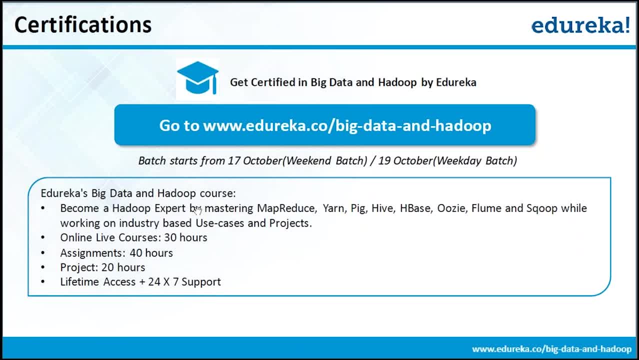 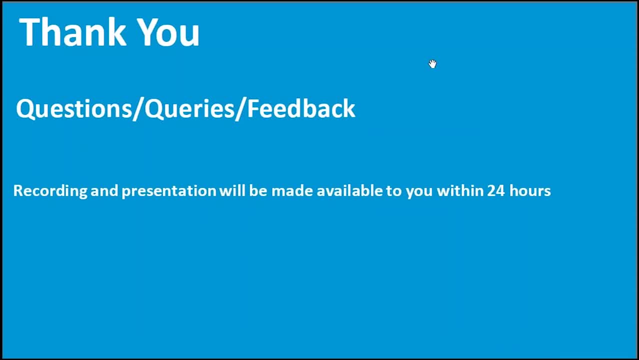 feedback is going to be super important and you have the certifications and you have this batch starting up pretty soon and you know, as some of you asked, I have done big data from Hedera and you know it is absolutely. you know data science, you know pretty vast and you know there's a lot of useful topics. I mean it's, it's a 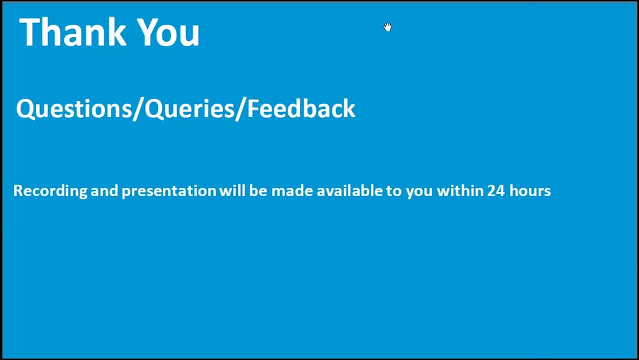 very expansive course again and you can check with a director. you know what is the course, criteria and all that. you can check on that. but now let me take up a few questions. we are- we are just at 10 o'clock. okay, now I'll take up questions for the next 10. 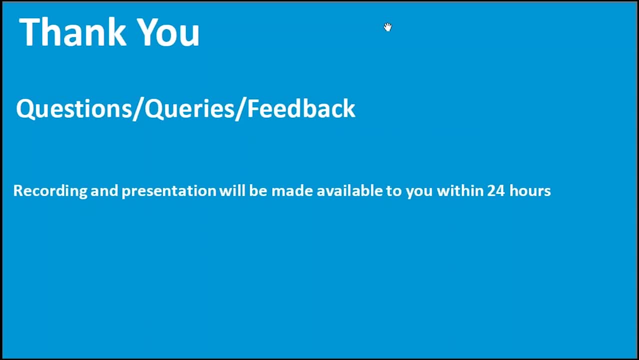 minutes, friends, so that we can end it on, you know, maybe 10 minutes from now max. how do they use various algorithm? in MapReduce or in the result of MapReduce? so MapReduce is a processing framework of each other. it's part of how to. when I 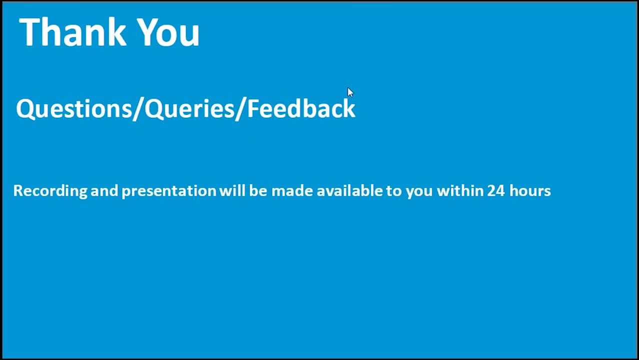 say algorithm: right, you can use different algorithms to use. you know, first of all, pig also uses MapReduce, right. hive also use user map MapReduce. in certain cases you really want to use pig or hive or the raw Java MapReduce because if the data is highly unstructured you may still want to use Java right. 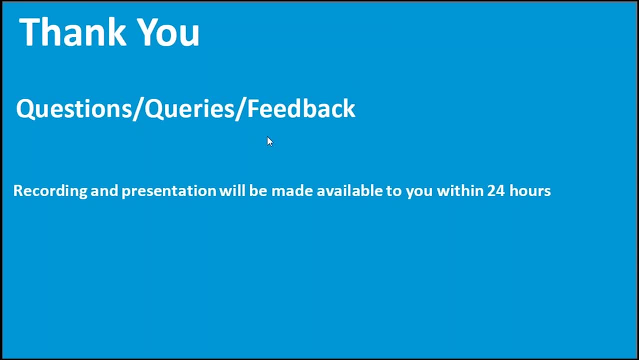 because Java has fantastic libraries and all that to handle various kinds of data the course contents. so many of you are talking about data science. I think Edureka is the best guys to answer this. but you know, I can tell you they definitely cover some of the data science and 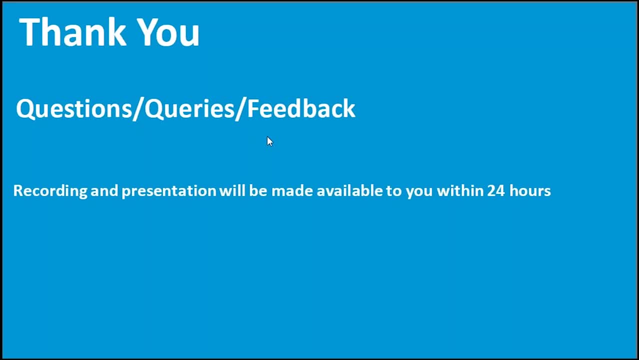 basics and they go in-depth into business analytics, they go in-depth into R and all those things and they also try to cover the Hadoop friend on few things. and you know, and you also will be talking about the big, the mahout and all that. so it's. 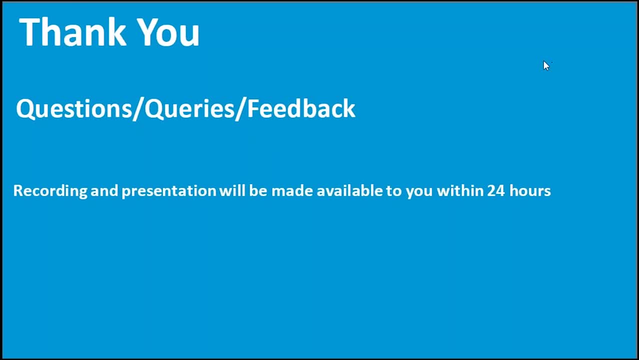 quite an expansive coverage there, right? so I am looking at the question window, friends, one by one. can we use Kafka as an input system? which is better? which is better, Kafka or Spark? both are different. Anand, right, Kafka it is to pro. it's like a you know rabbit MQ kind of thing, right, it can. 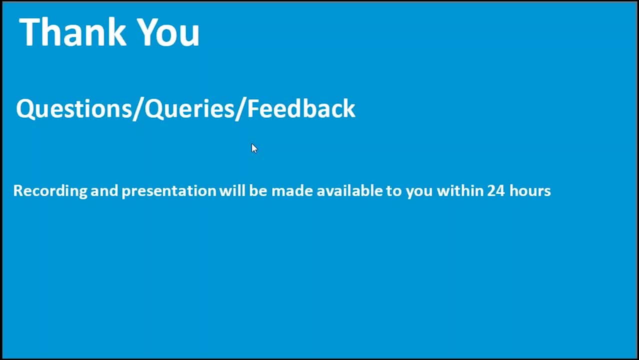 process messages right in an asynchronous way, whereas spark is more a batch processing but it does it in memory. spark streaming is real-time processing. for data science, do we need to have complete business knowledge of underlying data motion? I think data scientist is more towards technology. I think people you know. thanks for asking this question, but 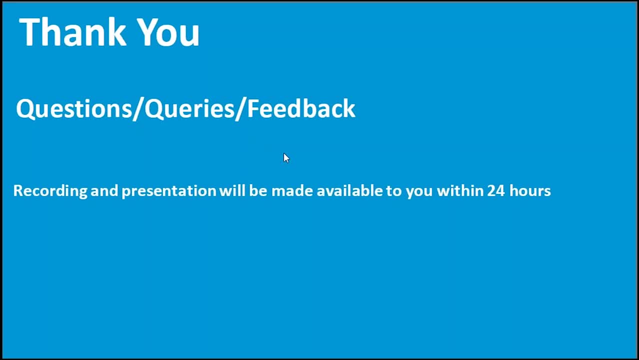 I think they know how to do so. so not getting taxed. branching out first question: because business analytics: they see there is a subtle difference, right, data scientists, they fixed algorithms, the optimized algorithms, right, much better business analysts: they need to know which algorithm to use or for a business domainr. 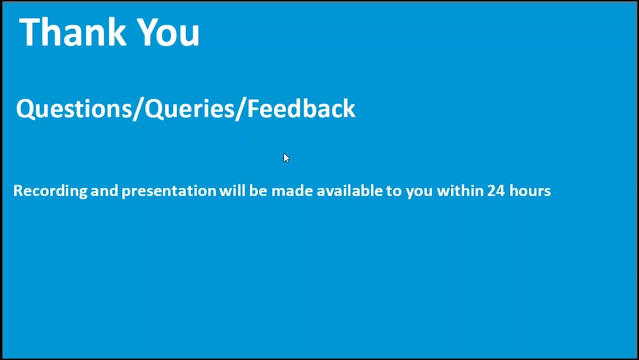 or for a business problem, because these guys are also masters in the business domain, right? so that's a subtle difference, but they work hand-in-hand correct. and data scientists also. you know they have a good knowledge- simple section of Movingron knowledge on some of the domains, but it need not be the case. so the business knowledge: 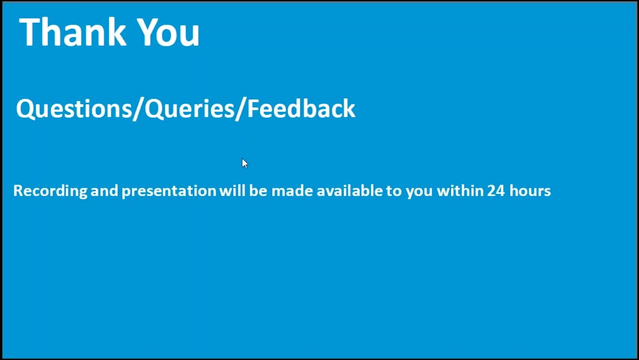 I would say more a business analyst kind of thing. data scientists are more scientific in nature. push up right, more scientific. they are good in- you know- scripting. they are good in machine language. they are good in Hadoop. they are good in technology. they know. they are good in my. you know some of the algorithms and all that. so that is the spark storm and 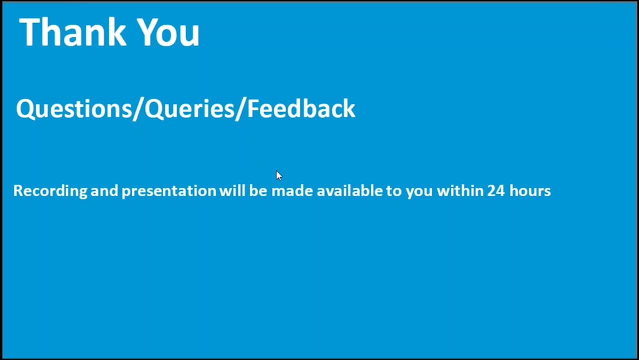 Hadoop, basic difference. so spark, as I told you, Shreyas, it is more a in-memory computing. spark streaming is very close to storm. I think spark runs on, you know, Hadoop. again, right runs on Hadoop whereas storm runs on mesos- I could be right or wrong here- and Hadoop as it said. 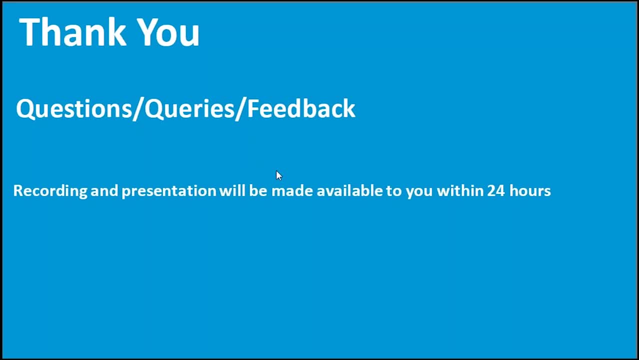 right, it is batch processing, correct. it is primarily for high latency queries. will recording be available For other course takers? this recording should be available. Arun Kumar I. you want to check with the Endureka support, but I guess this session is being recorded. how much execution? 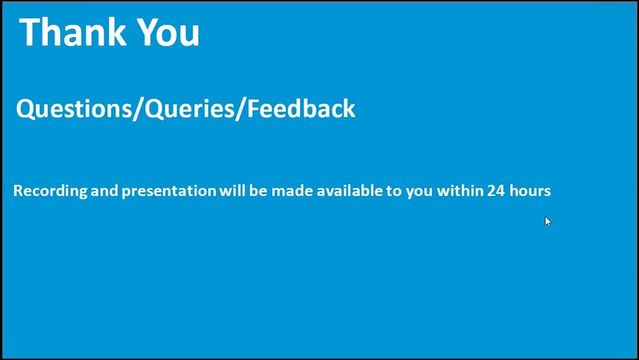 time would it take a value? need to be updated? okay, Updated in all thousands of tables, 1.5 terabyte of Oracle DB. Taniru, the point is, you know, if you are talking about Oracle DB, right, what I can do if you want to, if you have such a. 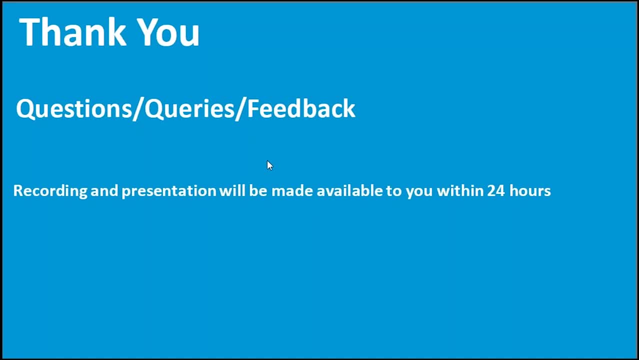 massive data. I can scoop the data. I can use, scoop to bring it on to you know, something like a hive data store, right, and I can do, and I can get the values updated. that is possible right at 1.5 terabytes is not a, you know, it's not a big data as such. right, maybe for Oracle. 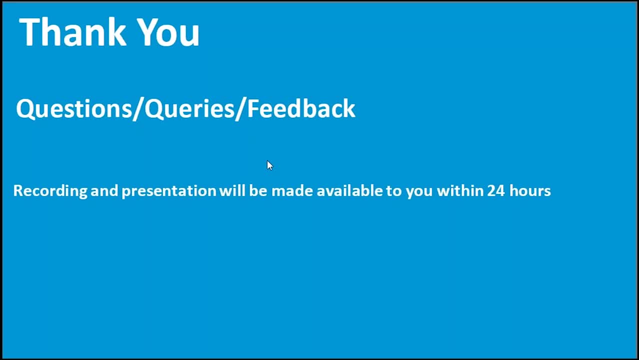 yes, but for hive it can take, You know, because any data that is coming from Oracle, right, it's structured data, so I should quickly get it on to hive, right, then I can probably update it and send it back to Oracle. so that's one way of looking at it. but if you're going to use hive as the 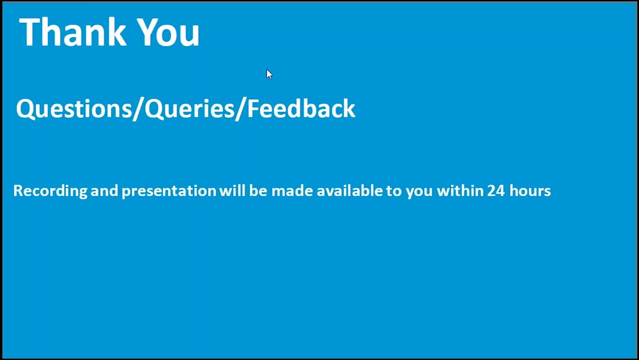 data store subsequently, then I can very well keep that in hive itself. when you say how much time, it should not take much time and you know it should be in. if you properly you know Thousands of tables, I don't think it's going to take much time. I'm not exactly, you know. 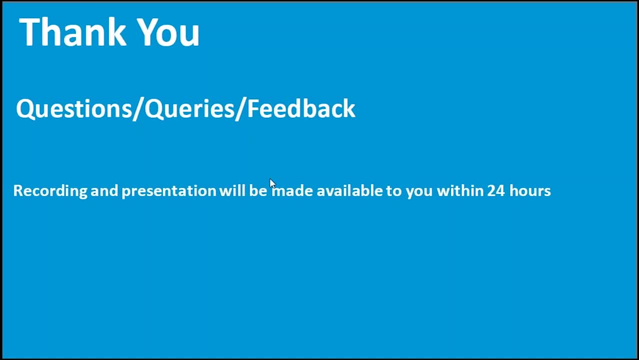 because it depends on various parameters. Taniru, I cannot say it will take milliseconds, but should take few seconds. that's all right. why is both HBase and HDFS are required? is it either or optional? it depends, Sajit, it is like HBase. I'm not saying it's required, I'm. 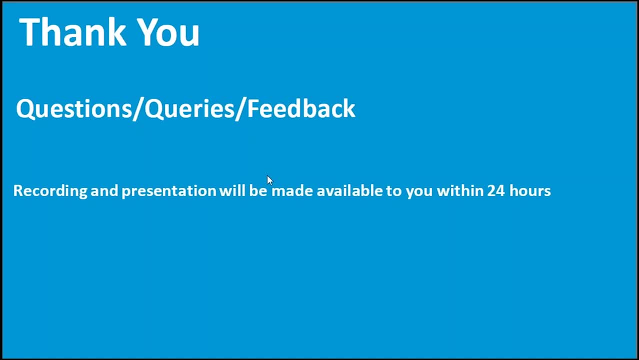 not saying HDFS is also required in certain cases. if you want to use low latency queries, go for HBase. if latency is not an issue, go for HDFS. right, HDFS is a pure file store. you have any other language instead of Java apps? absolutely, Pankaj. you have, Python, you have. 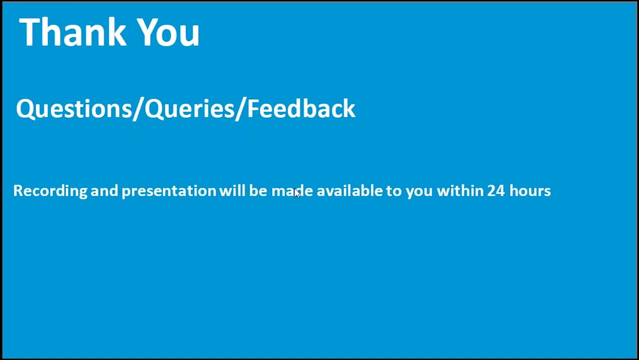 big. you have all these things are there, right, hive and everything. sure, hive is a data warehouse system, data warehouse tool. It's one of the Yeah Ecosystem tool provided by Hadoop Mohamad. where is HBase used in your demo? I didn't. 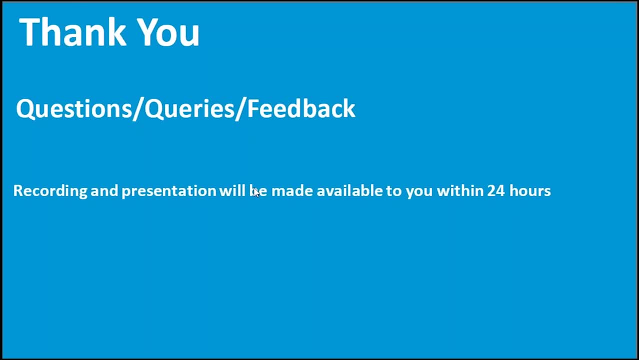 use it? Sajit right, I didn't use it at all working as a support project tableau administrator. career change to big data analytics with one year with cloud era? yeah, it's a tough question, right, Kishore? it is see, it all depends on everybody's ability also, so it is like yes. 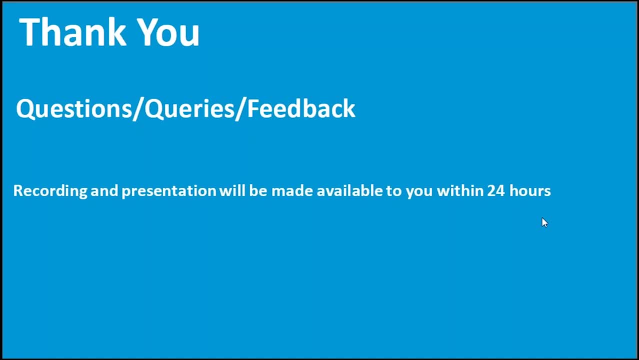 I mean You know positives note. I can tell you can definitely make a shift, because I would say, Kishore, because you are a tableau guy, right, you should be good in visualization. I I feel so maybe you can look at how you can marry, even tableau can connect to Hadoop. maybe you 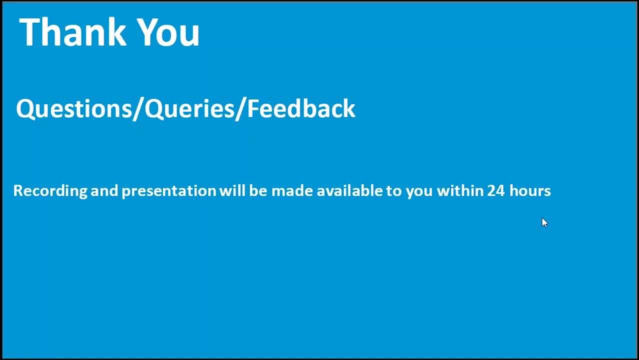 can look at that kind of portion right and how you can bring the analytics overall. you can learn that analytics and how you can bring the analytics all the way to visualization. that is one area you can explore, Kishore. Okay, Just as a thought. Hafiz is asking: is it similar to SQL? hi, absolutely, it uses MySQL dialect. 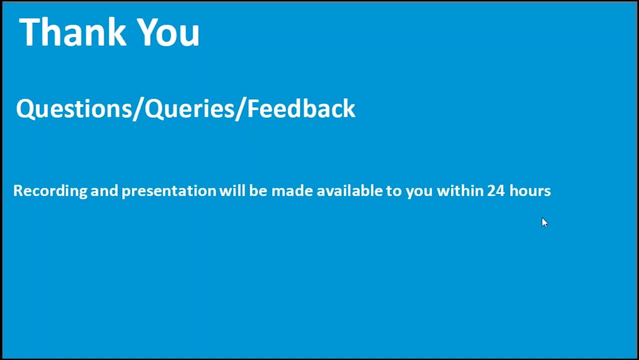 Hafizullah, yeah, when we decide to move to Hadoop, when PhD masters in statistics required for data scientists, that is one way, tamachari, right, it is not a mandate, though there are folks who can also, but you know, generally people come up with such kind of degrees and 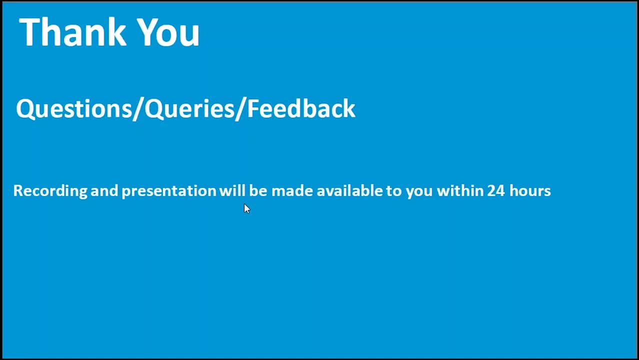 all, quite a lot of people, right, But I would say you know somebody who has an aptitude for math and algorithms and all that- they are fairly good candidates to get into a- can be groomed as a data scientist. we can use MapReduce for data, then what is the need of NoSQL DB like MongoDB? okay, that's. 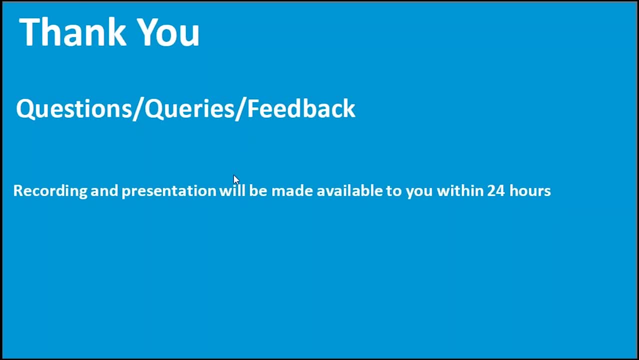 something different. right data processing is that is, processing the data. correct. MongoDB is a storage right. it's a data store. both are different. Storage is different. Storage is different. Process is processing is different. correct any programs other than. is there any other programs other than word count? why do you ask that, Malika? there are millions of programs. 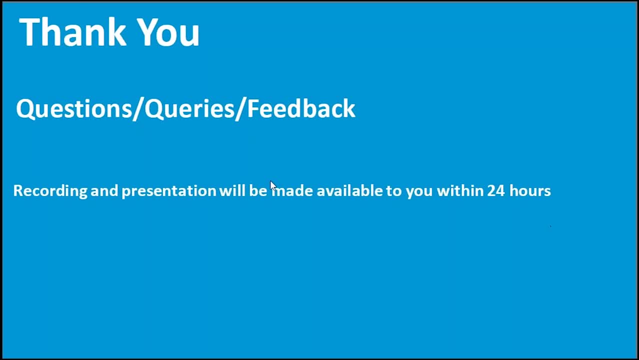 so many programs are there for a person better in programming? what extent do you think statistical knowledge is required? I'm dumb in math, okay. so, friends, I think there is a interesting anecdote or something which I saw very recently In a data science thing. right so a data scientist Jagdish, you know, you don't need to be discouraged. 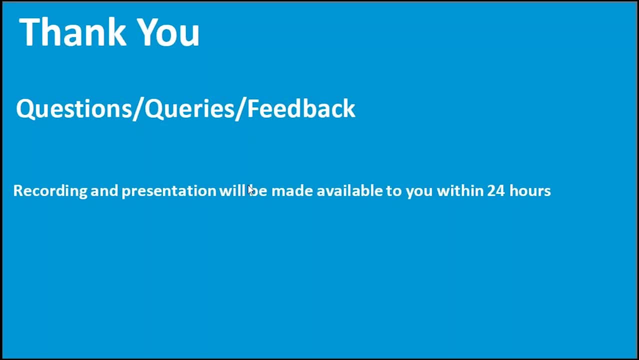 at all. right, my point is: a data scientist is generally knows you know more statistics than a software programmer or engineer would know, right, and he will know more software engineering practices than a statistician raw statistician will know, correct. so they know they have a combination of these two skill sets. right, they have a combination. 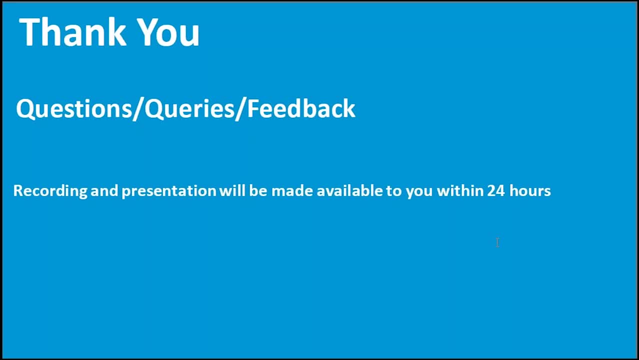 of these two skill sets. so they are generally good in math, they have a good analytic aptitude and they are good in stats, so that you know they can understand all those stat, complex functions, algorithms, regression and all that stuff. right so? but you know it is, it is not. 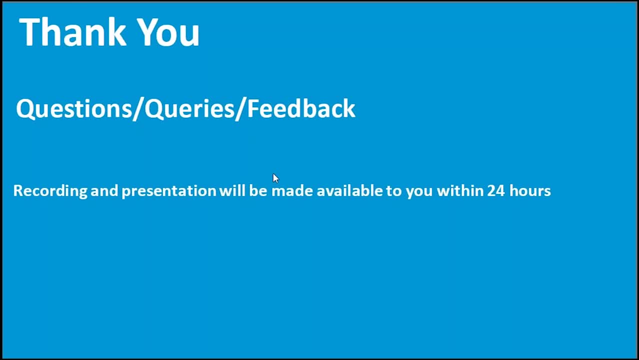 a skill which is impossible. you know it cannot be picked up or anything, sure? so you know it, you can learn it, you can always invest on that difference between MongoDB and Hadoop. yeah, in fact, MongoDB is a NoSQL again around. how dope is a file store, right? MongoDB doesn't. 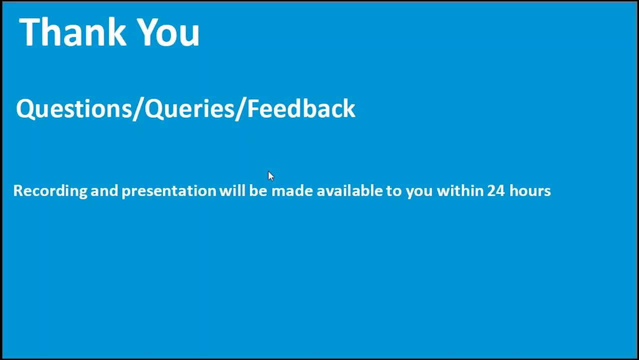 need to be on Hadoop in the first place, whereas HBase needs to be on Hadoop. MongoDB is a NoSQL database, correct NoSQL database- where it can store data. how do can also store data. but MongoDB and all these NoSQL databases- right, it is primal. it is fundamentally different. 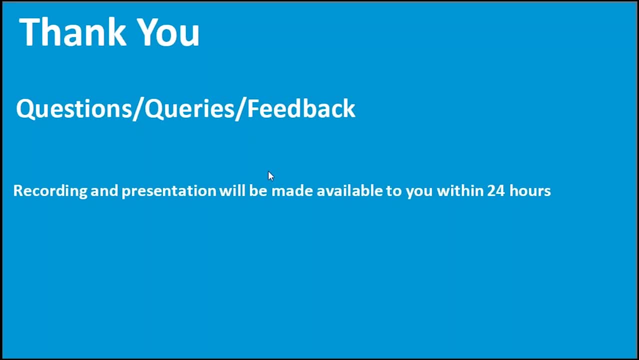 from Hadoop, Hadoop or the Hadoop file system in the retrieval process: right, the random retrieval: correct. So those things Hadoop doesn't support. as I told you. right, It comes up with high latency. So any real time data you want to work on, right. 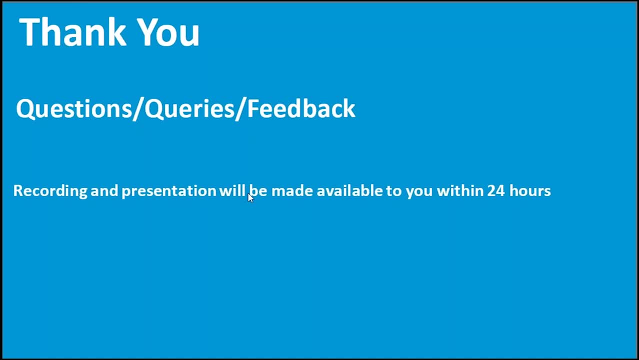 These databases makes it possible? I need some real time projects. Is it possible for real time projects? There are lots and lots of projects, Mallika, So maybe you can check with the Edureka support. I'm not trying to, you know, make any marketing pitch here. 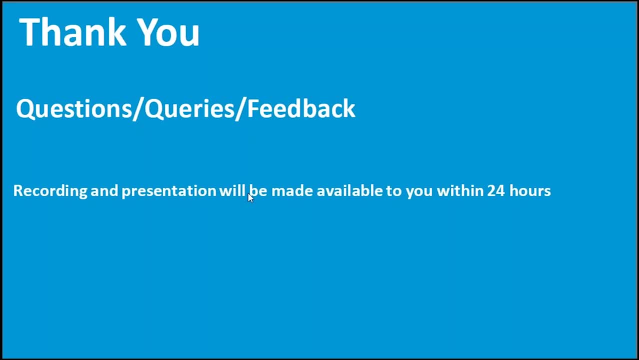 but you know, there are lots of you know, and for you to take a quick outlook, right, You can always go to. you know, Hadoop, powered by Hadoop, and all that. right, There are lots and lots of companies they are doing. 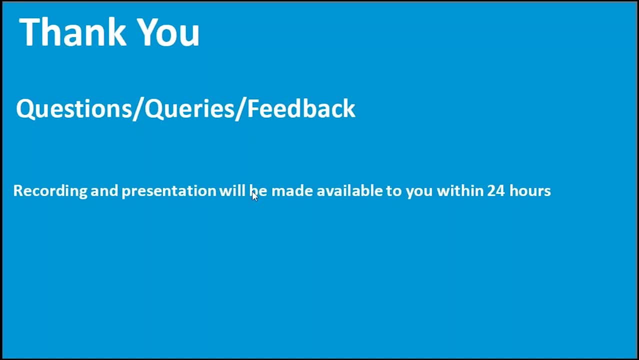 real time projects on Hadoop. Most of them are using Hadoop clusters, Store the data in file format and process. Sure, Abdul, it's possible. What is Hive? I think I answered you, Hafizullah. Is it similar to SQL? 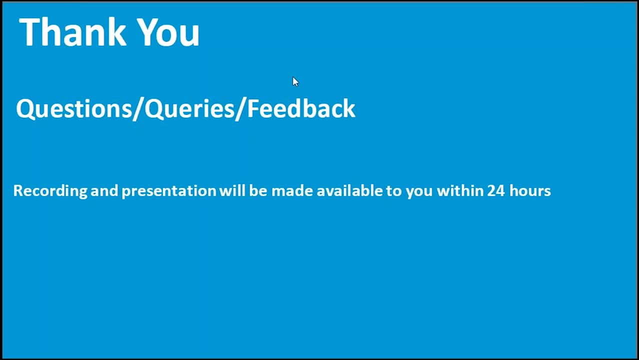 I think I think I'm again. this was answered. What language do they use for MapReduce? Java, PIC, Scala, real time projects? I think anything can be used. Java can be used, PIC can be used, Scala can be used and Python can be used. 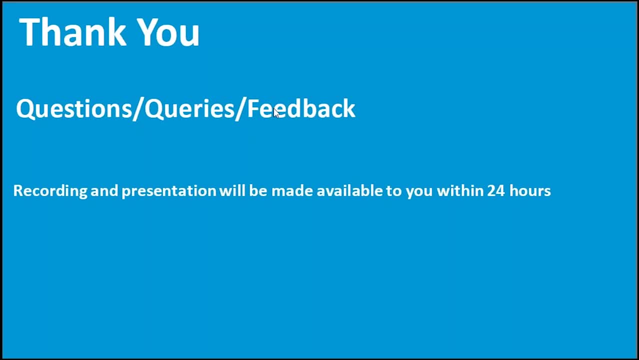 Can you look into Hive as a career in big data? Absolutely, Hafizullah, it's possible. Yeah, in fact, I come from C++ background and you know I understand Java, but I but there are simpler ones. 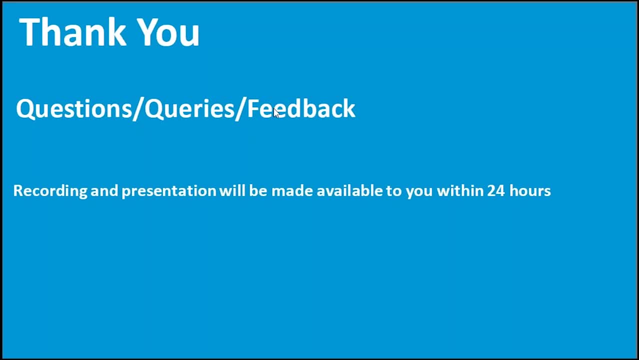 so I always try to use the simple ones correct. Whenever you can use that, okay, Why use HDFS, why not? I think I've answered this Hadoop: compatible with R Yes? the answer is R yes, Python. I think somebody told me right. I think one of you asked PIDOOP or something Which one has an advantage. So I would say R has got connectivity with Hadoop. I'm sure Python also has. I'm not, Though I haven't used it. I've used R with Hadoop. 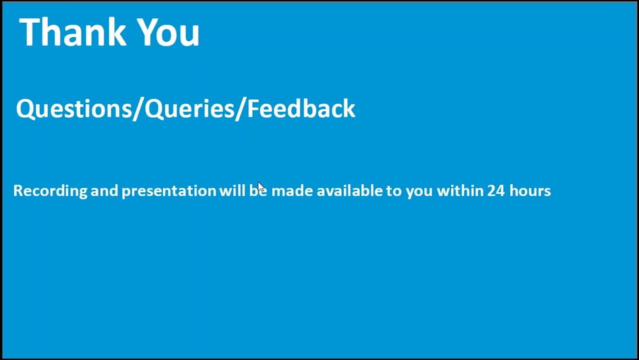 How important is RAM memory for running MapReduce? Should it be proportional to data sets? I think RAM memory, I think whatever we have right, a typical Hadoop commodity server generally if it has, like a, you know, 8 GB. you know this is what we are talking about, right? 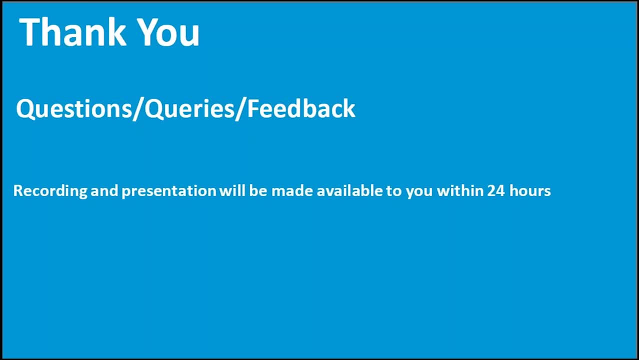 8 GB kind of thing we are talking about. So a fairly good commodity server can do the job, sure. So it depends. you know how important RAM memory I'm not. we are not really looking at a very sophisticated machine. 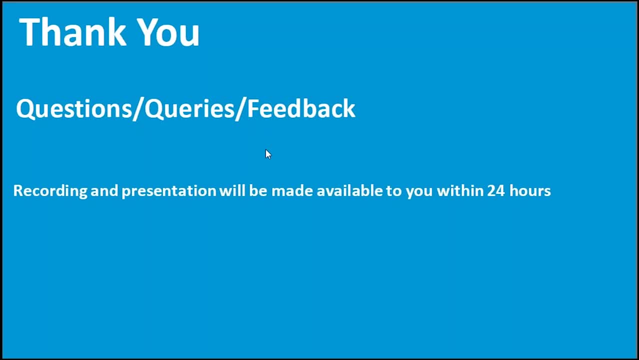 But it is. We are not looking at a very cheapo hardware. also, We are not looking at a throwaway machine. you know which. you can use it for Hadoop cluster. We have a reasonable, good terminal server Which is also very cost effective. 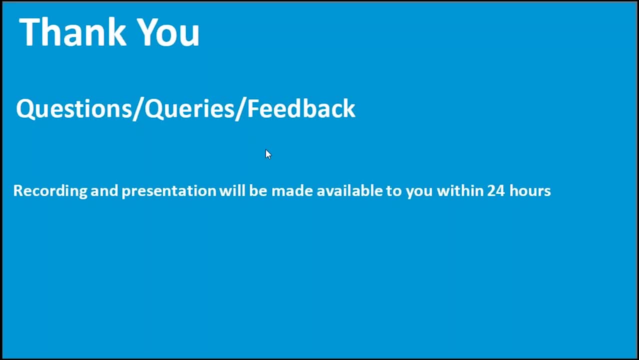 Punkerge eight years in Oracle. can I switch? Definitely Punkerge, it's not a you know. Anytime you can switch because people are moving into big data. people are moving into analysis, analytics. Wherever there is data, you'll have analytics. 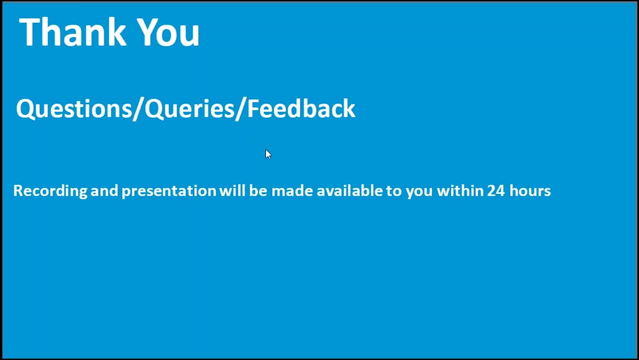 and wherever analytics and people are gearing up to IOD and all that stuff. it's all cloud big data. These things are going to be the future for sure. Data brought to the memory at the time of processing Ajit. it's a long story short. 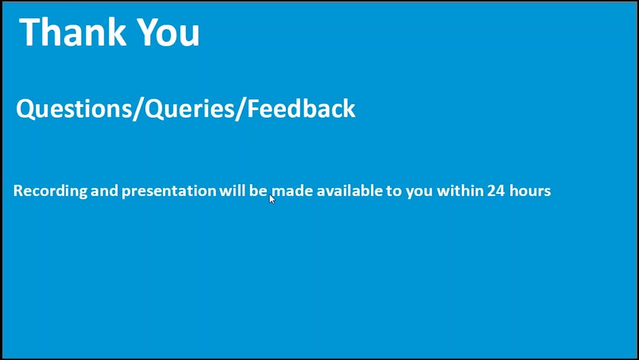 The data is not brought. The program is taken to the data right. Yet he can project. he can get project use cases from Edureka support. Jagdish said: Okay, sure Jagdish. yeah, I'm not okay. I think I've answered this. 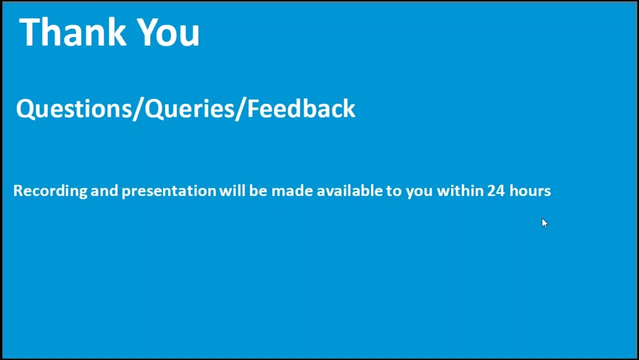 I can use complex transaction. I know it's a dumb question, but I knew how long would take Hadoop to implement the level from scratch. It's not a dumb question at all, Shreyas. I think it takes anywhere between. Just if you can take a course right. 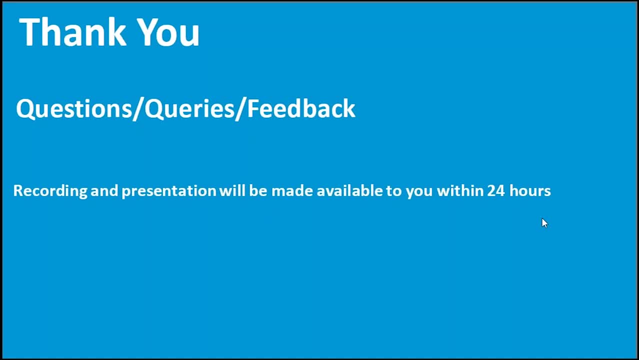 It need not be anywhere. I mean, you can just take it at your own, whichever course you want to take. right, Make an effort to do Hadoop. yeah, that's all. Just make an effort to read Hadoop and understand the basics. 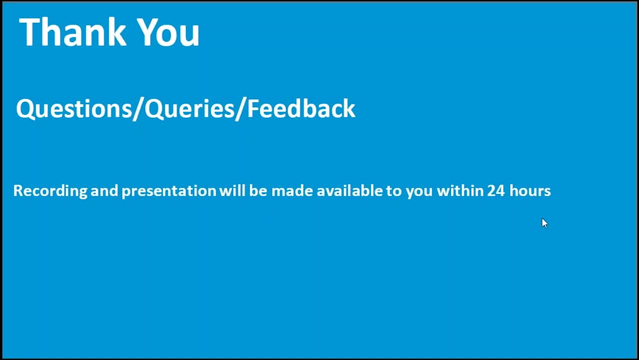 in how things are implemented and where all they are implementing and what are all the fundamental advantages. all these things you need to understand. So it takes for you to have a good grip on Hadoop right Anywhere between three to six months. 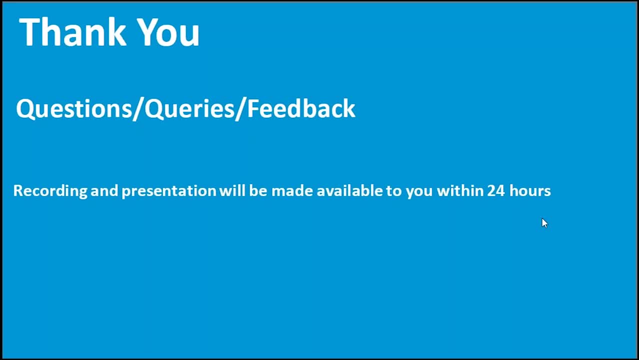 you know, just to get a a good grip, because you need to at least have a couple of implementations for you to claim that you know you're good. correct Average salary data scientists. it depends, Jagannath. I wish I knew this, but you know, but they are. 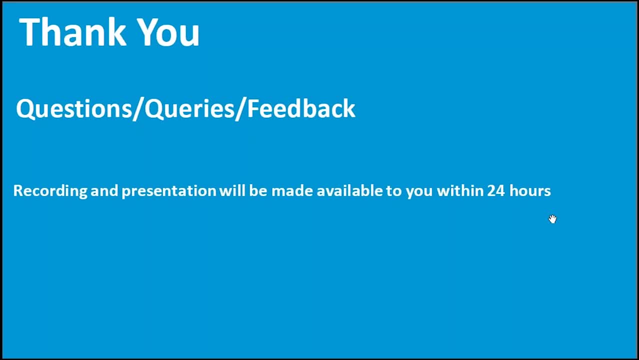 it is considered one of the sexiest job of the 21st century, which is a. you know, everybody says this, but you know, but it's really true, People are, you know, really moving in this direction. So I think people are highly paid in this area, sure, 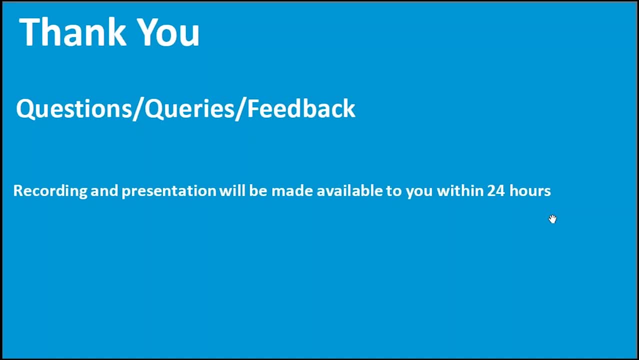 Okay, necessity, yes. You didn't answer the question yet, Khalid. yes or no? No. the necessity, yes, Khalid, It is. you know if you are, because we are talking about data preparation, we are talking about data transformation. 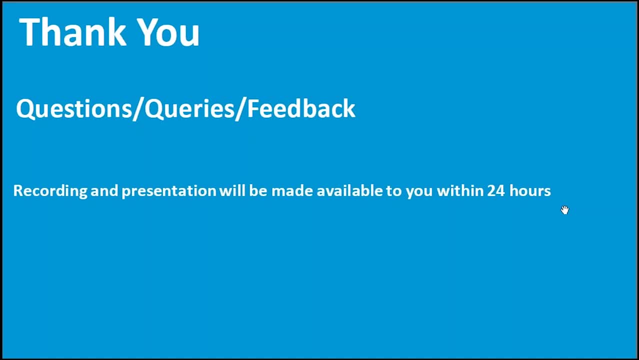 we are looking at data cleansing, all these things right. Hadoop is one of the platforms that can provide seamless integration for all these things, So I feel that you know it's one of the one of the- you know, favored platform. 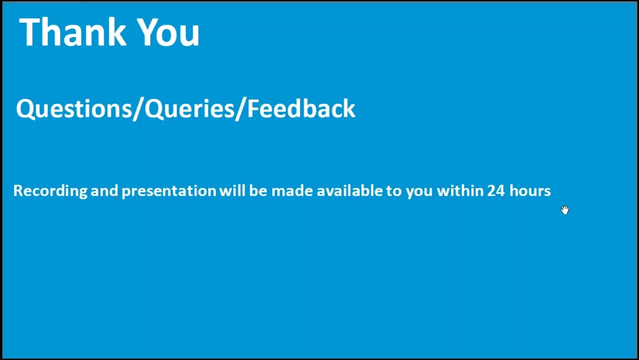 platforms for data scientists as well. Sure, Spark is going to replace. what do you think Krish is asking? In fact, Spark. yeah, as I told you right, Krish, Spark is not going to replace as such, Spark is going to complement it. 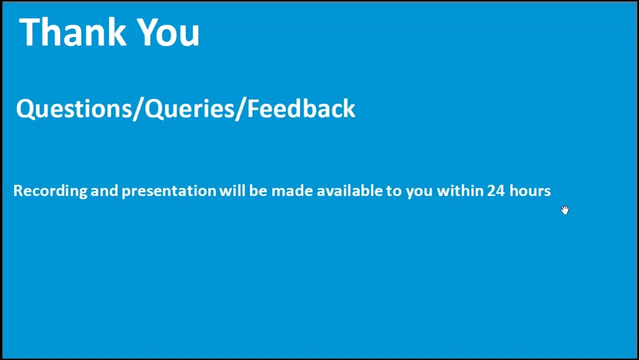 You know, friends, as I told you right, it is like you're not. I mean, a lot of people ask: RDBMS is dying. yes, it is waning, but it's not going to die. If I can use RDBMS for you know, for certain solutions. 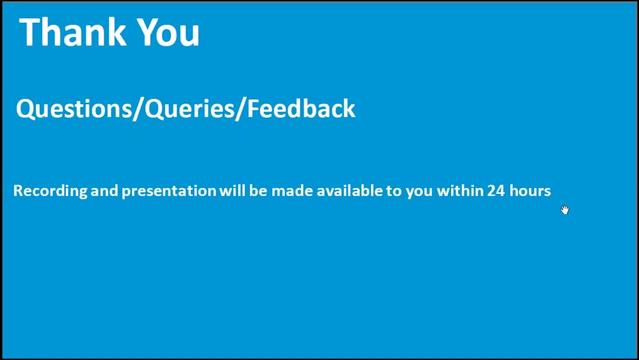 right, which the data is never going to grow, but I'm going to have extensive querying. I would rather go stick to RDBMS, right, I can use, you know, maybe SQLite or MySQL wherever possible. right, And for real-time queries, I can use, you know. 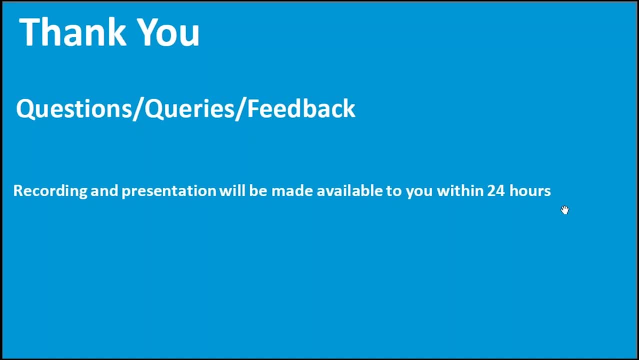 any streaming data, I can use Spark streaming or Storm. And for real-time queries, I can use Spark streaming or Storm. And for real-time queries, I can use Spark streaming or Storm. And for real-time queries, I can use Spark streaming or Storm. 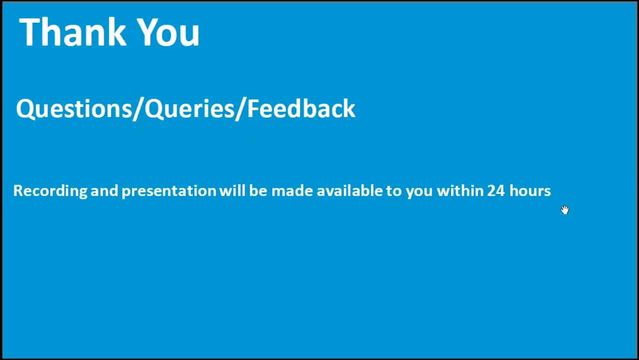 And for data which is like you know I you know, latency is not an issue which I can get it done in minutes. right, I can park that in Hadoop or one of the you know NoSQL databases. there's lots and lots of solutions. 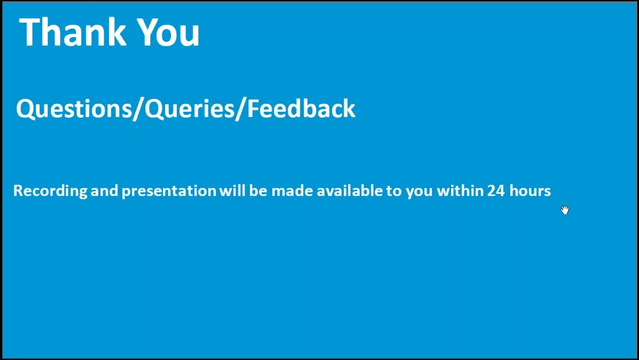 People are looking at not single solution, right? So they are not looking at single data source. They are looking at an assorted solution, because you may have five, six business scenarios within your organization. for each scenario you may have a solution. So they want to just put that together. 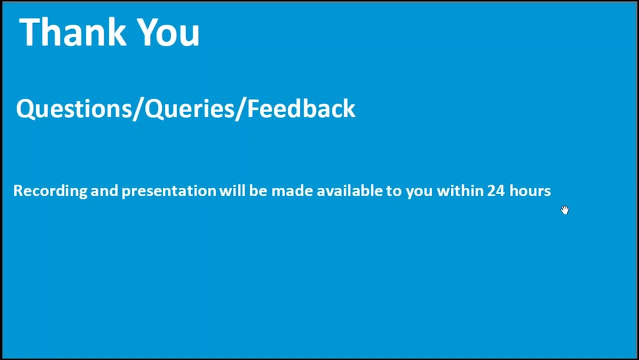 and have it as a overall solution. correct, friends. So it's nothing like you know, one size fits all model. You'll never find that kind of thing going forward. PIG is a data warehousing technology. How will it be useful for data mining? 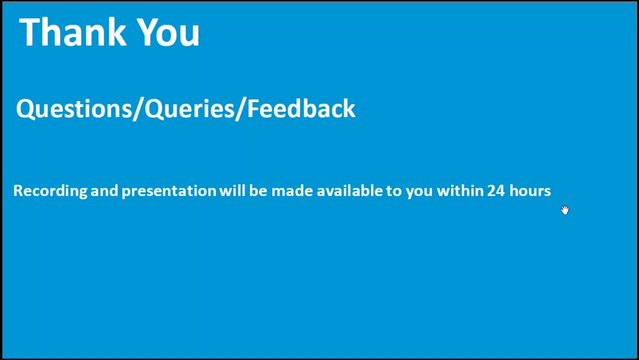 Thaniru, the point is PIG is more a data transformation, It's a ETL tool. Data warehousing is more. Hive is data warehousing part. PIG is more a ETL tool to do the cleansing, you know, especially when you have. 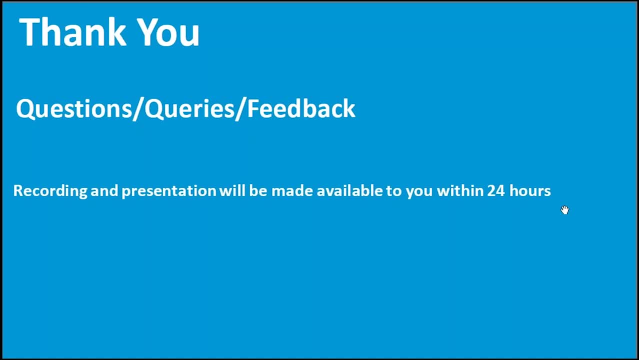 you can use extents, you know the date formats are coming in different ways, and all that You can do a you can use that tool to clean the data right Using regular expression. It provides lots and lots of features. Sure, it's very easy, also very simple to learn, and all that. 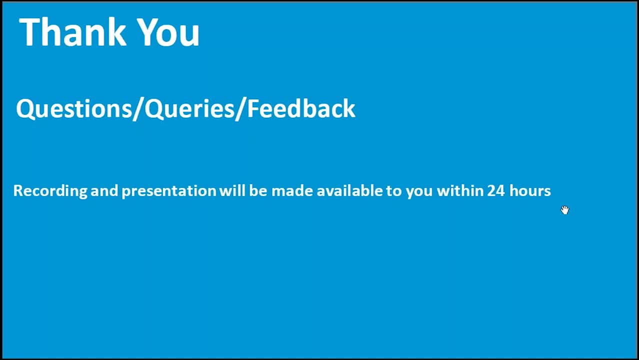 So, friends, I think I hope I was able to answer the questions, because I don't see any more questions here, Hope you all enjoyed the session And hope you found it useful. And I would request, as usual, just provide your feedback. provide your feedback. 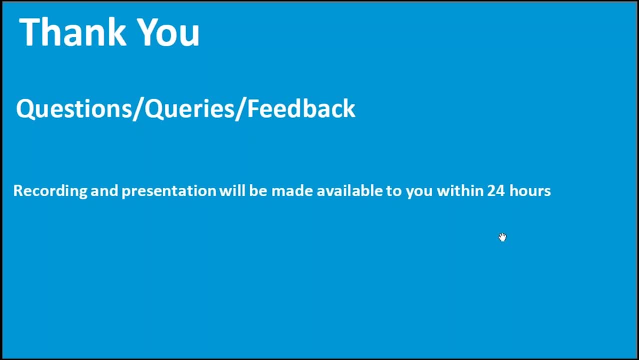 And you know we are here to improve further, right? So thanks for your patient listening. So I look forward for your feedback once you end the session. So please take time and you know provide. you know provide the feedback, friends. 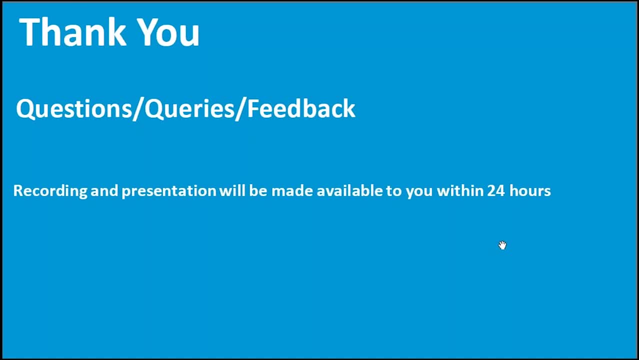 So for anything on the tech, you know the recording or anything on the logistics part, check with the Edureka support and they should be there to support you. And thanks, friends. Thank you so much. I really enjoyed the session with you.